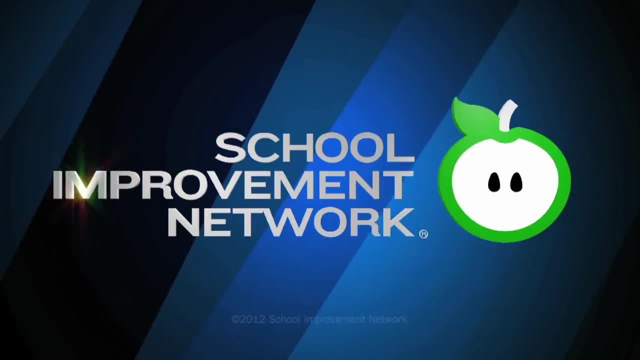 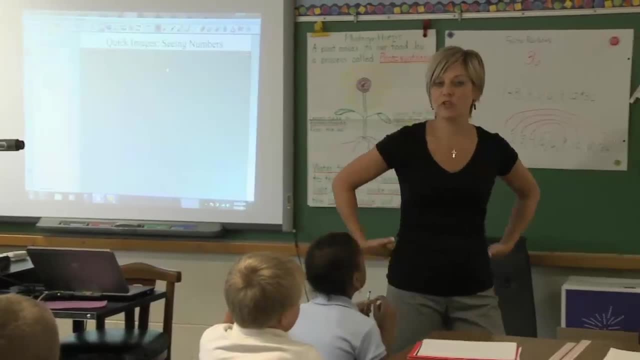 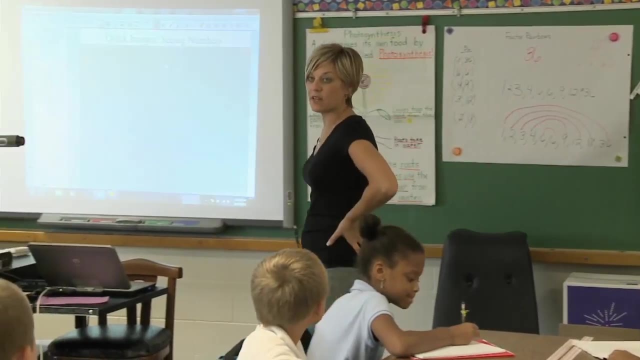 Boys and girls, today's lesson we're going to start off with quick images, so you need to have your math notebooks out. Let's date it for September 14th. We start at quick images just in the beginning of this week, Remember? I'm going to show it once, five or ten seconds. 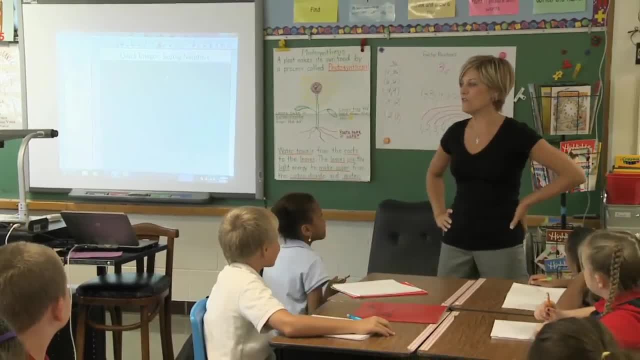 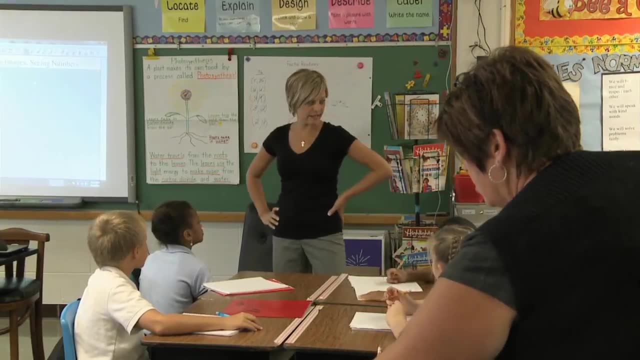 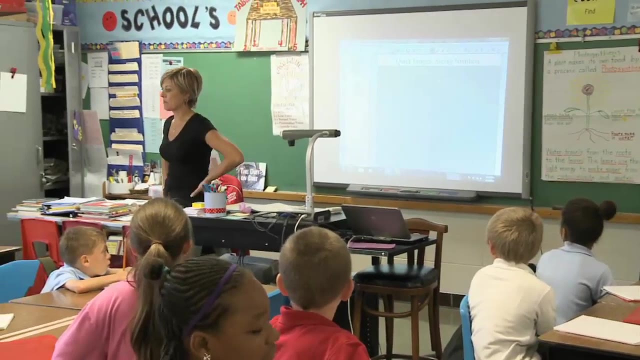 and I'm going to hide it again. So you need to really visualize what you see and draw what you see. I'll give you a few seconds, I'll show it again, I'll hide it again. Again, you're going to add to your visualization of what you see. Then I'll show it a third. 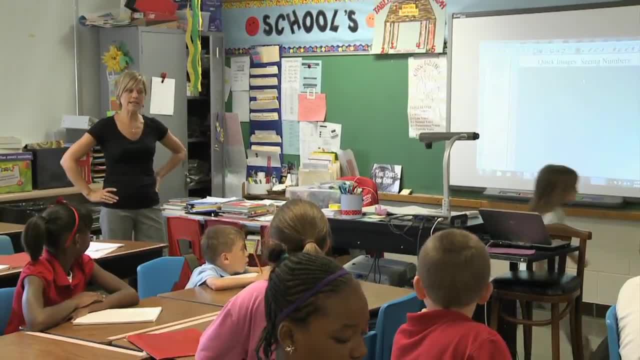 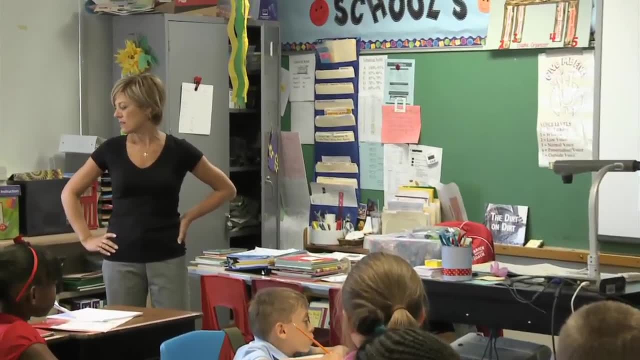 time, and we'll talk about it. We'll talk about how we can get it to relate to math, math equations, And some people think we're going to probably have different ways of viewing it, So we'll talk about that too. So are your eyes ready? Okay, here we go First time. 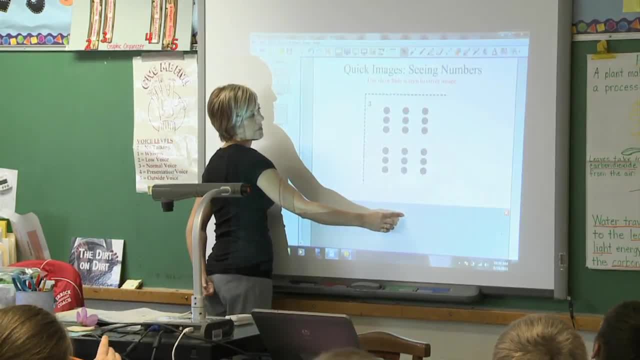 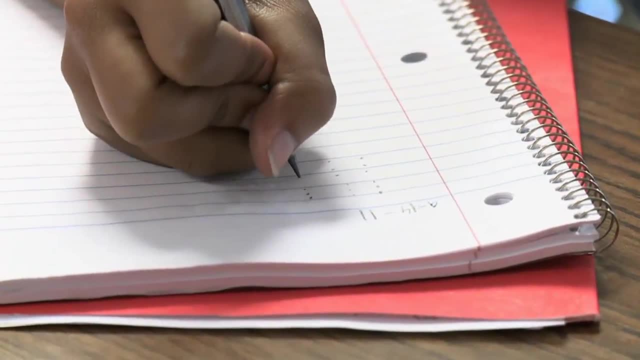 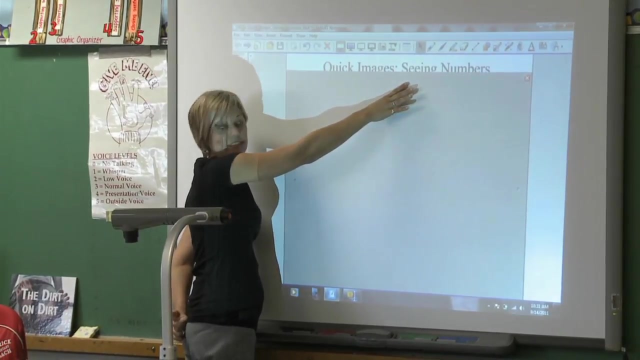 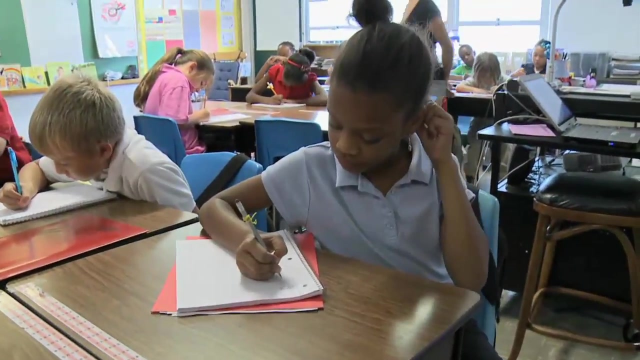 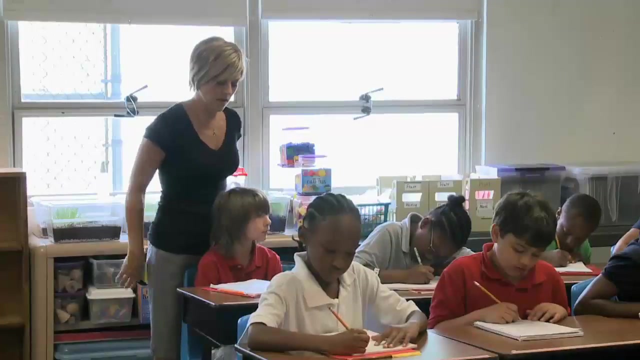 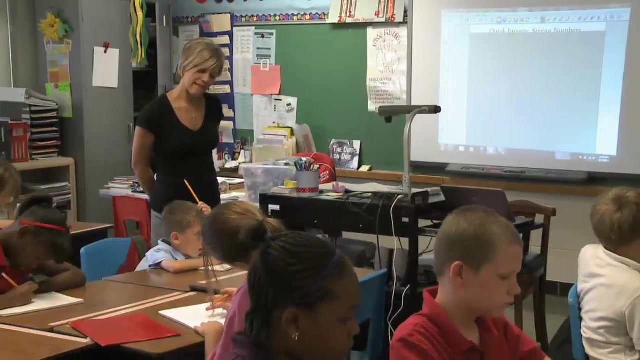 let's look at it again, Your eyes ready. I don't want anybody to miss it. Can you think of an equation that might go with this? How did you know how many There were? Can you circle your three groups of six so I can see it even better? Okay, 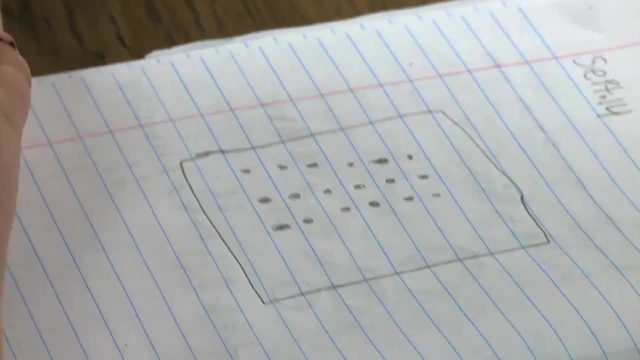 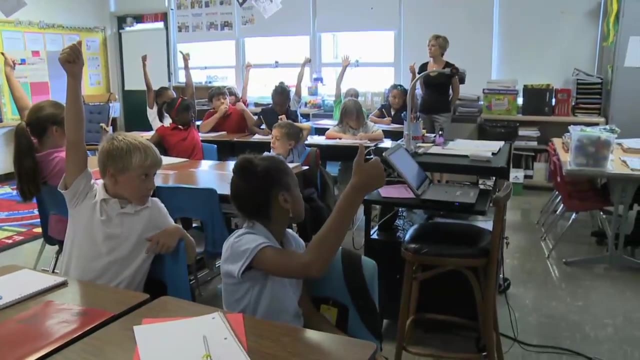 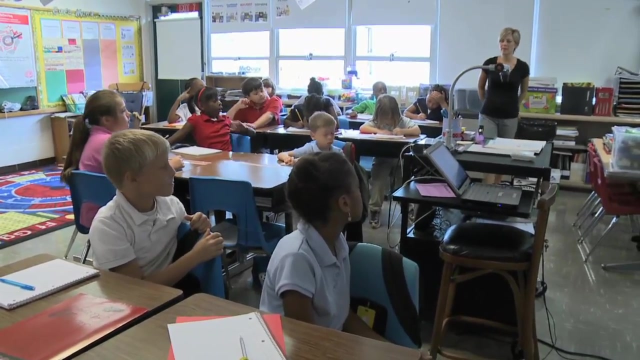 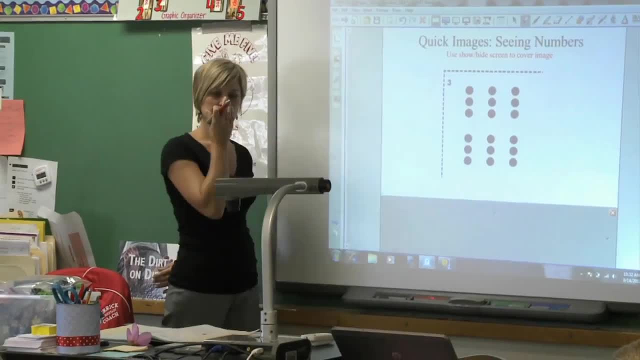 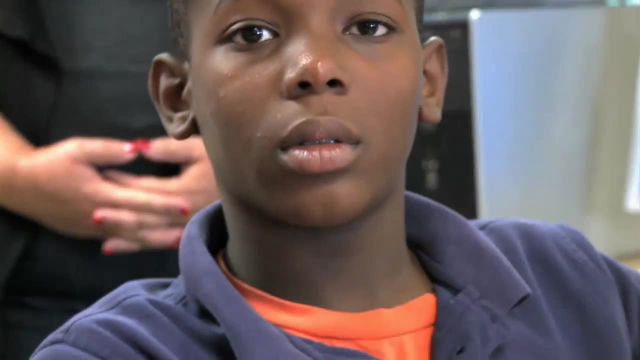 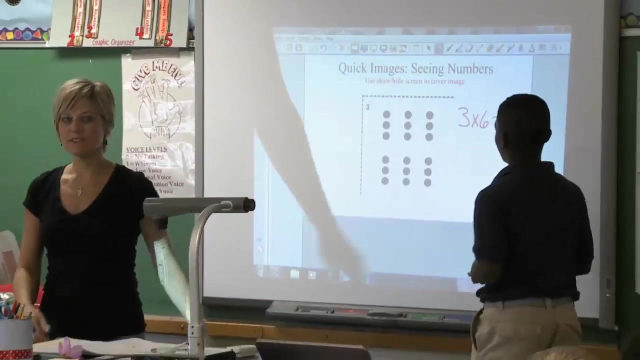 Jose, what you do? I put: three times six equals 18. you got three times six equals 18. you come up here in circle how you visualize three times six equals 18. please thumbs up if that's what you saw. ah, so we've got some thinkers that are 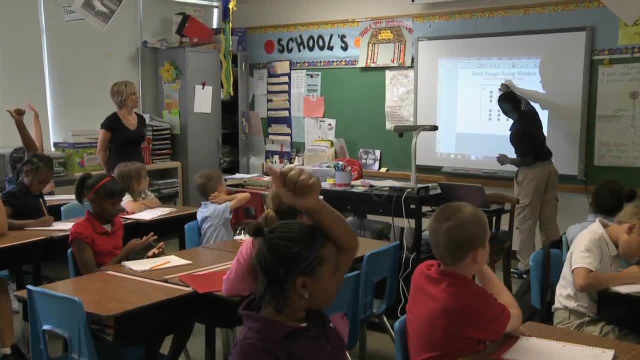 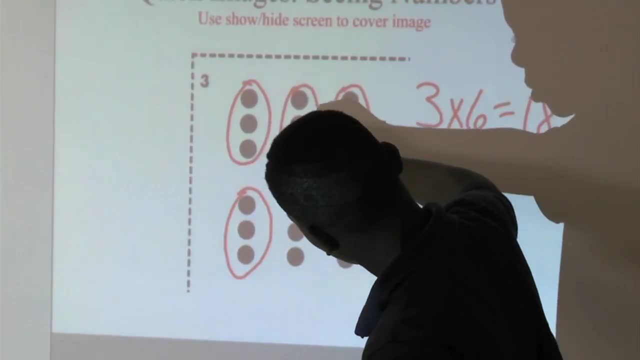 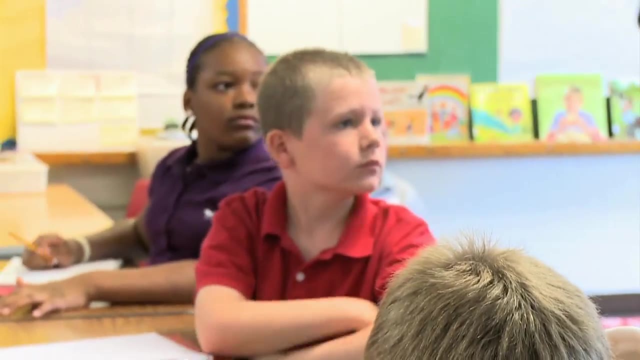 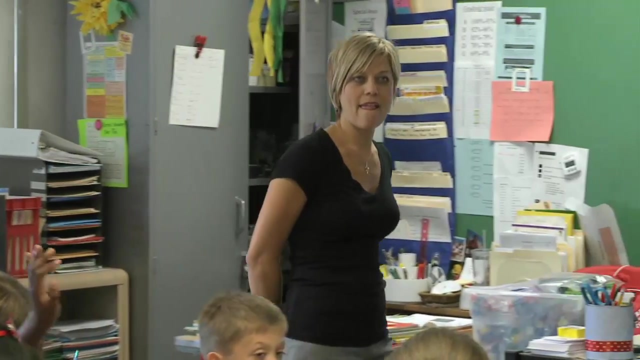 all thinking the same. now he's showing us what's he's showing us. what's he's showing us. Ethan, say it again please: groups of three, groups of three, and how many groups of three did he get? six, six, good job, thanks. anybody see it another way. anybody see it another way? what you? how do you see it? 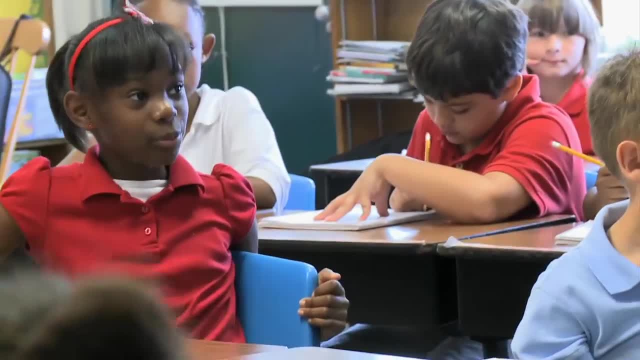 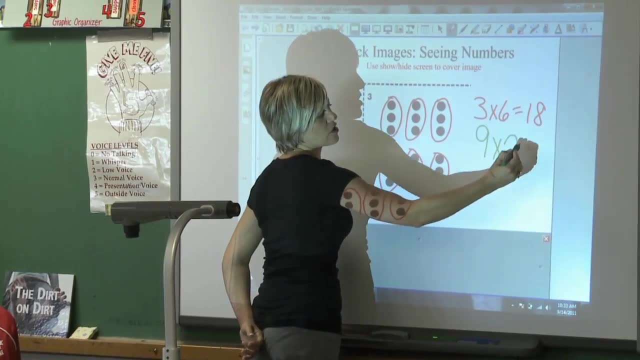 uh, t'andra. two, nine times two, nine times two. and what did you get for nine times two, 18? nine times two equals 18. can you come up and show it, please, using a different color marker, so you could see it? did anybody think like t'andra? 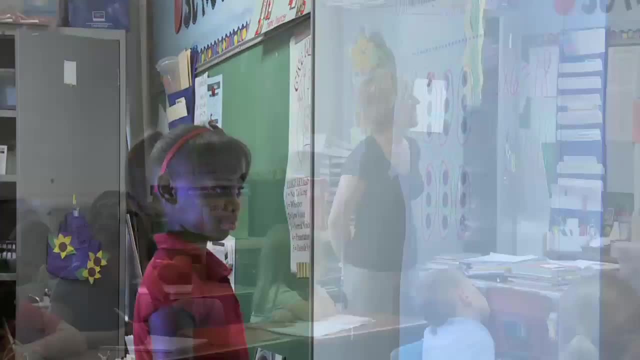 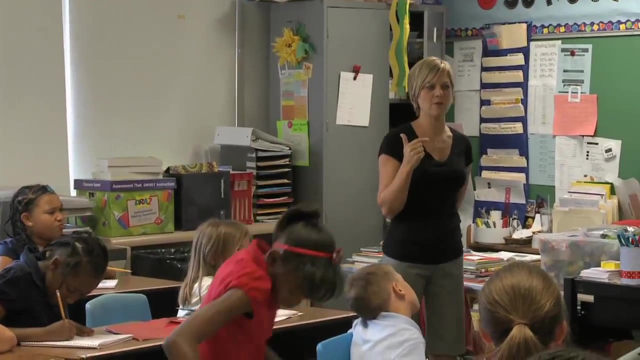 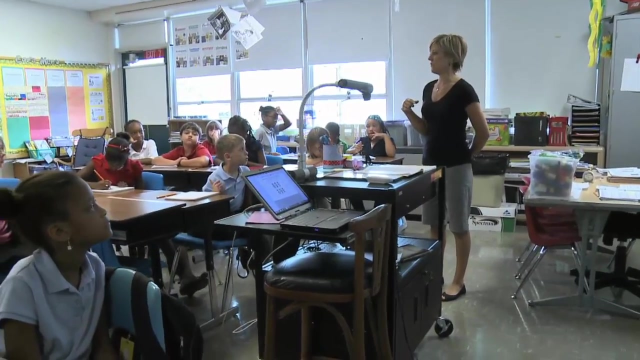 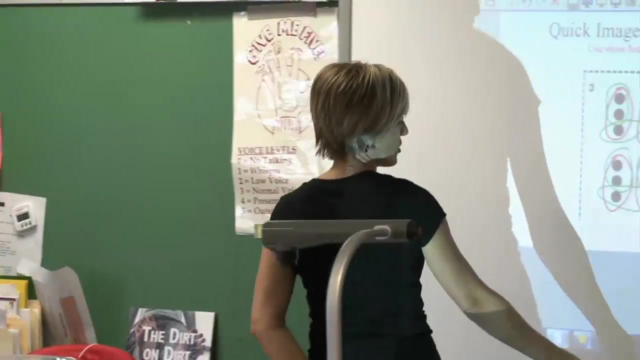 oh, okay, I see how you connected it: nine groups of two. did anybody do the commutative property of that one? because I really didn't think nine groups of two. I thought of it as what's the commutative of 9 times 2, two times 9, and I'll show you what I do. did he might think of it like that: two times nine, two groups of 9?? 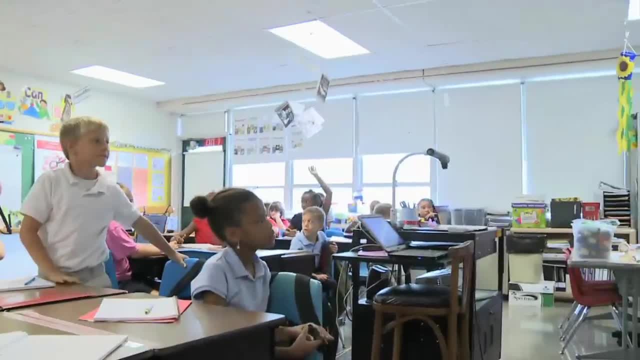 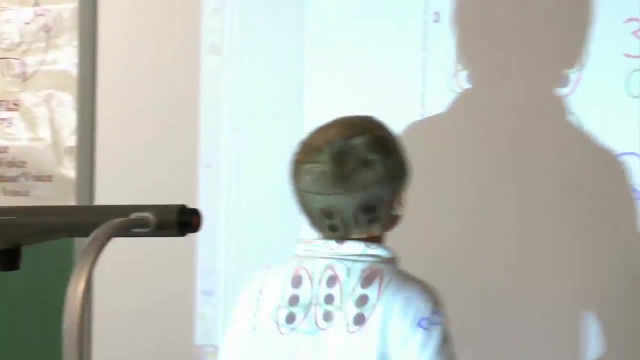 Come up, Jacob, and show us how you saw it. that way, We know that these mean the same thing. We've already talked about that, But circling them might show it in a different way. Show me your two groups of nine. 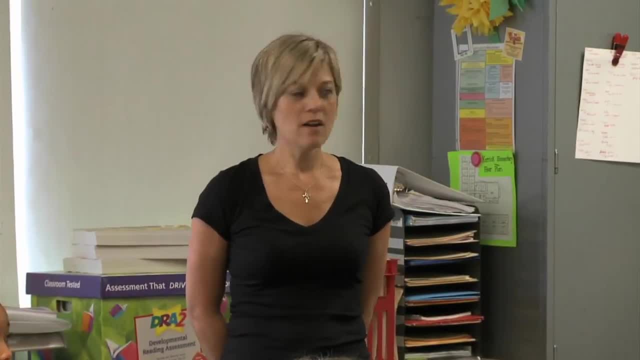 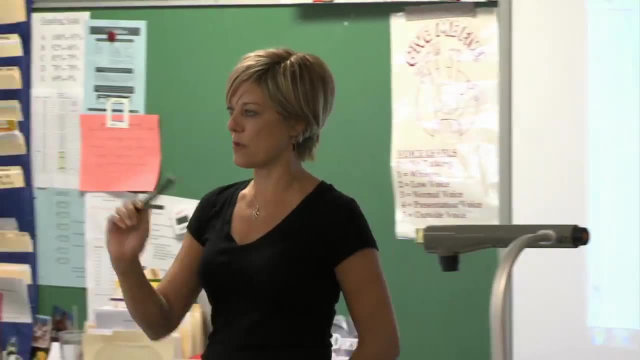 Good job, Good job. Another way. We've got another marker. We can do it one more way, and then we're going to go on with our math lesson for the day. Another way, What did you get? Kiera's going to show us what she's doing. 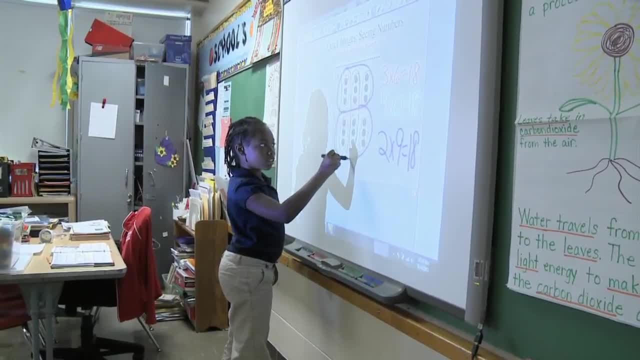 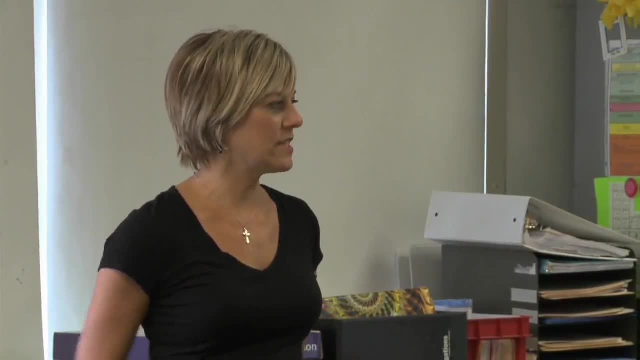 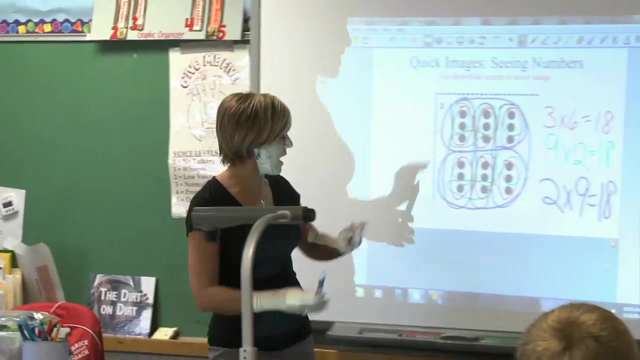 Oh, okay, Good, So you and Jose were doing the commutative of each other. The first Flip-flops is what kindergartners call them right, But not in fourth grade, So a lot of us saw it as looking at groups of. 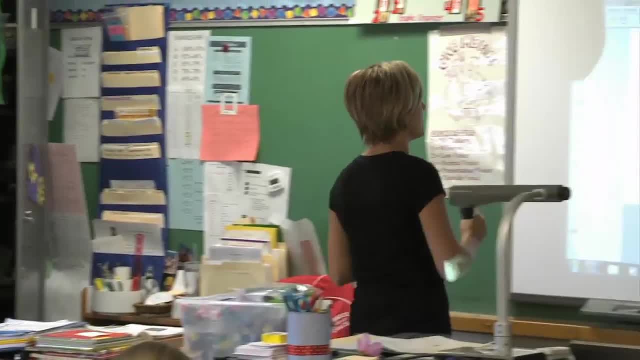 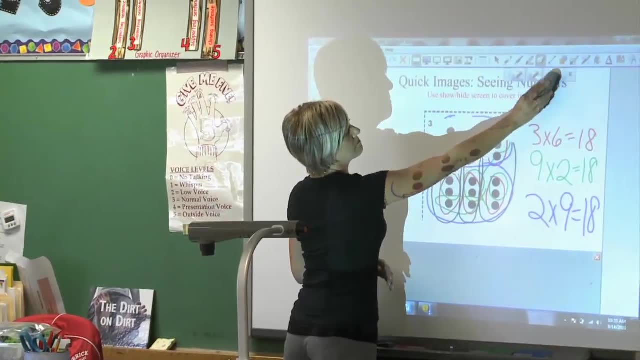 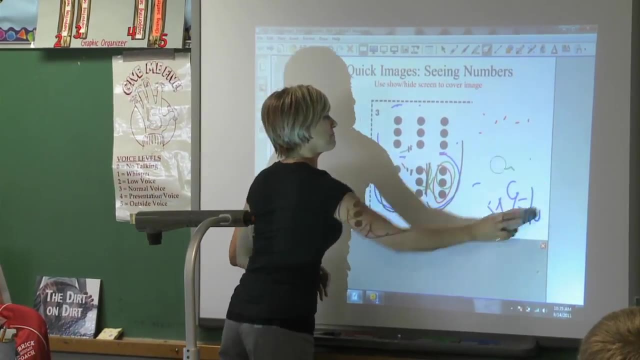 As groups of. If I was going to put- and this is just going to extend it a little bit- If I was going to put all of these together, Well, Grab the little eraser out. It's not. Does that look big? 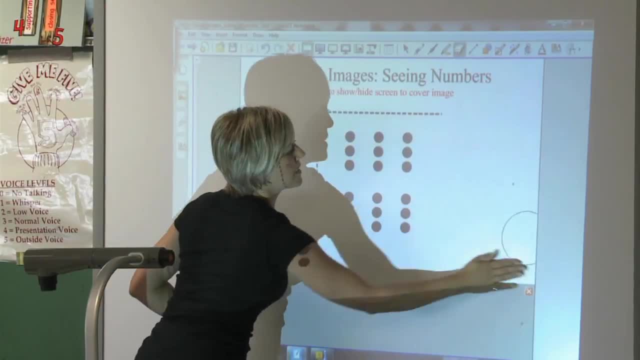 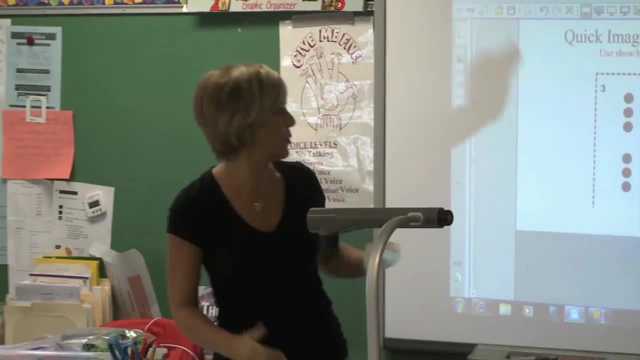 Uh-huh, Oh, that's big, That's big, It's like quicker. If I was going to put all of these together and make What am I making if I put all of my rows and columns and I fit them together? 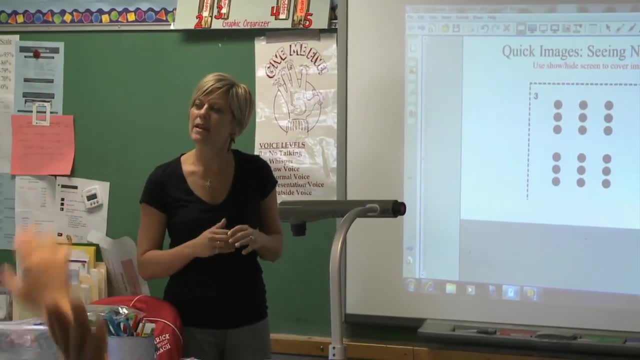 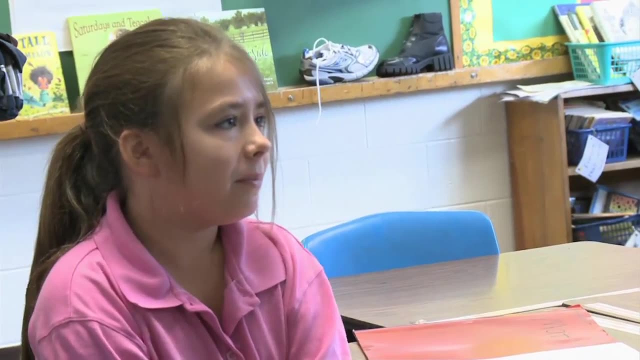 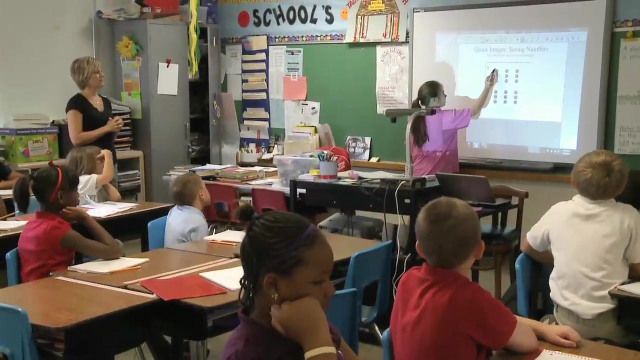 What am I making Trent, An array. What am I making? An array? An array. What would the dimensions be if I was going to slide them all together, Six by three? Good job, Come and show us, And then label where your six would go. 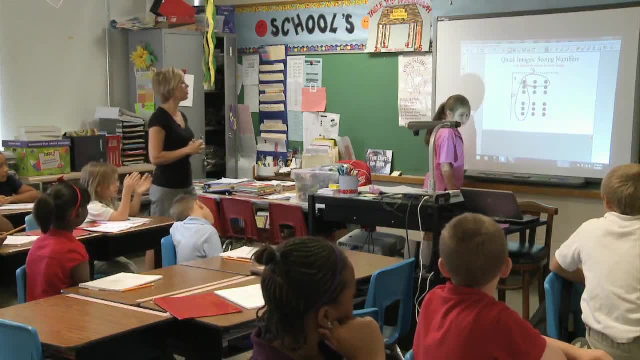 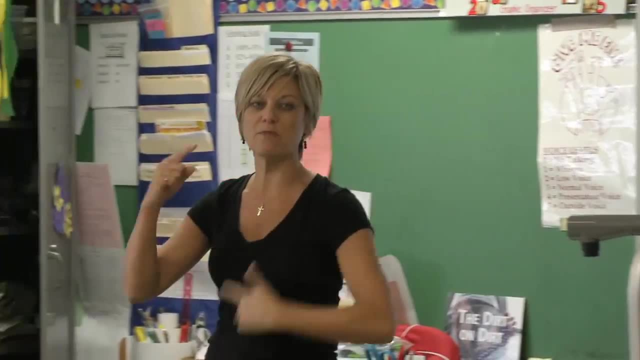 Good job. Cool, Cool beans- That's the new word, Cool beans. Good job. Good job on quick images. We're going to do those. Why are we doing them? We're going to keep doing them. Why? What's it going to help us do? 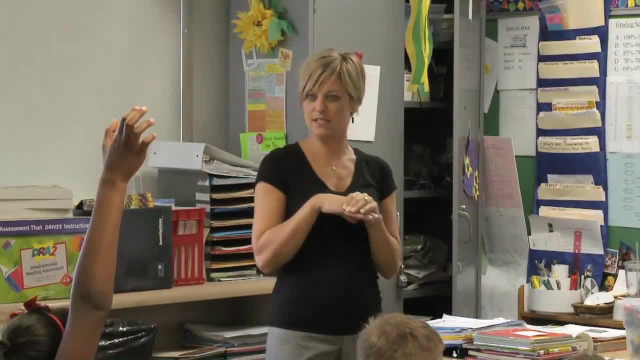 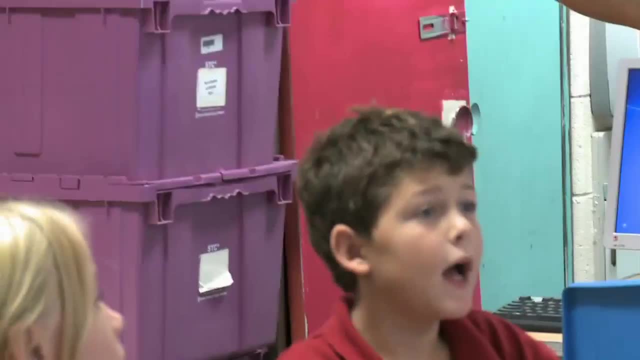 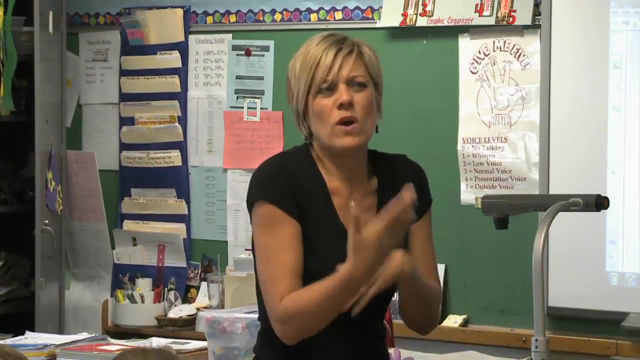 Especially us that still are trying to memorize some things. What's it going to help us do, Matthew? Sometimes it can help us count better, count faster, And what's counting have to do with arrays? It can help you learn times. 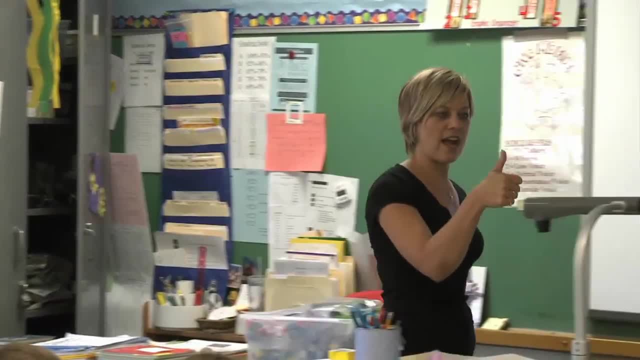 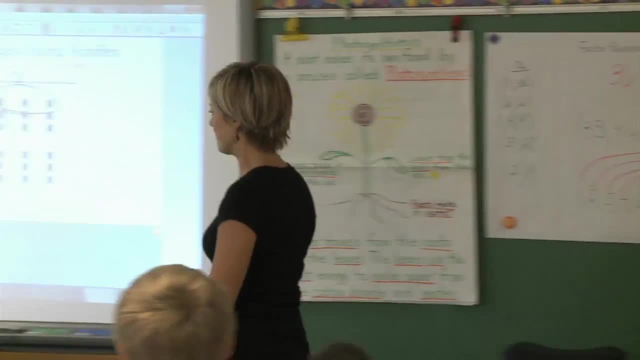 Exactly, Very good. Exactly All right. You can keep your notebooks open because you're probably going to need them, But I need your pencils down And all eyes Up here. Up here on our smart board, We're going to do a think-pair-share. 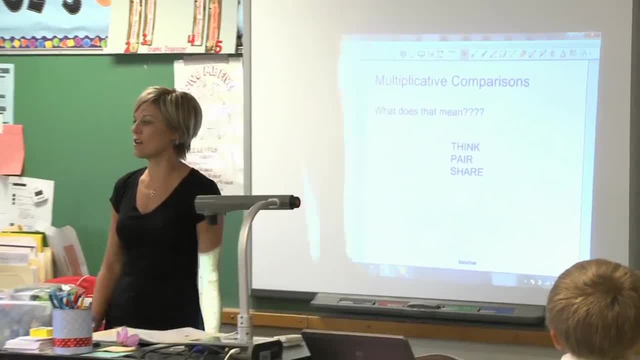 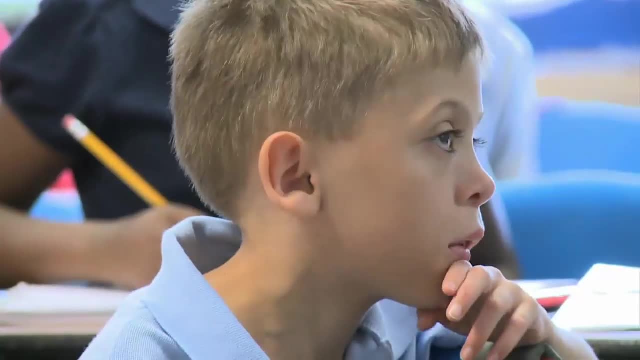 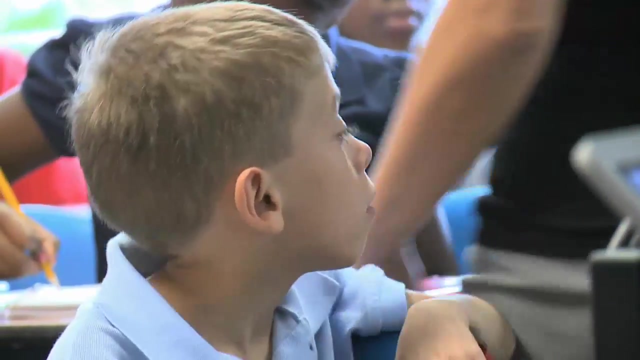 We're going to do a lesson today. It's called multiplicative comparisons. I want you to think: what does that mean? And I'm even going to give you a little bit of a hint. You all know, back here on our cafe menu, how to figure out what words are. 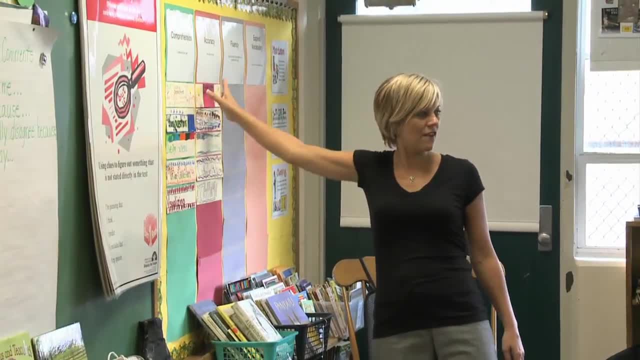 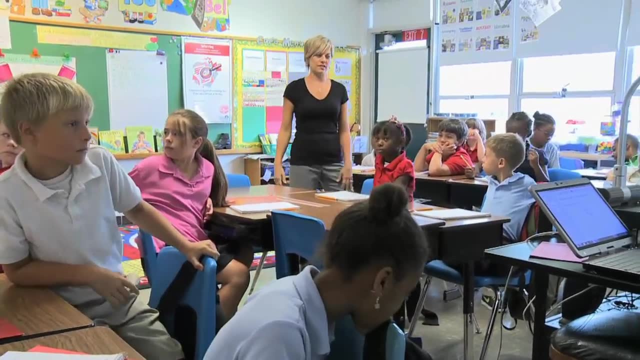 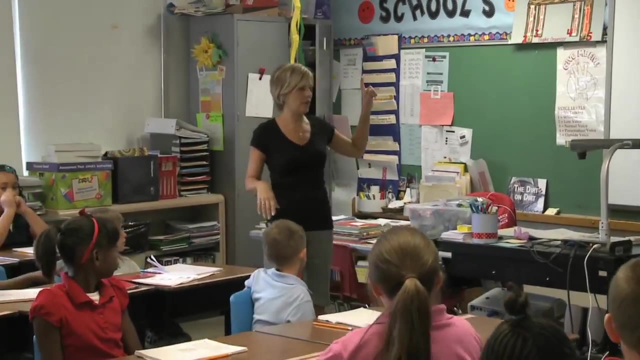 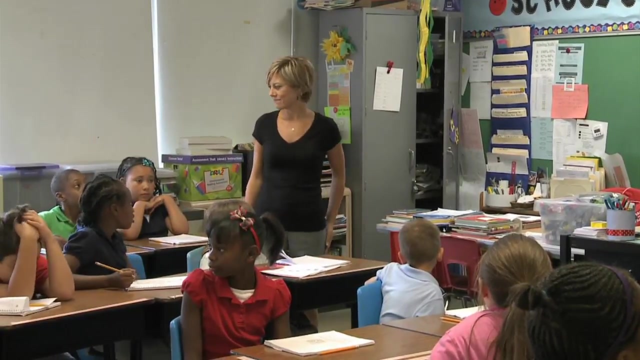 You've given me these ideas how to figure out what they mean. We've done Nifty, Thrifty, Fifty. talked about prefixes and root and base words and suffixes. Use your schema in reading to help you figure out those math words. Think: What does multiplicative comparisons mean? 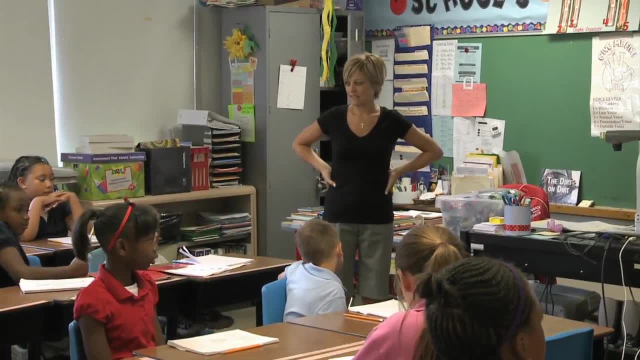 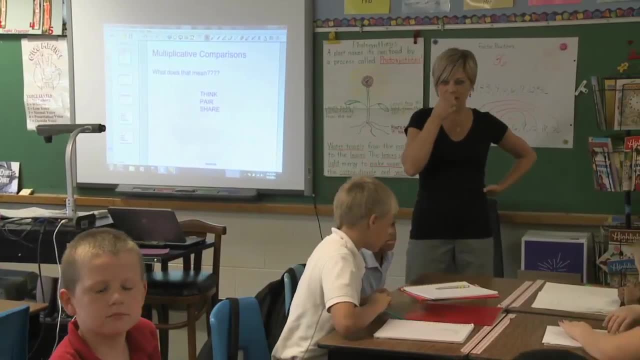 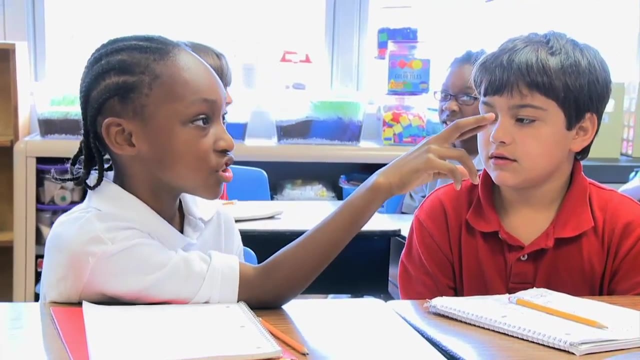 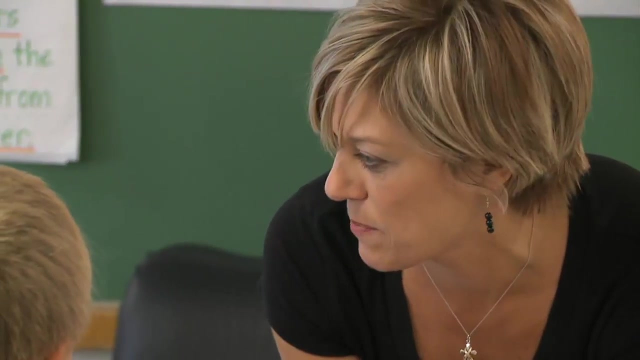 You're thinking, Pair up with your partners sitting around you Talk about it. What do you think it means? Multiplication, and uh, talk about multiplication and then compare, compare. We compare the multiplications together, Multiple, multiply. What about comparison? 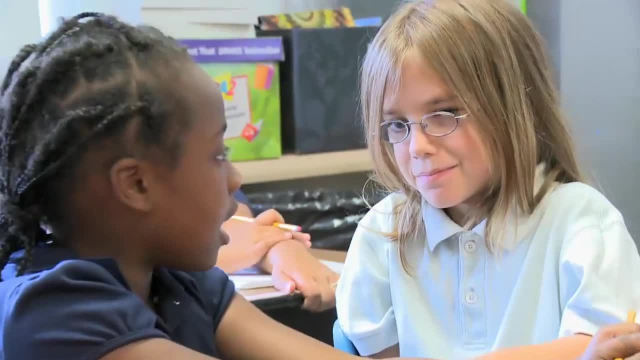 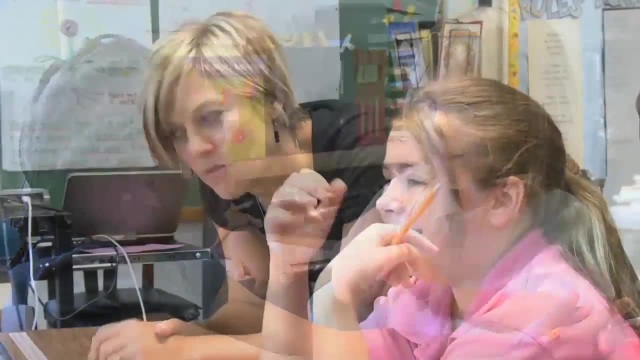 Comparison. What's the word in there? Comparison, Like it's the same. Now, what do you think it is? I'm thinking kind of the same thing. What did you say that she agreed with? I said um multiplication, com comparison. 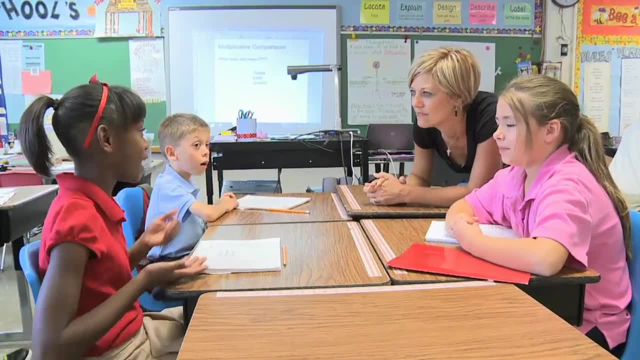 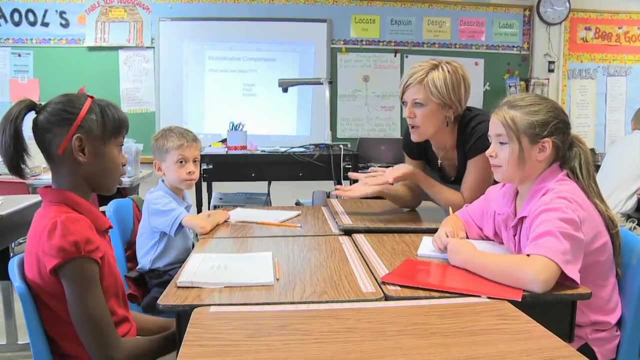 I know it's hard. It's where, like you both, get them like steady for each, for each one, if they're like flip-flop or not Steady. So what's steady mean when you're talking about multiplicative comparison? 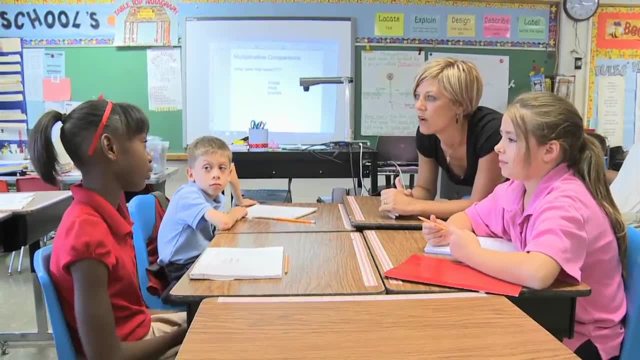 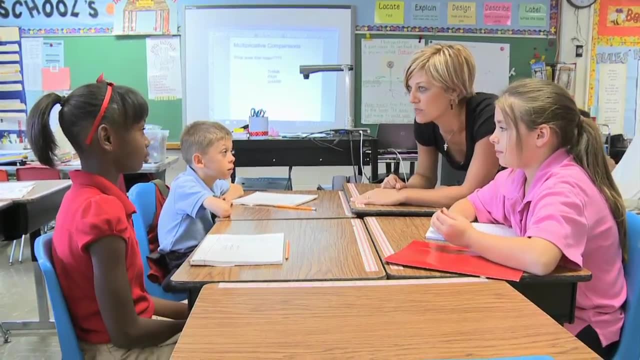 Um, seven times three and three times seven. Okay, So you think it kind of means flip-flops, the, and you said that the commutative property. Okay, I love the way you always try to give examples to help me understand. 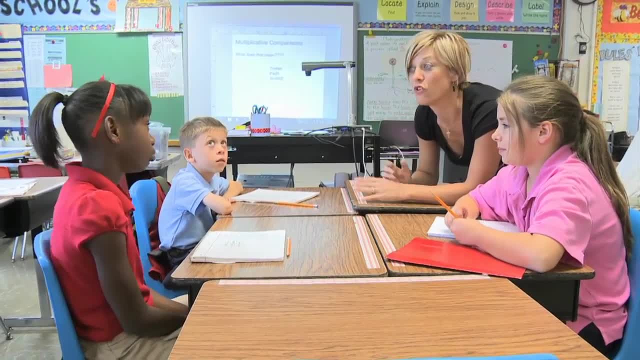 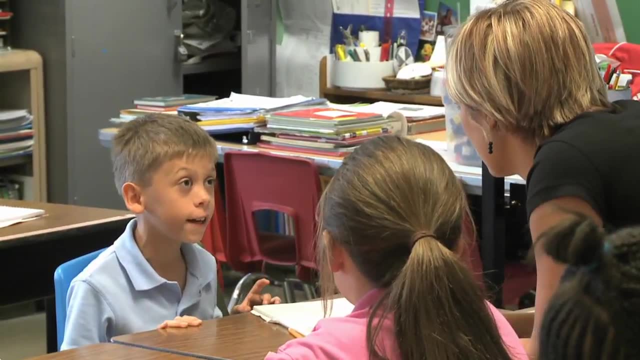 That helps me, And like you can still get to compare them. Yeah, And you're comparing those two. Okay, What do you think? Well, I think it. it could probably like, mean, like it could be a different array. 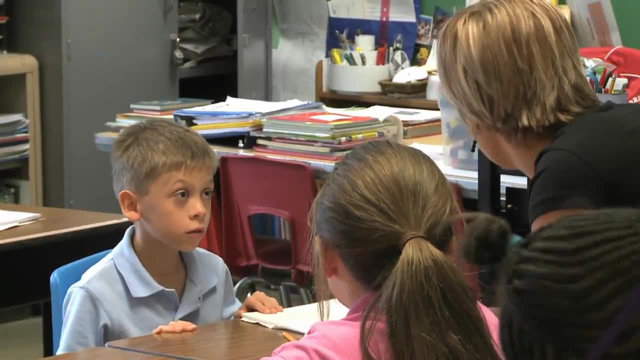 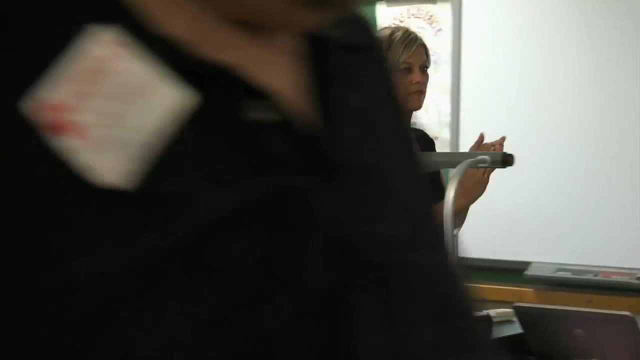 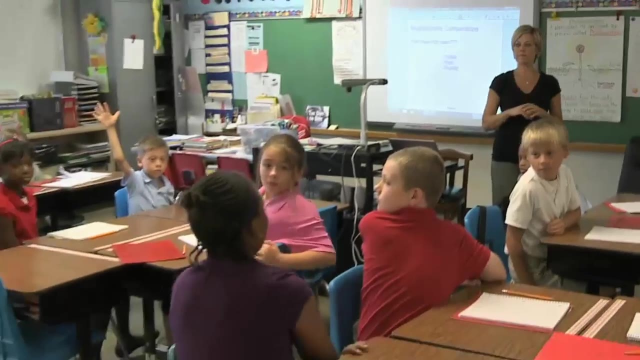 A different array, So you're going to compare one array to a totally different array. Yes, ma'am, Okay. Does anybody want to share their thoughts, their ideas? Mm-hmm, Kiana, Me and my partner said that multiplication is a common thing. 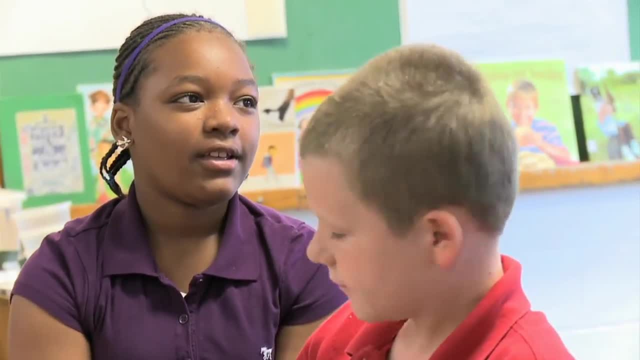 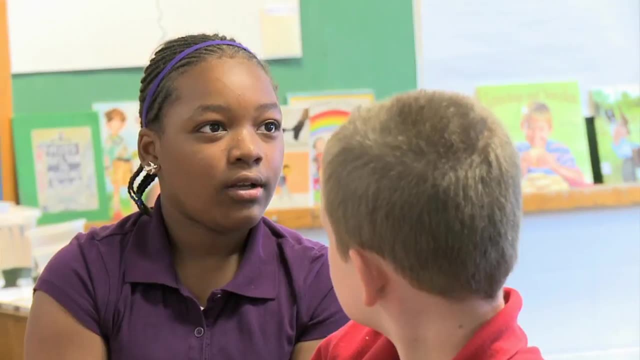 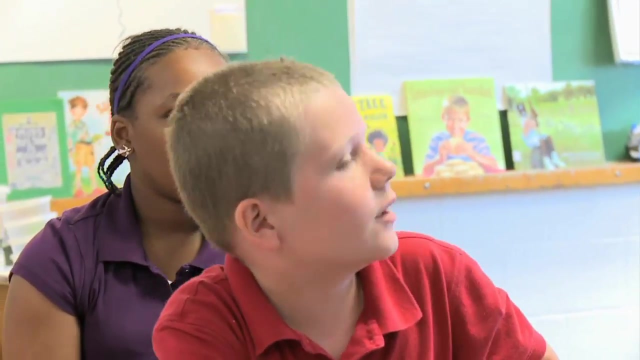 Compare multiplicative comparison. Multiplicative comparison means- we think it means- that you compare one one. What does she say? Multiplicate? Yeah, Ethan, you can help her out if she wants your help. We believe that um. 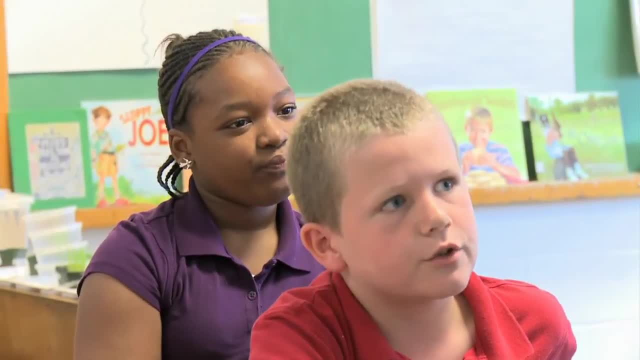 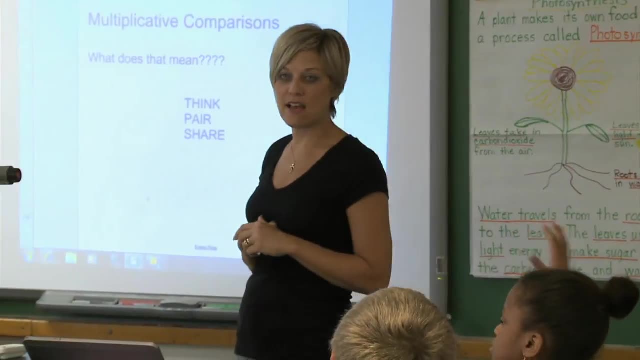 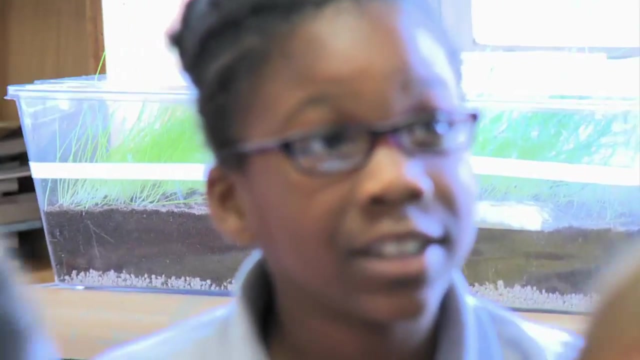 That means that we, that you compare one multiplication equation with another, Okay, Okay, That's a good idea, Good thinking, What do you think? Uh, I think that we, we have to put two numbers together and see what it equals. 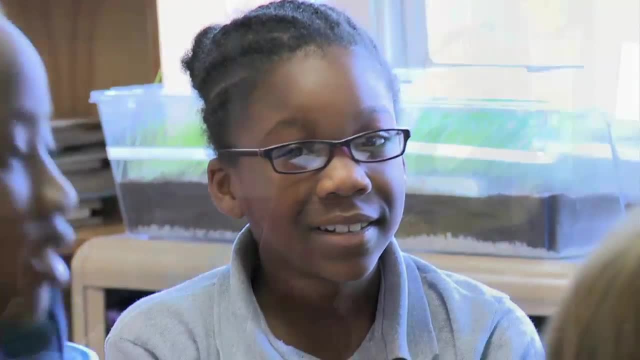 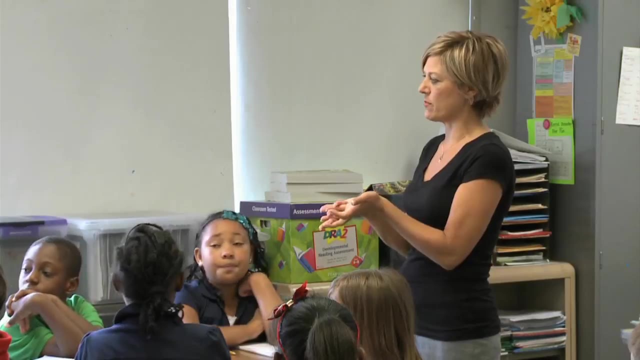 Any two numbers? No, Um. And you said: see what it equals. Well, let me rephrase my question: What are you going to do with those two numbers when you put them together? You got to tell me what put together means. 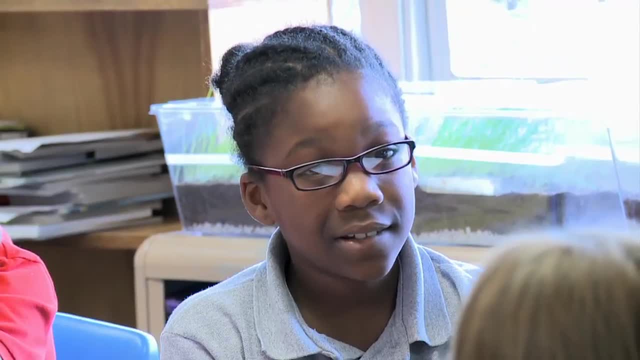 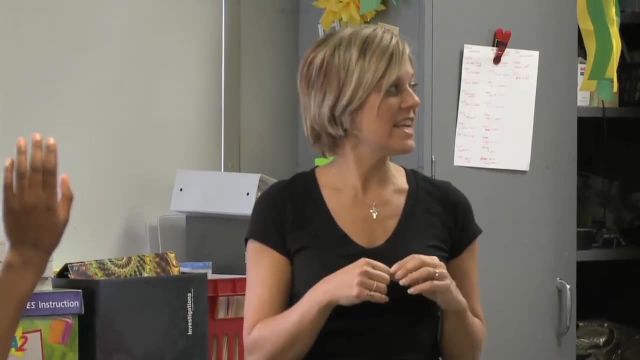 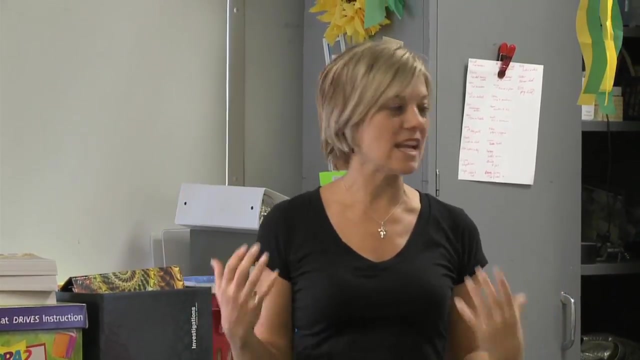 Because we can do a lot to numbers. Think of your word. Yeah, Think of the word. Think of your word. Do you see any words, small words, that jump out at you in that big, long word? multiplicative comparison. 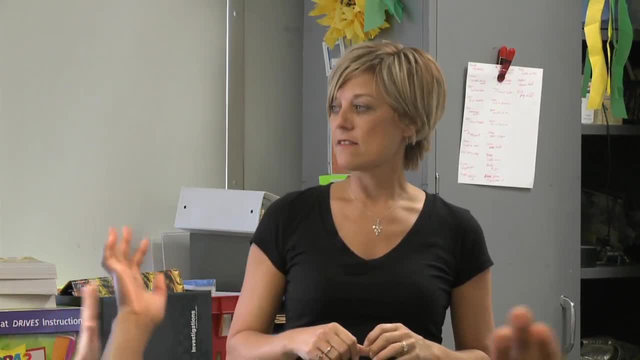 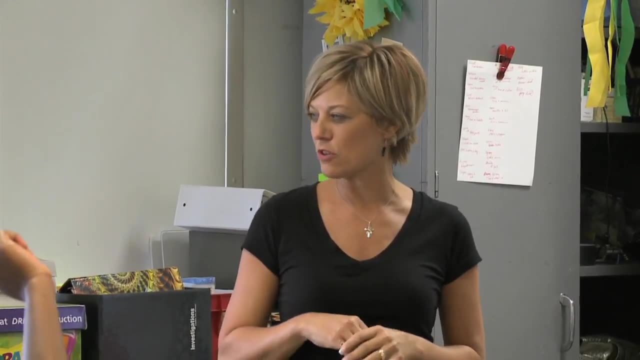 Yes, Compare, Okay, But I you were talking about doing something to two numbers. Do you see another word up there that might help you decide what you're going to do to those two numbers? besides compare them, Share, Share them. What are you thinking, Trent? 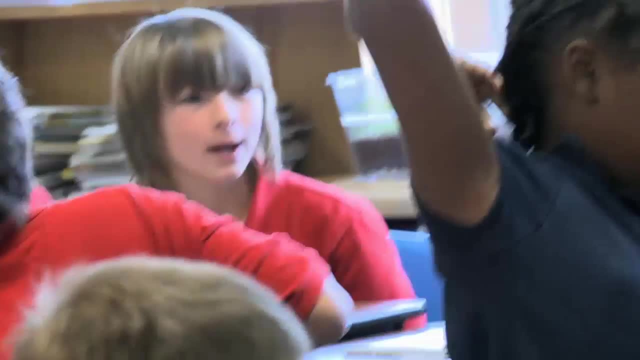 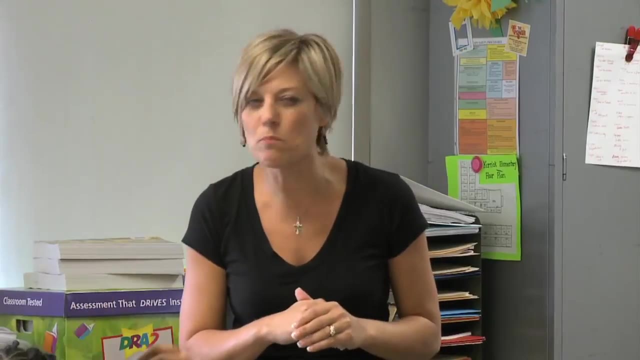 You have your hand in the back. I was thinking that it might. you might have to have two numbers and you have to find the multiples. Okay, And why do you say two numbers with multiples? Why, why do you use the word multiples? 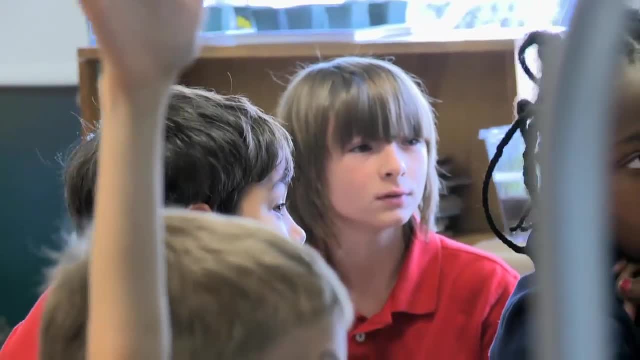 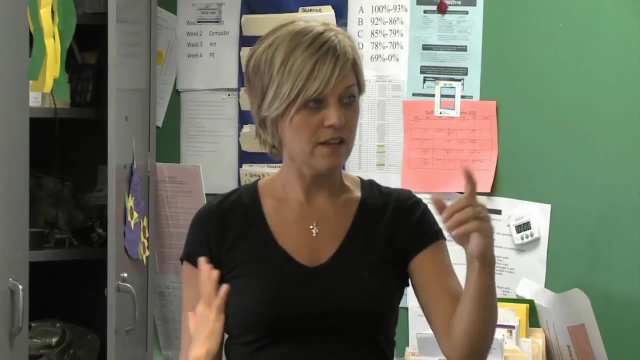 Because it says multiple. So you're, you're chunking, You're seeing a little word in that big long word. That's one of the things that we said about accuracy. That's one of the things we're learning about Nifty, Thrifty, Fifty. 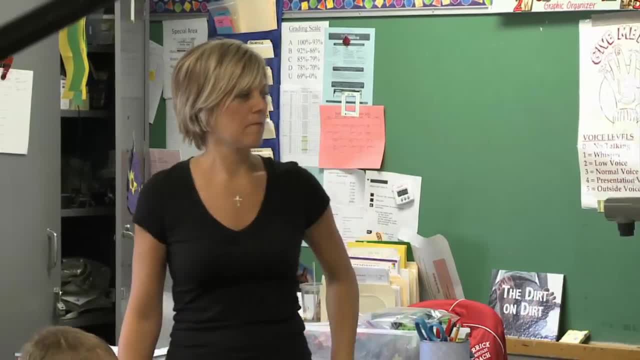 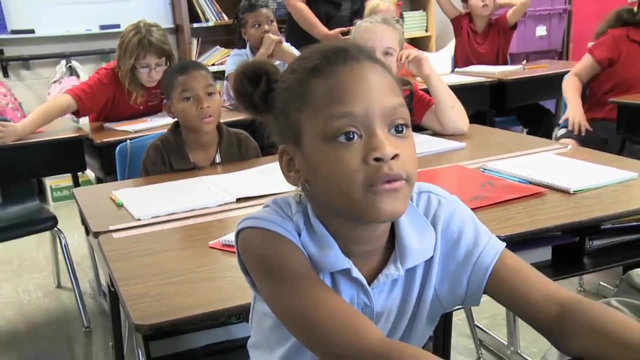 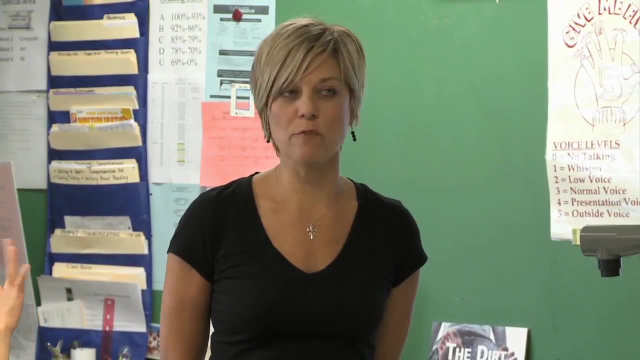 Um Dejanay, Me and my partner thought: um, you take two different multiple multiplication equations and see if they equal the same. Okay, And I'll have time for one more. and then we're going to go on and we're going to see if what. 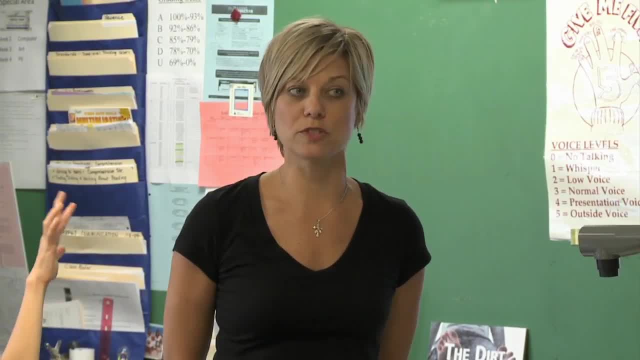 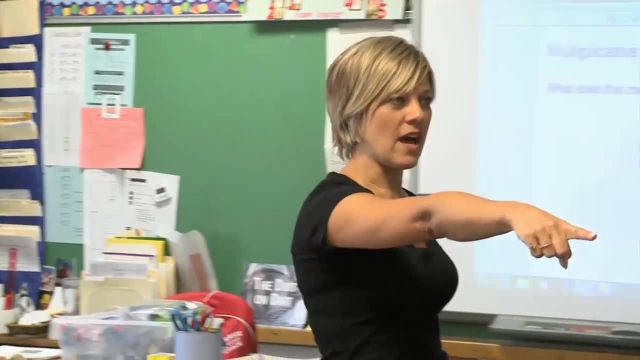 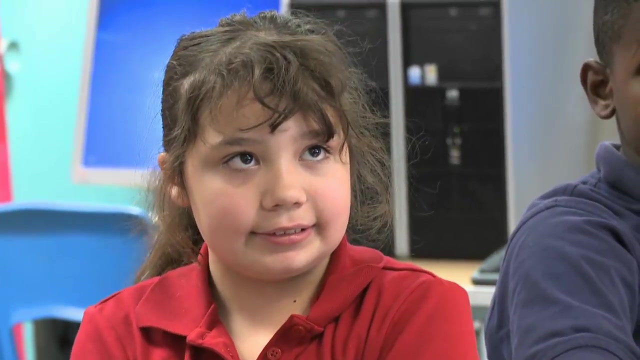 we were thinking is really what we're going to do? What we're going to be doing with multiplicative comparisons? One more: Um, how about Olivia? Uh, sure, Multiplying means multiplying by numbers. So you think multiplicative means multiplying numbers? 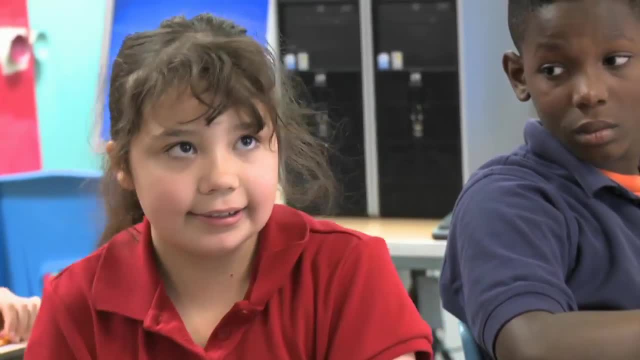 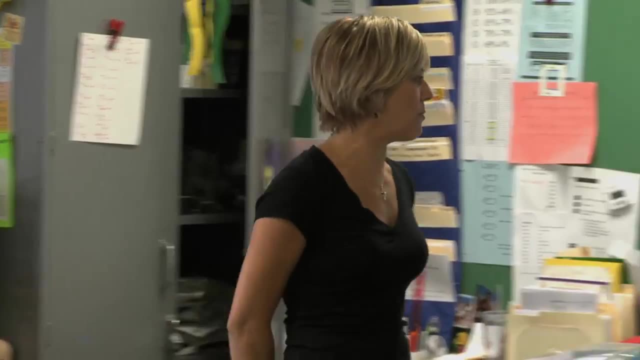 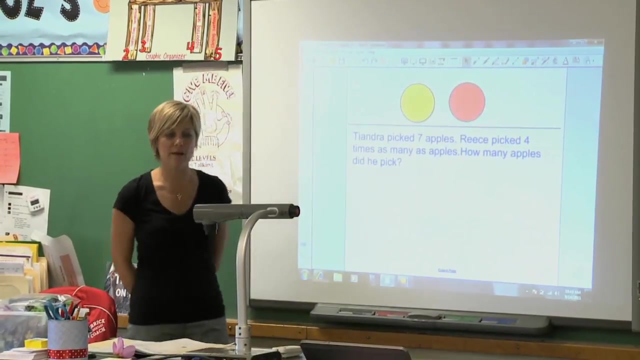 Mm-hmm. Okay, We're going to compare them, Sure, Sure. Okay, We'll try. All right, Let's focus back. We've done our think, pair share, And I want to show you a problem. that is an example of multiplicative comparison. 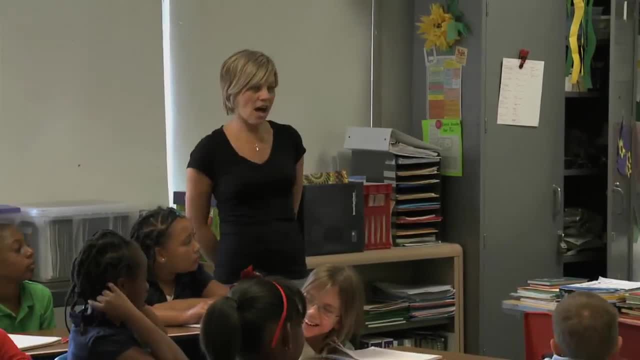 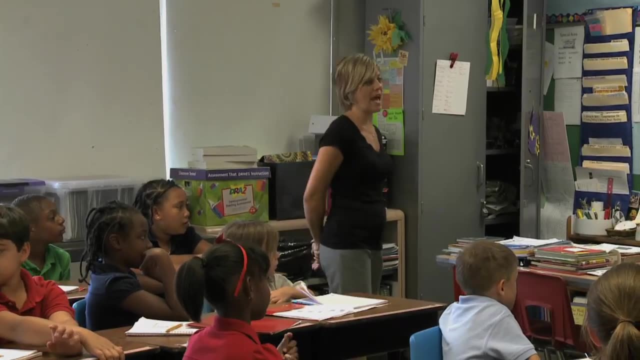 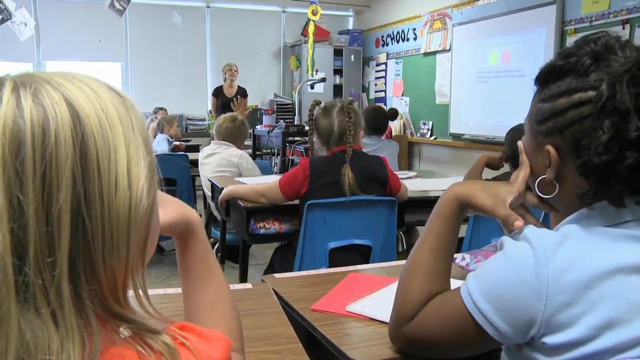 And it sounds like this. Tiandra picked seven apples. Reese picked four times as many apples. How many apples did he pick? Before I even start to think about it like math, I think about it like reading. Who are the characters in our story? 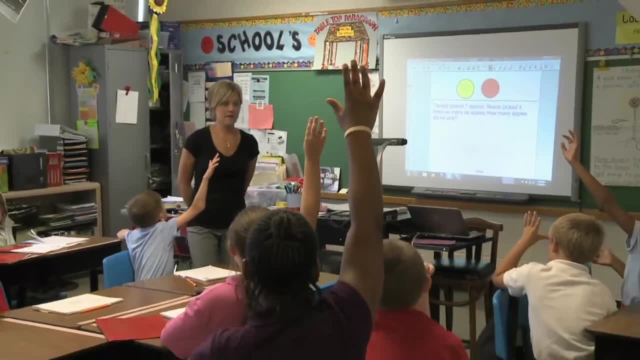 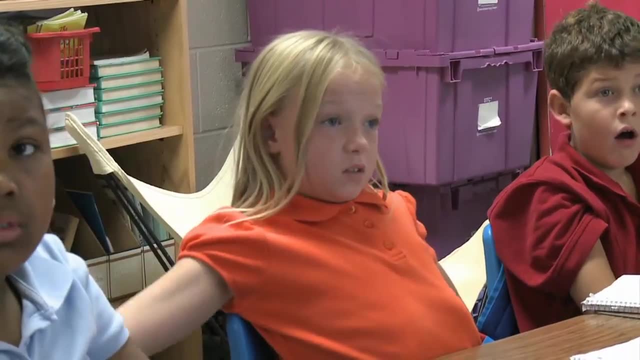 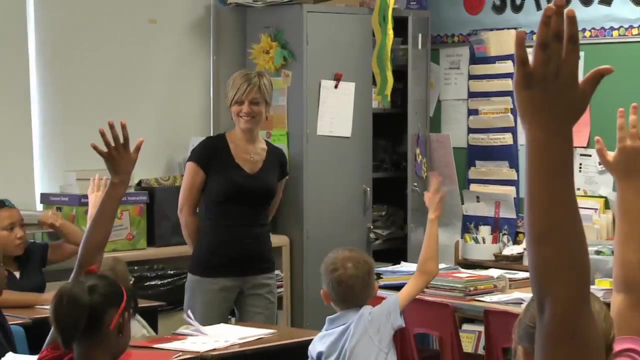 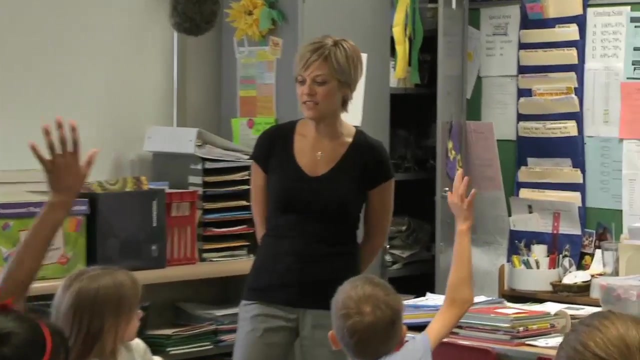 Who are the characters in our story? Kaylee, Tiandra and Reese? Tiandra and Reese: What are Tiandra and Reese doing? Shayla, They're counting apples. Uh-huh, They're counting apples. Do you think they might eat them? 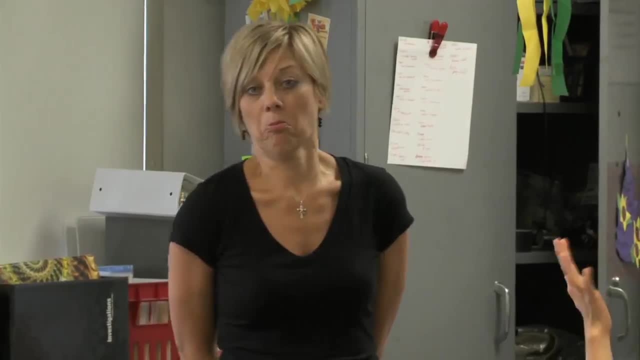 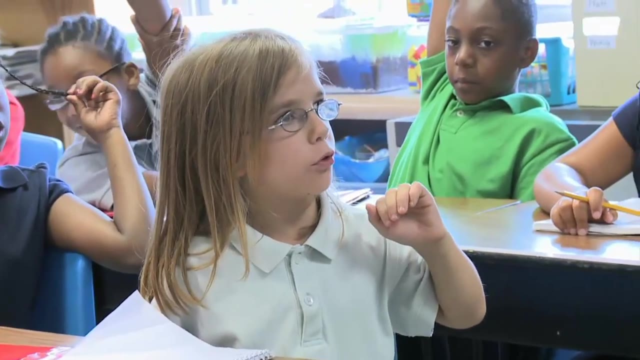 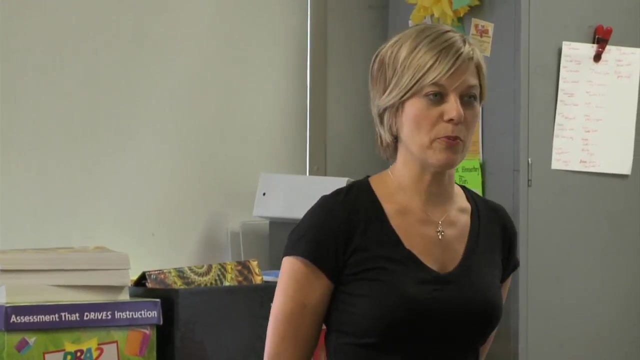 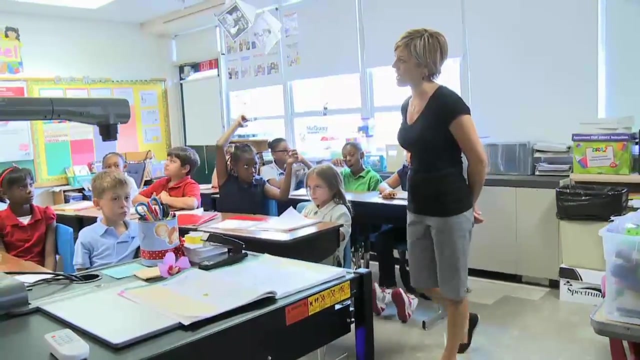 What can you infer they might do with them, besides eat them? Oh, okay, Might plant the seeds out of them and make other apples Cool. All right, What is your problem? Because in math, the story problem becomes your problem. So what do we need to figure out here? 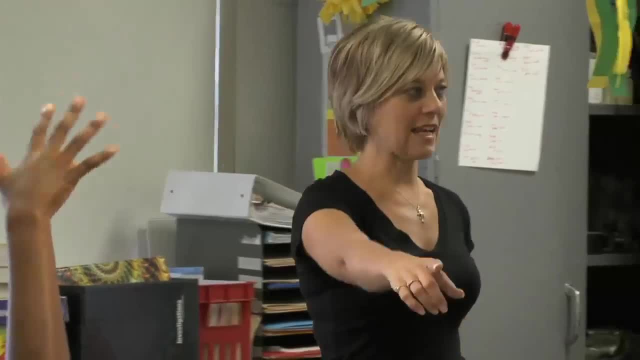 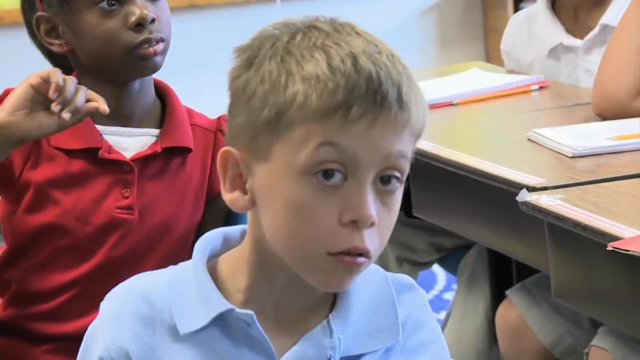 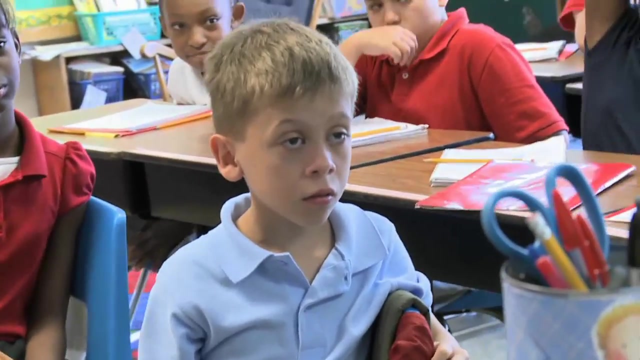 Alex How many apples they have. Do we need to figure out how many apples they have? Do you need me to reread it for you? Okay, It says: Tiandra picked seven apples, Reese picked four times as many as apples. 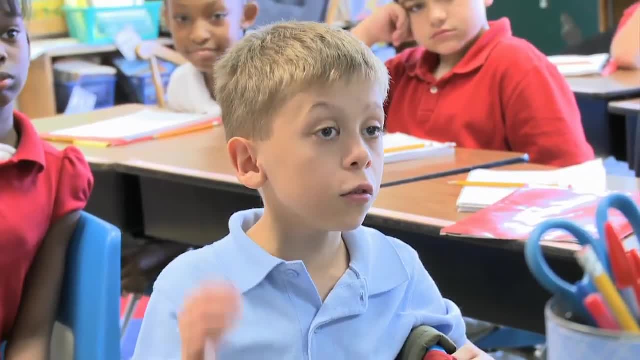 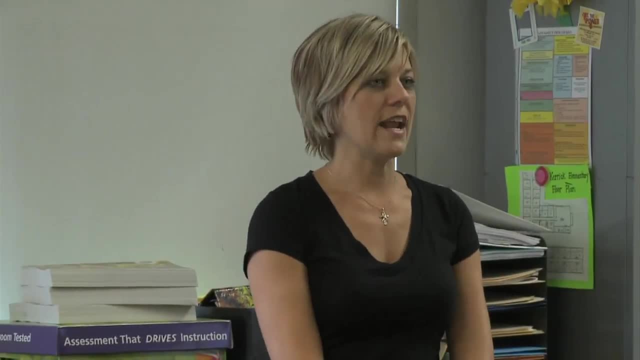 How many apples did he pick? So who are we looking to see? We're looking for Reese. We're looking for Reese's apples. Good job, Good, good, good, good job. All right, Hands down. I'm starting to learn how to use this smart board. 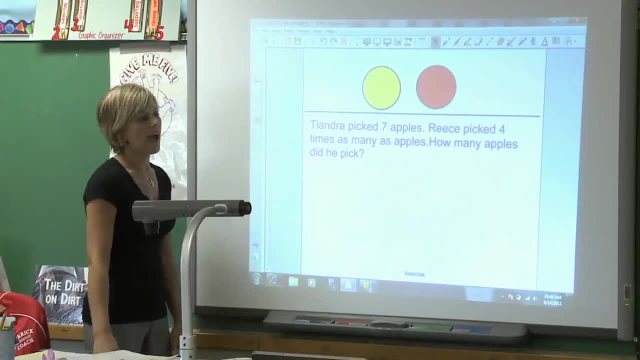 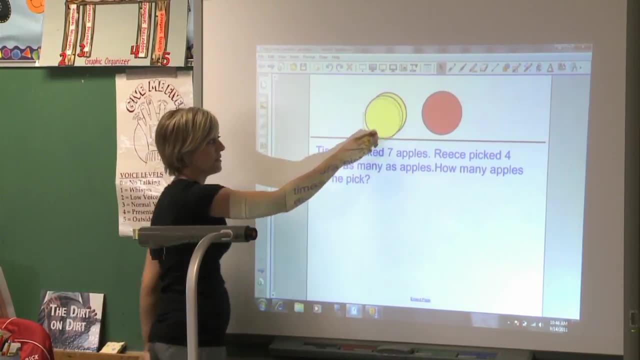 Y'all are going to think this is pretty cool. Your third grade teacher may have already showed it to you. I am going to show you the apples that Tiandra picked. Okay, You can count with me One, Two, Three, Four. 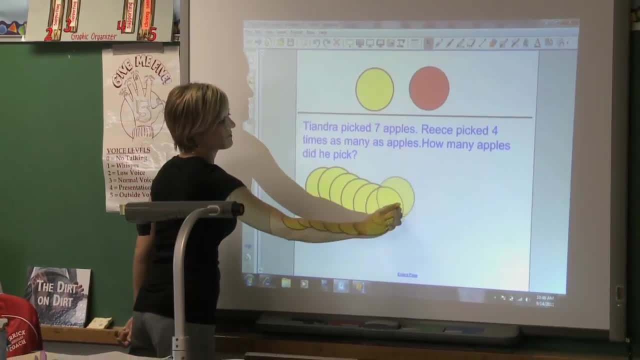 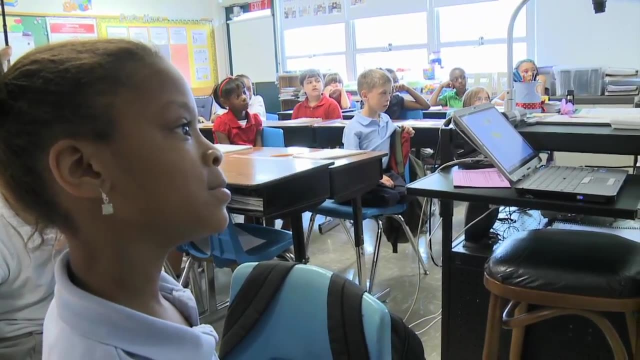 Five, Six, Seven, Eight- Oh, what's this? say Seven apples, Exactly. I'm going to make this page just a little bit longer. All right, Seven apples. Tiandra, did you have fun picking your apples? I like apples. 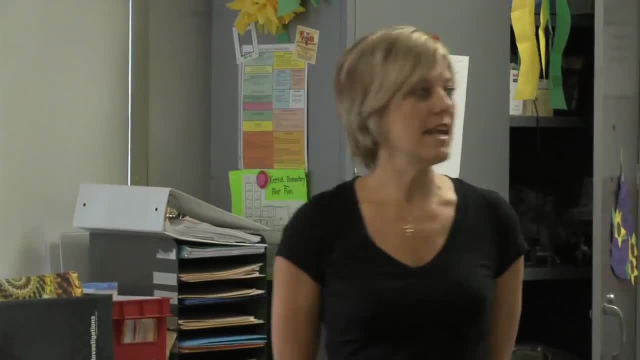 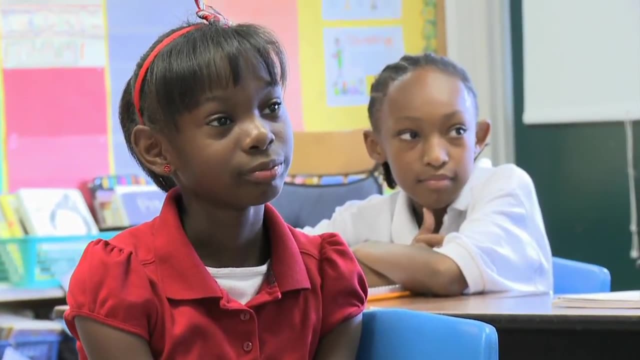 You like apples? Cool, All right. Reese comes along and he the story says. he picked how many more, or how many times more? Four, Four times. Who wants to show me the one time, The one time, One time? 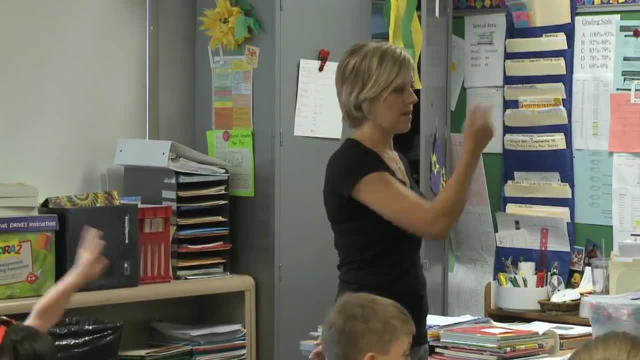 One time as many as Reese. One time as many as Reese, Jacob, all you got to do is your apples are going to be red, Reese Tiandra, yours is yellow, So you're going to show me one times as many. 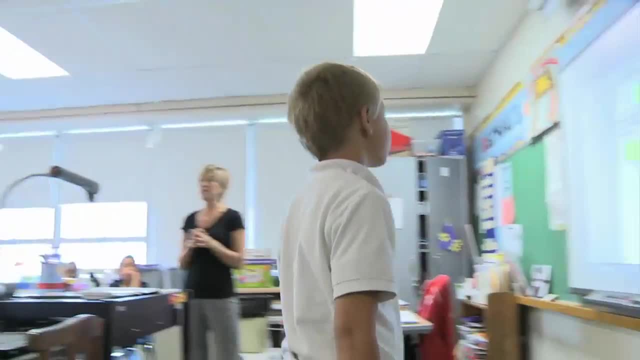 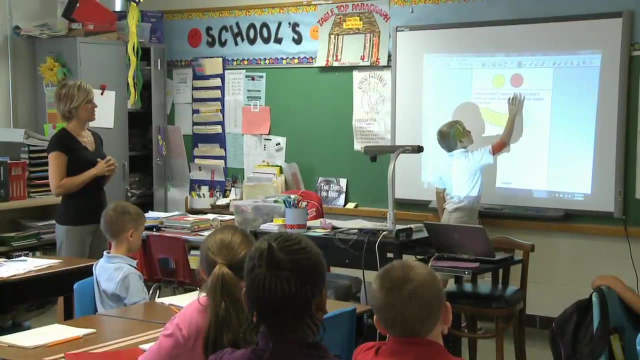 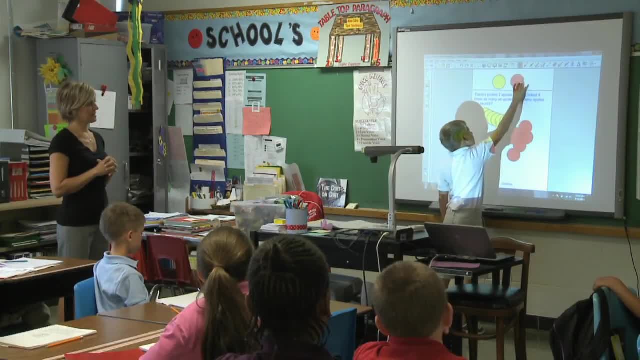 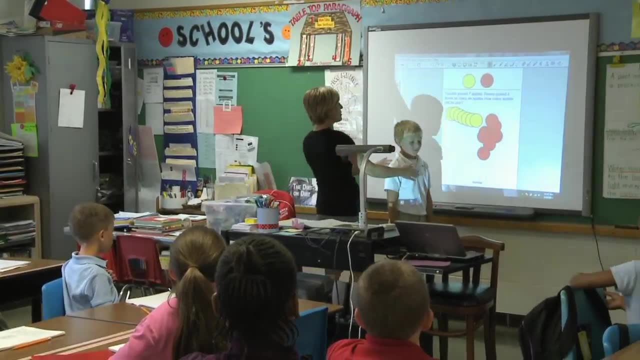 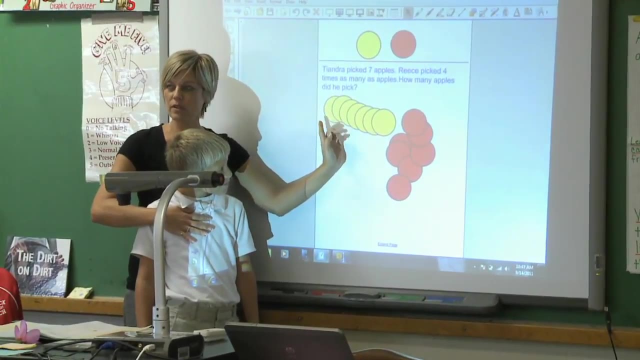 Two, Three, Four, Five, Six. Good job, Are you done? Good job That, for let's get back because we're in our, we're in the thing. This shows that one times as many as who Tiandra. 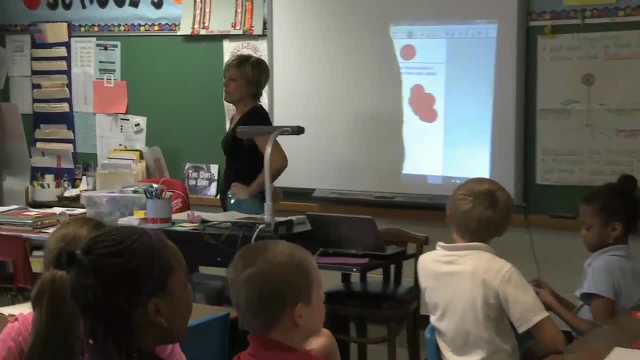 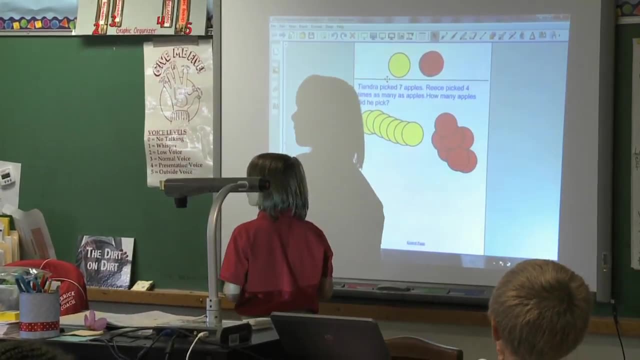 Tiandra, That's one. Okay, All right, Trent's ready. Jacob said he's ready. So, Trent, you're going to show us two times as many, but you got to use what Jacob already has on there, Okay. 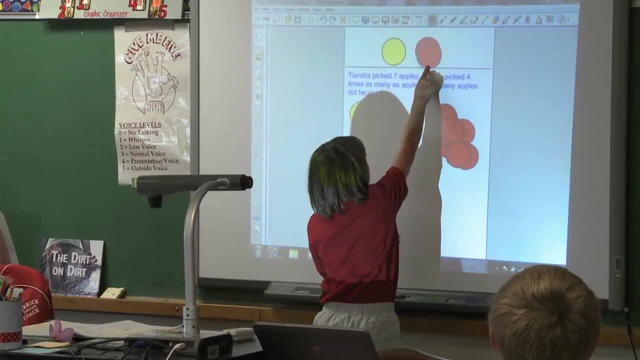 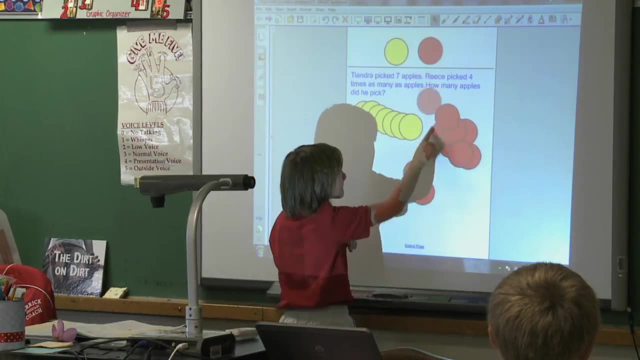 Keep, do what you do your stuff, Do your stuff, Do your thing, Do your thing. One, Two, Three, Four, Five. Oh, just click off of it. There you go. This is Five, Six. 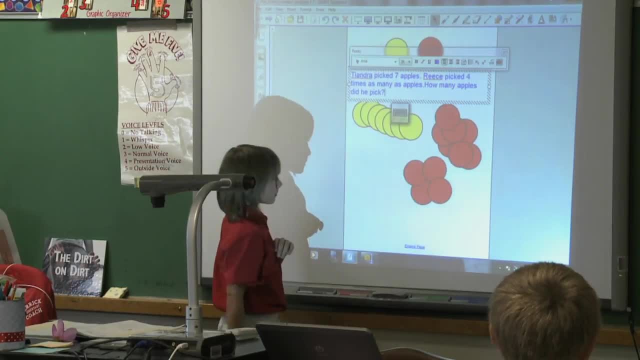 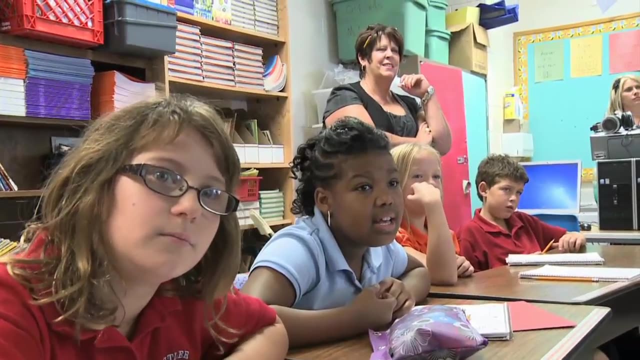 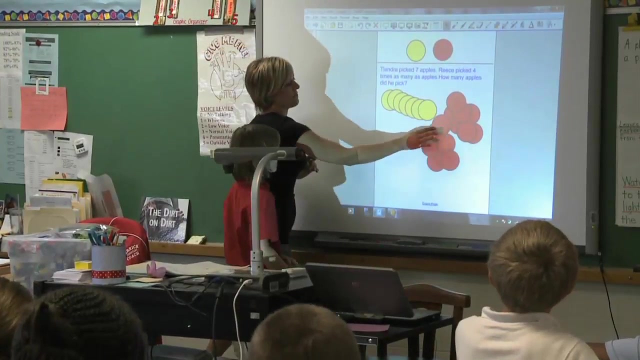 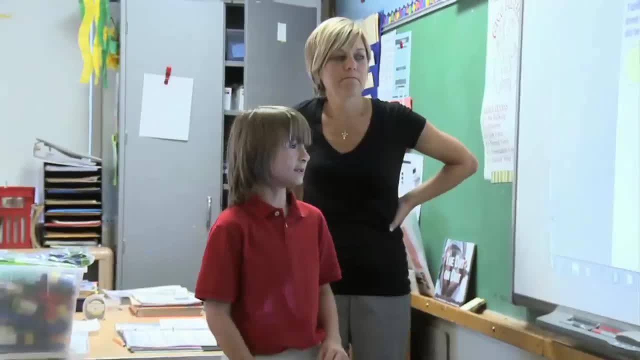 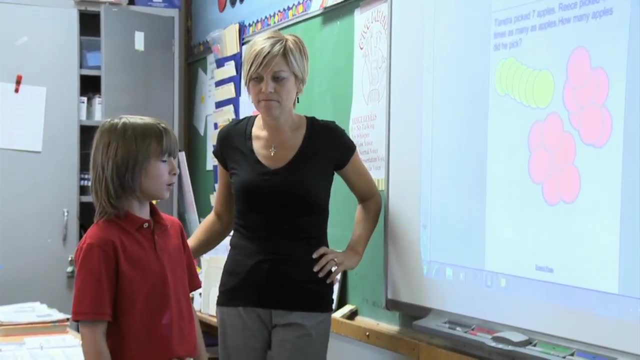 Okay, Okay, Yes, I'm finished. Tell me why I said: show me two times as many. Because I put seven. Wait me, Show me two times as many. I did seven apples. You did seven apples. Is that a group of seven apples? 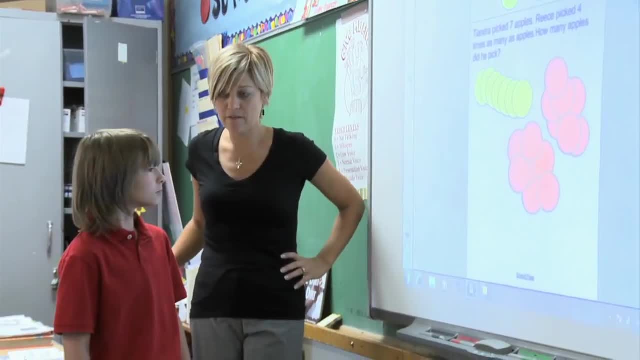 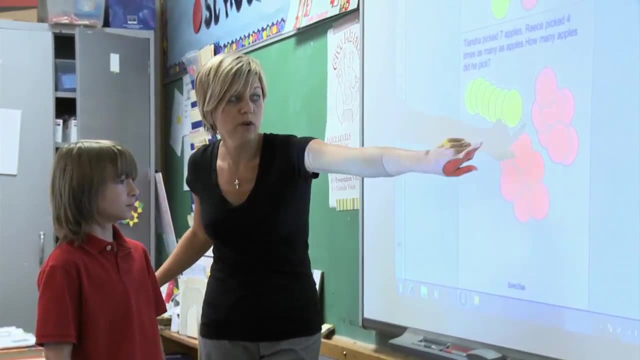 Nope, It's not a group. Er, yeah, You, You, you tell me, Yeah, You think it is a group. Why is it considered to be a group? Because I put seven apples And you put them. We could put a circle. 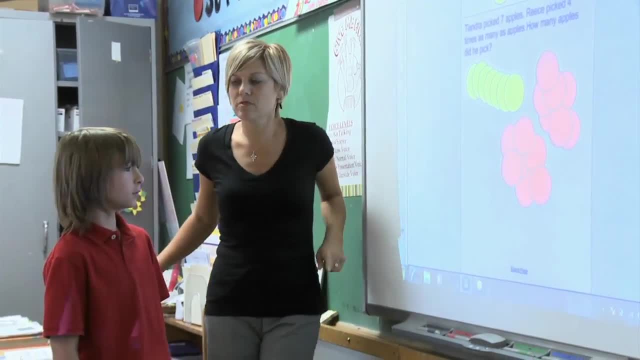 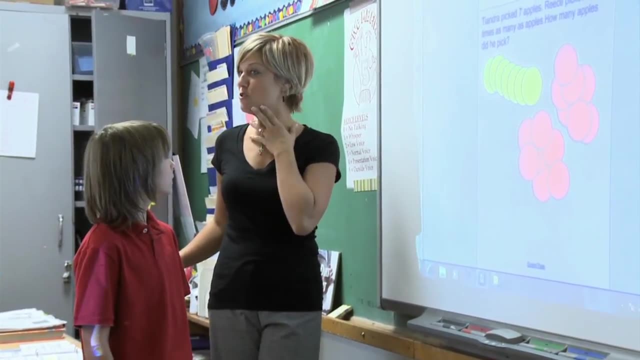 Did Jacob finish? He finished: make a group of seven apples. And what did I ask you to show? Did I say: show two groups of seven? You are interpreting that and that's exactly what I want you to do. That's exactly what I want you. 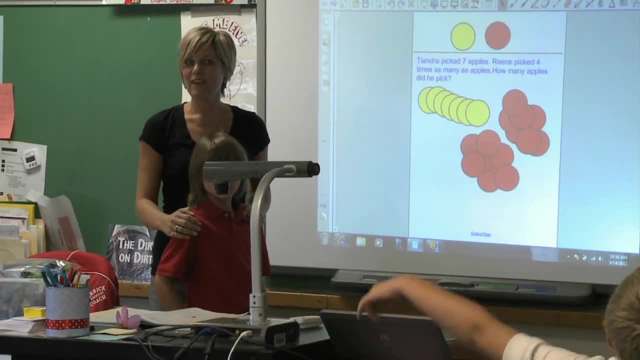 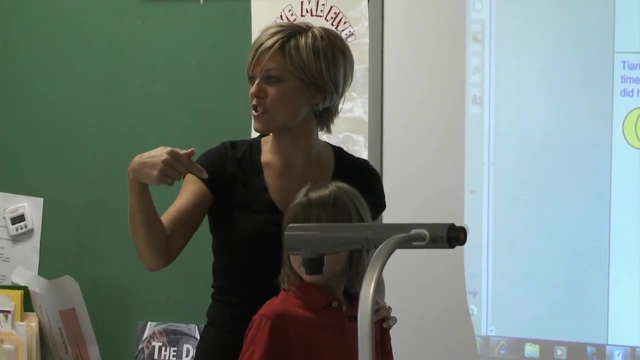 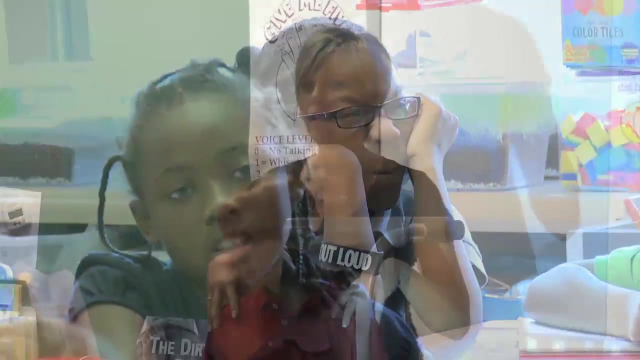 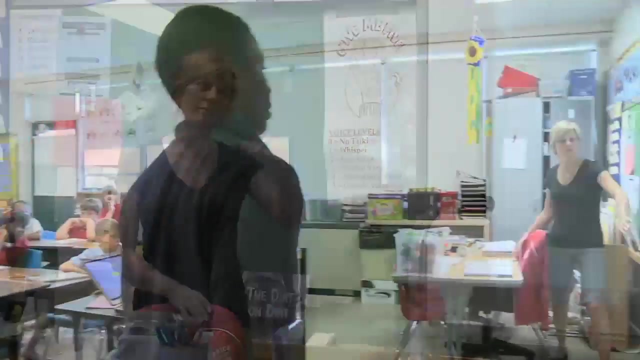 to do. But what did I really say? What did I say? I said: show me two times. But listen to their language. They keep saying: two groups up. Hmm, Are those synonyms, maybe? Maybe, Think about that, Jose. you want to show me three times as many. I'm going to extend this page a little more. 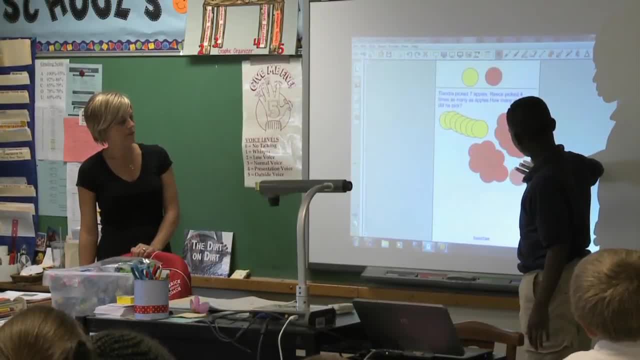 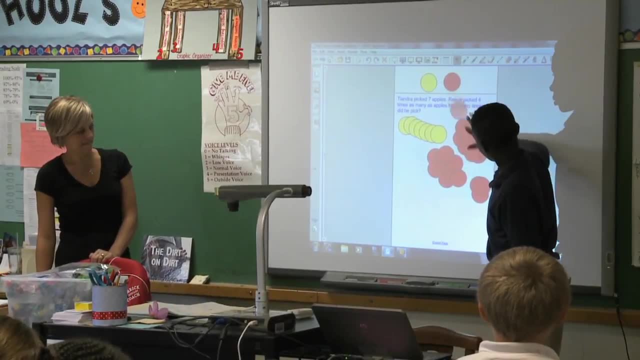 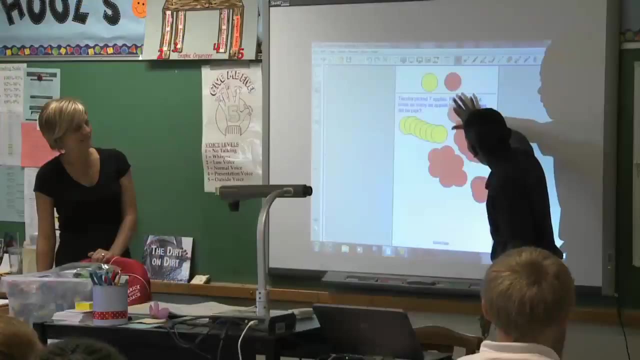 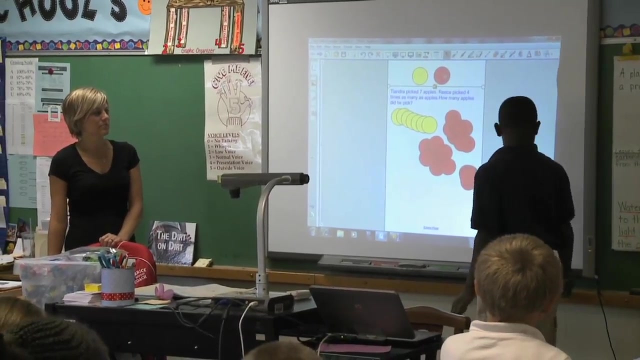 One, two, three, four, five, six, seven, eight, nine. Ah, you caught yourself. Why'd you go back? Because I heard eight and I wasn't paying attention. Ah, heard eight, but he wasn't paying attention. Well, he probably he. 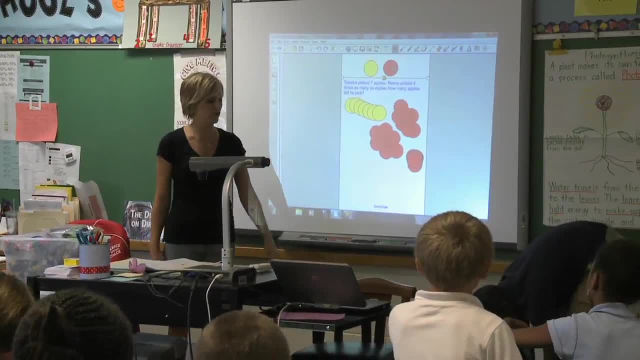 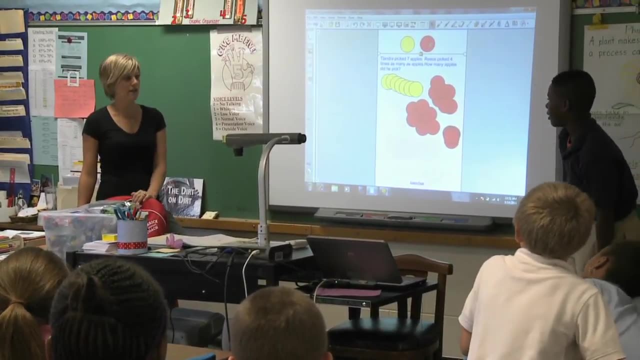 must have been paying attention, because he stopped. If he didn't pay attention he would have kept going. So you did pay attention. So tell me what you got here, Jose. I got 21.. You have 21? How do you know? Because I know that seven times four is seven. Seven times four is seven, Seven times. 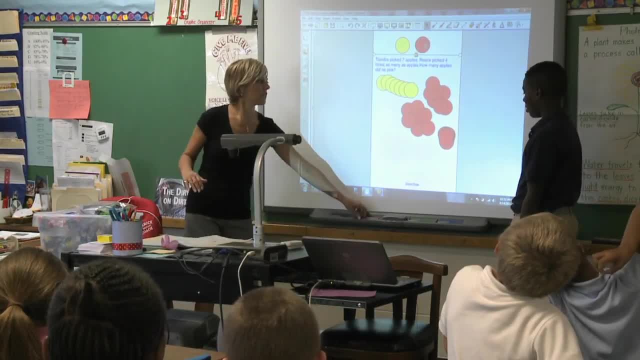 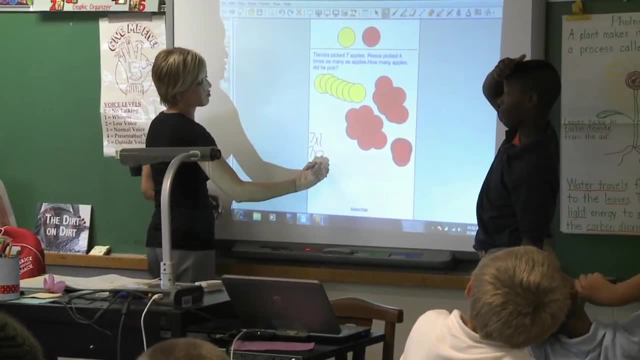 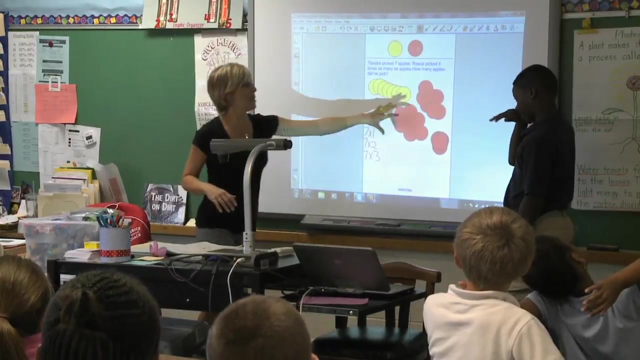 two, 14.. And if you add seven more to 14, you'll get 21.. Cool, So you got. can I'm going to say: do you have seven or do you have how many groups up here? That's what I want to say: How many groups. 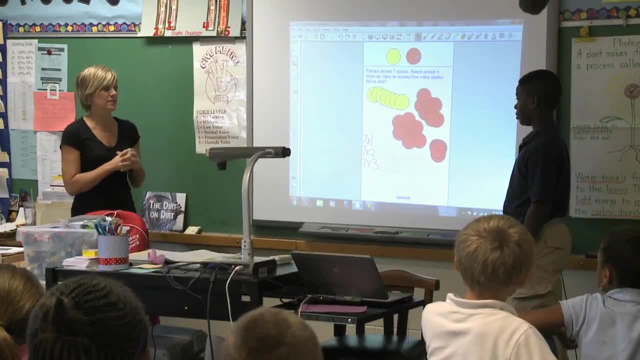 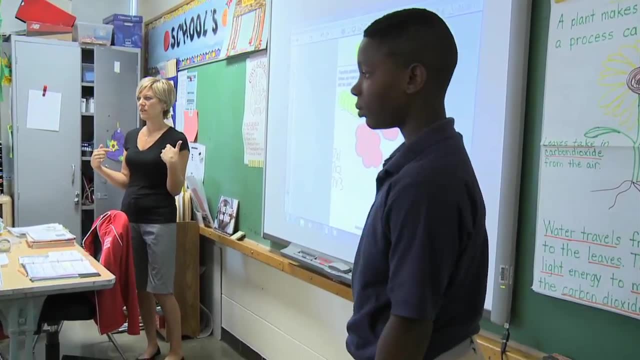 do you have Three, Three. So could I say you have three groups of seven? Yes, Can. does anybody know the synonym of what I asked him in the beginning to do? What did I tell him? I didn't say: come up here and show me three groups of seven. What did I say? 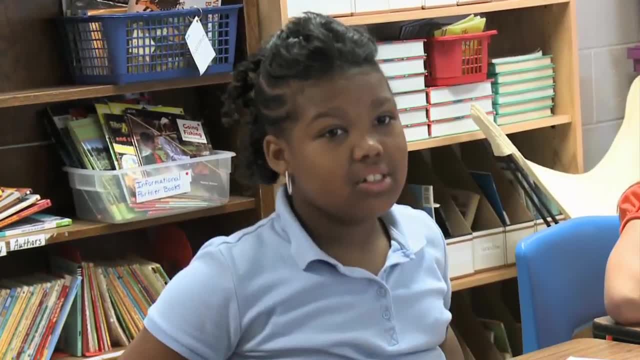 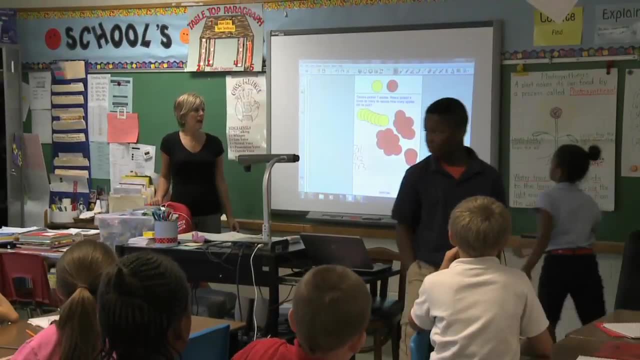 Giovanni, Three times is seven. I did. I said: show me three times is many, didn't I? Three times is many. Good job, Jose. can you pick someone? Dejanay, I need you to show me four times as many. 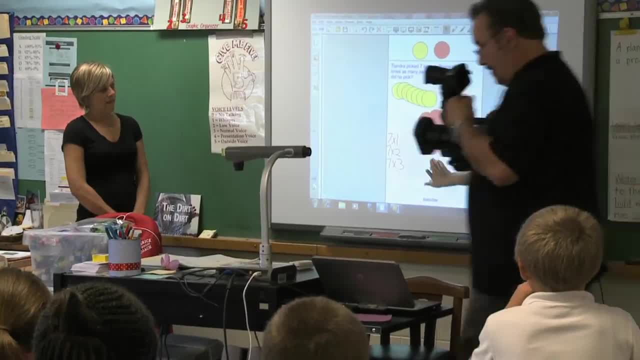 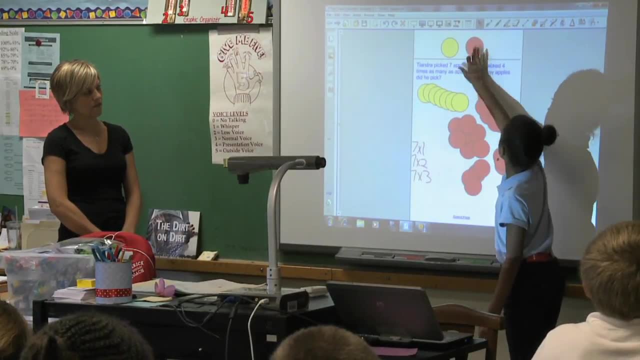 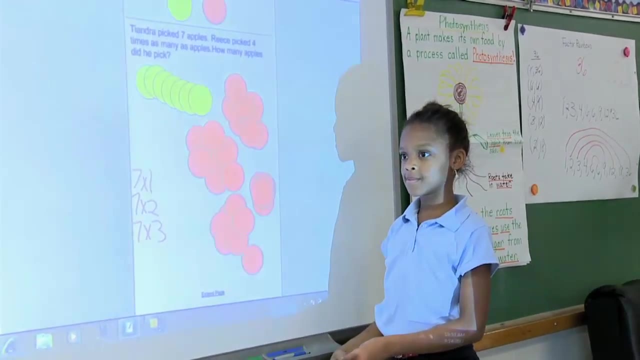 using already what they have: One, two, three, four, five, six, seven. Are you finished? So can you explain what you have up on the board, using all your peers' stuff too? Four times seven. You have four times seven. 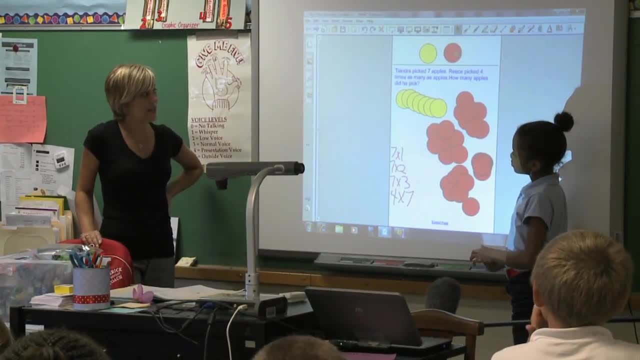 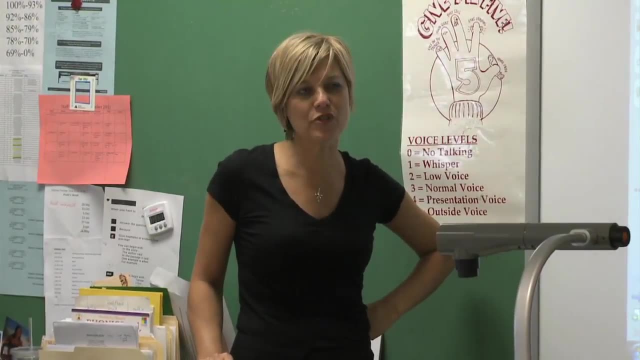 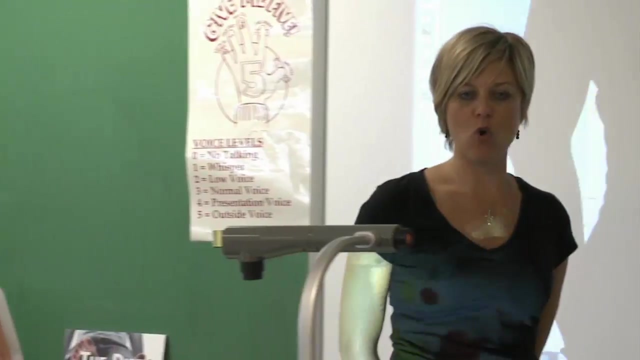 Do you have four times as many as Tiandra? Yes, Yes, you do. So tell me, are we finished? Yes, We're finished. Okay, And how do you know? Think, Are we finished with the story? How Do You? 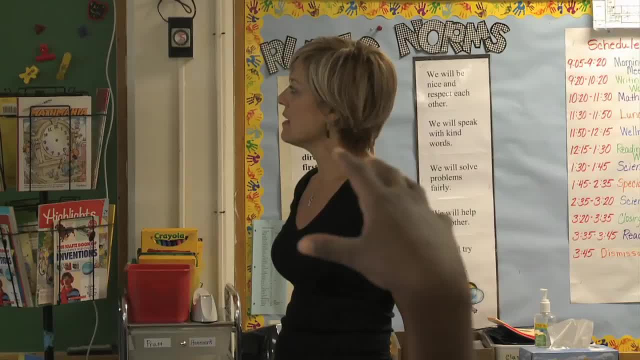 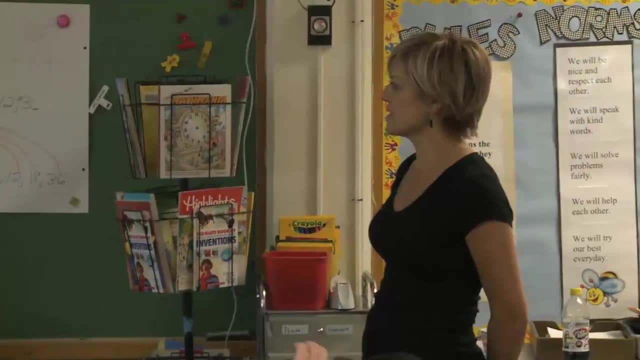 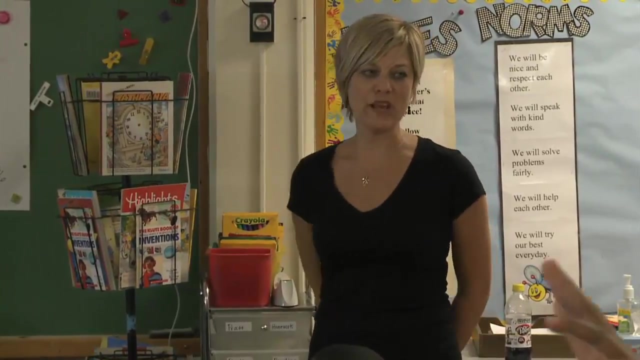 Know I'm going to read it out loud because I think some people might need that. Tiandra picked seven apples. What color are our apples? everybody Yellow. Good Rhys picked four times as many apples. How many apples did he pick? Are we finished with our story? Did? 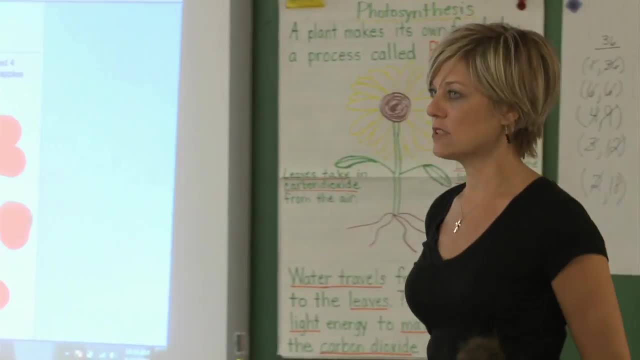 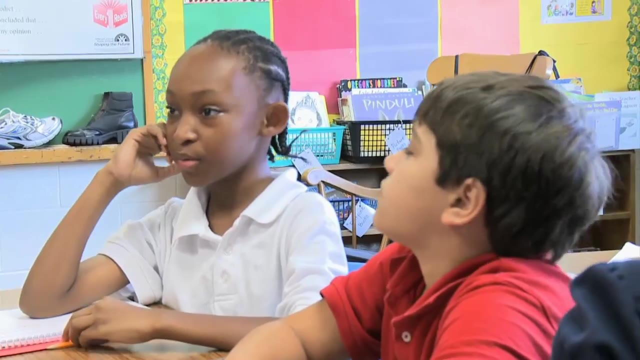 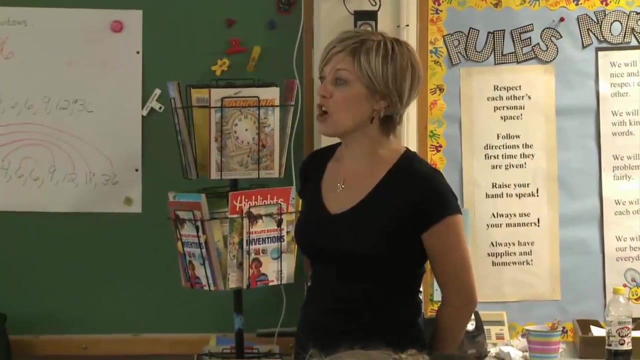 we solve our problem. No, Talk to me about that. Talk to us, Because we have to figure out what it equals. Have we done that? No, How many of you think we've shown what it equals? What should go with our picture to make it very clear that we have an answer? We've got some. 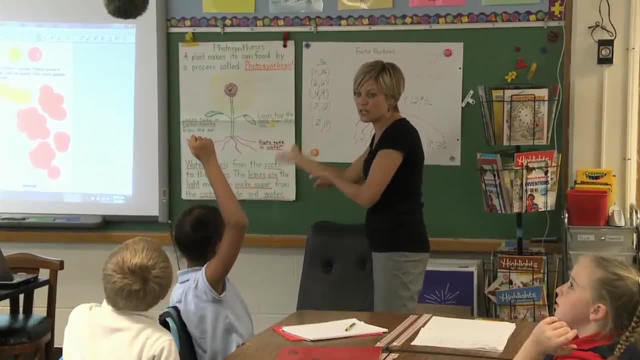 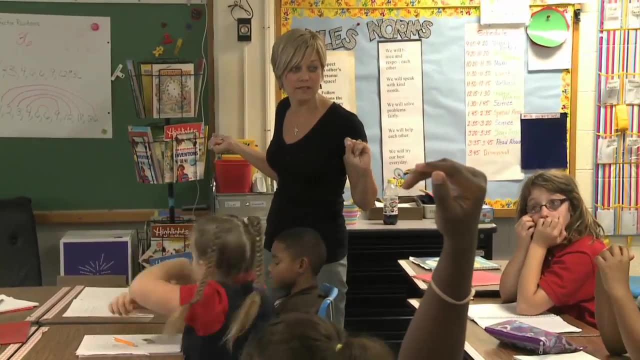 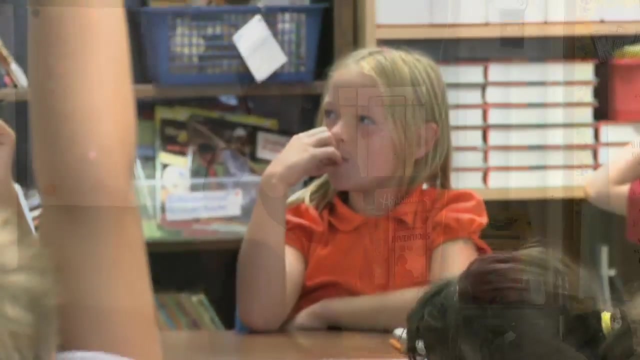 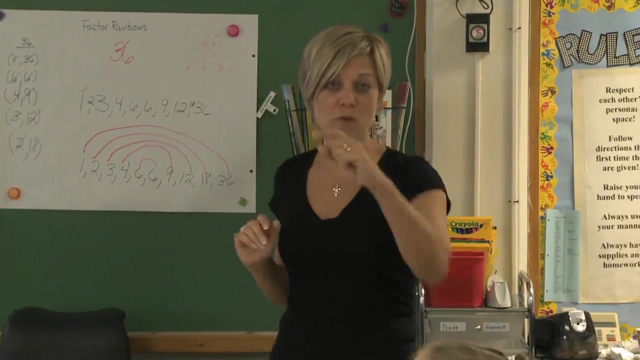 equations up here. We've got a visualization, a picture up here. What else would even make it better? Total: What is the total, Kaylee? Twenty-one, Kaylee, what were you going to say? Twenty-one, Twenty-one, Jose? did you say twenty-one when you? 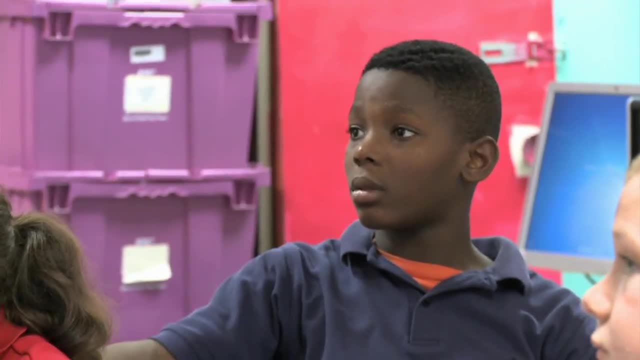 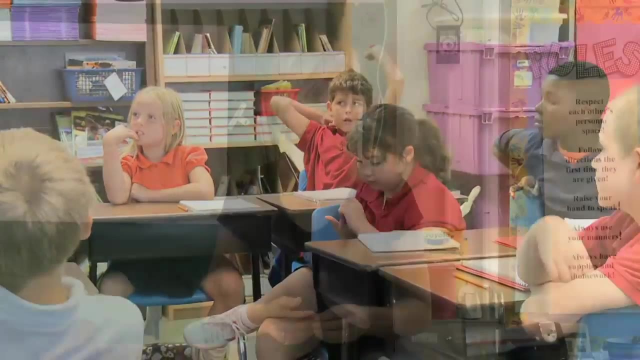 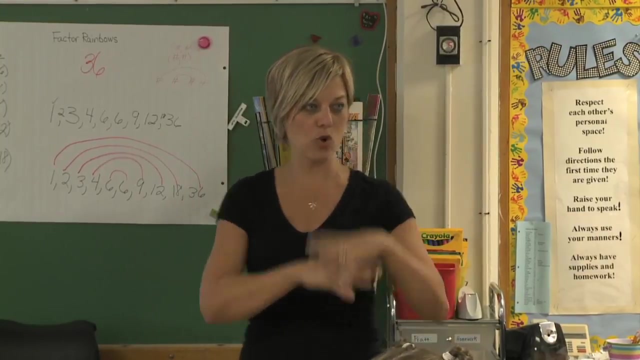 had three groups of seven. Yes, Okay, now there's four groups of seven. so what would we do? Add, Let her do it. Ten, It's four groups of seven. What do we need to add to the three groups of seven? Seven more, Seven more. Get it going. I'm waiting, We're waiting. Twenty-eight, Very. 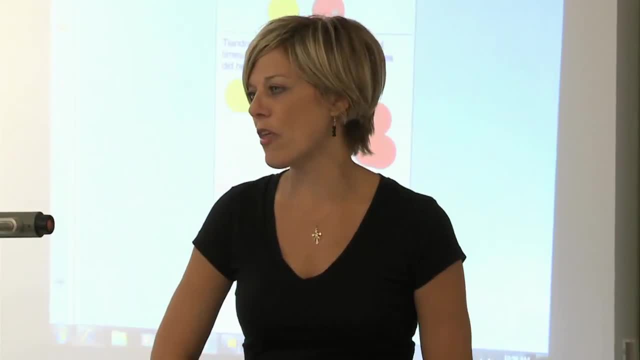 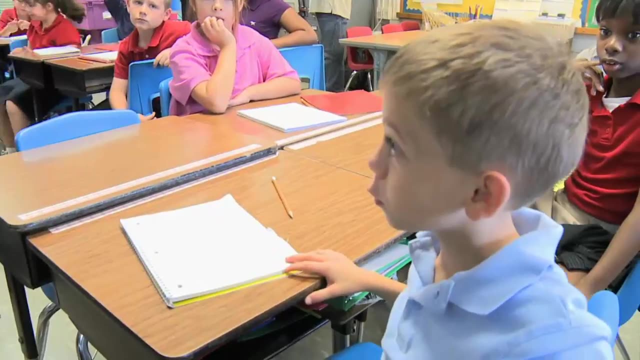 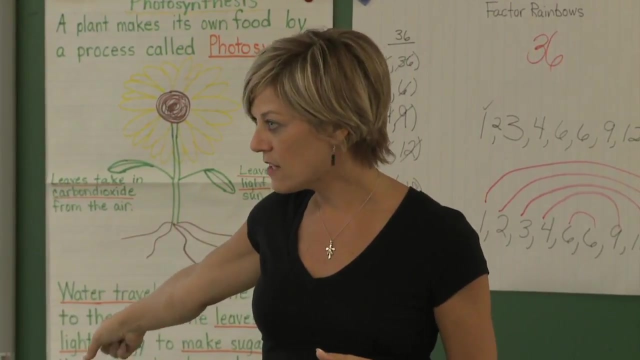 good Twenty-eight. what Twenty-eight apples? Why should we label them? Why should we label every answer in a math story, So the person knows what you're talking about, Absolutely. What's this story about? Apples And we don't want to put oranges. No, We don't want to put raindrops. No, We want to put. 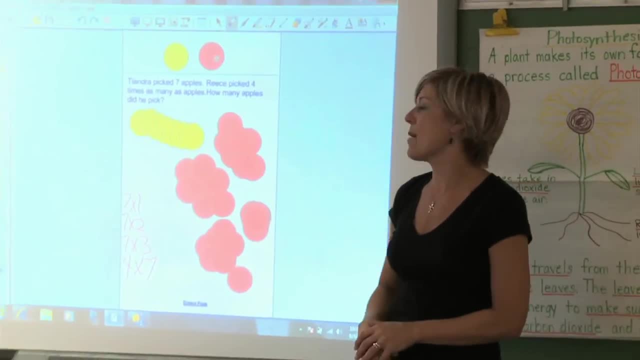 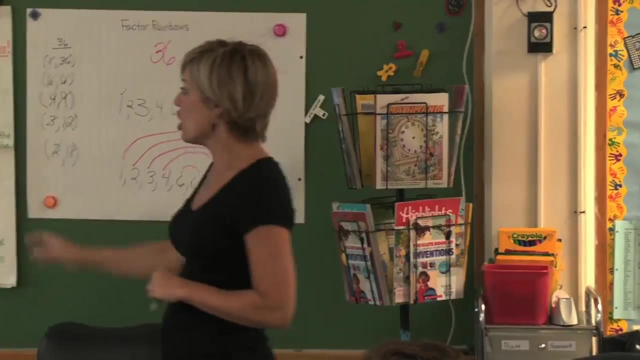 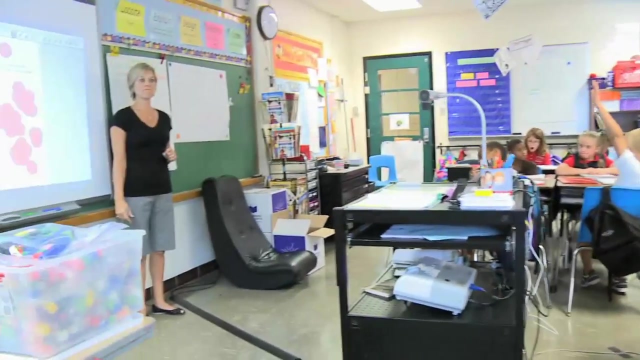 apples. So if I was going to answer the question, how many apples did he pick? Using our visualization, the manipulatives on the smart board, using the math equations that you gave me, what would we put for our answer? Every hand should be up, because good listeners should have heard Kaylee. She worked. 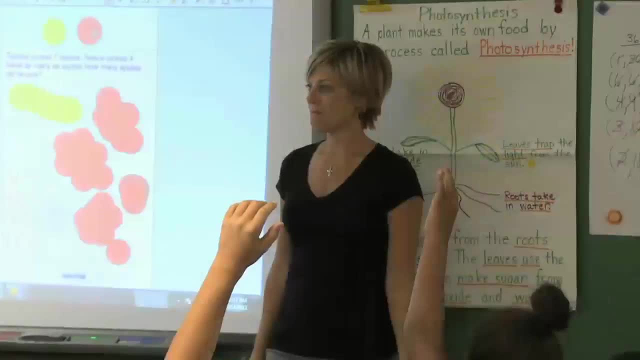 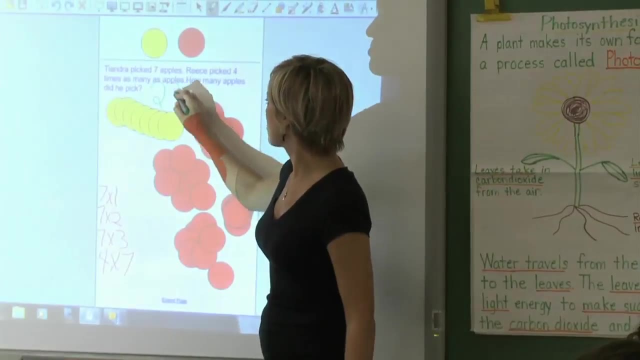 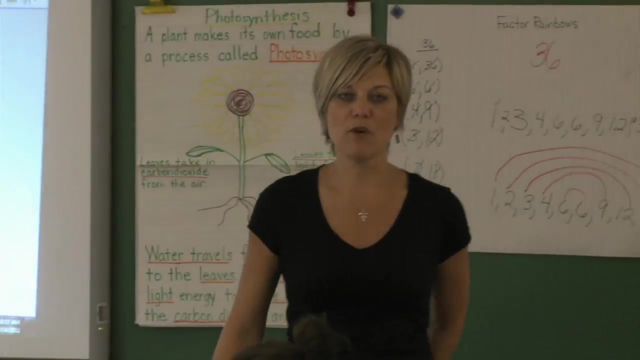 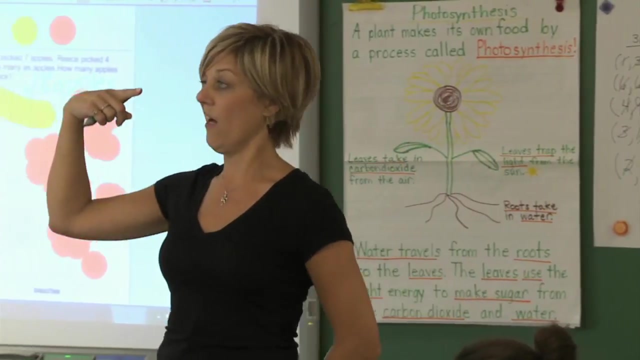 hard on that. Twenty-eight, Iona. Twenty-eight, Twenty-eight, what? Twenty-eight apples? Very good, Twenty-eight apples. That is an example of multiplicative comparison. Are you changing your predictions a little bit? Are you still going? huh, How many of you are like that? huh, It's okay to be like. 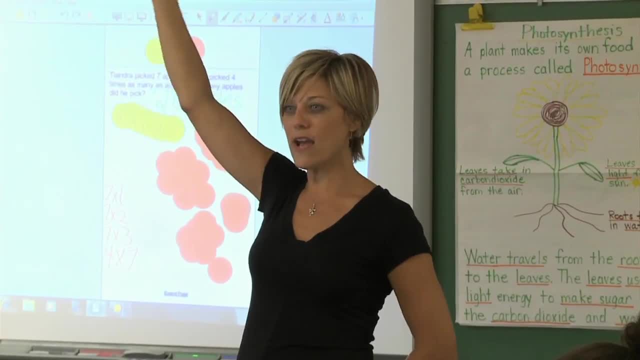 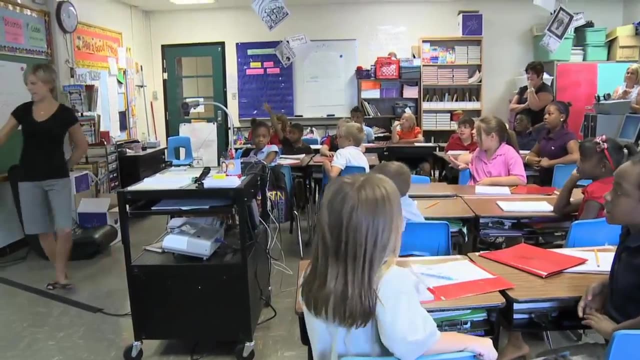 huh, Go ahead, Don't be shy. How many of you are still wondering: oh, I need more help, I want to see it again. Well, guess what? You're going to see it again because I have a feeling most of you are like: huh, It's brand spanking new. I'm going to show you another problem. 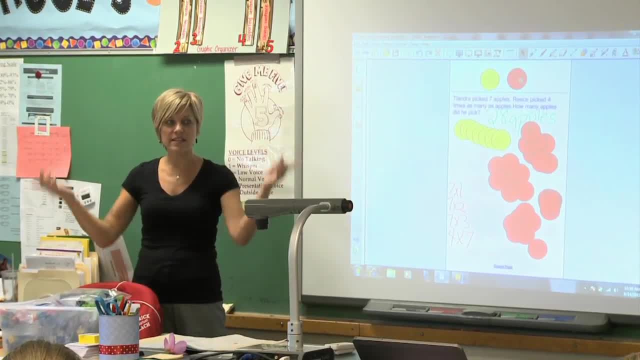 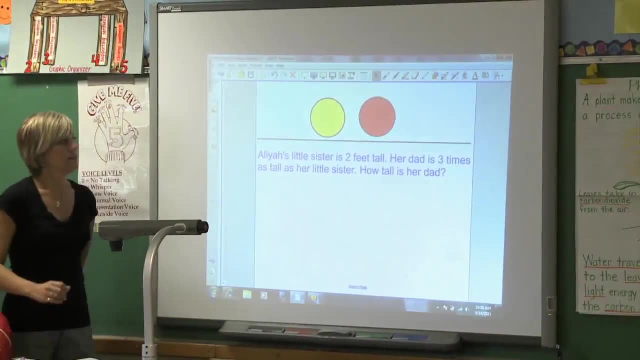 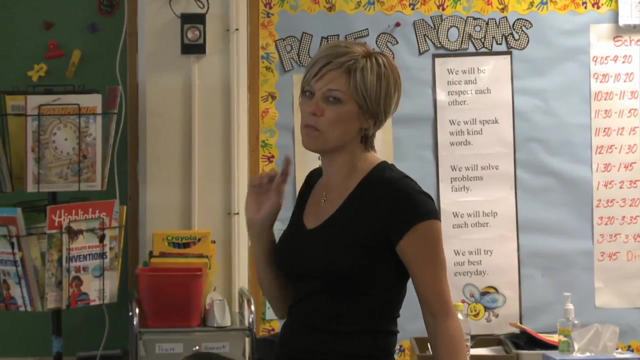 okay, It's an example of multiplicative comparisons. Think about what you were predicting it was all about and let's see if you change your mind. Alright, here's the thing There are. Go back to what you were thinking multiplicative comparisons was all about. 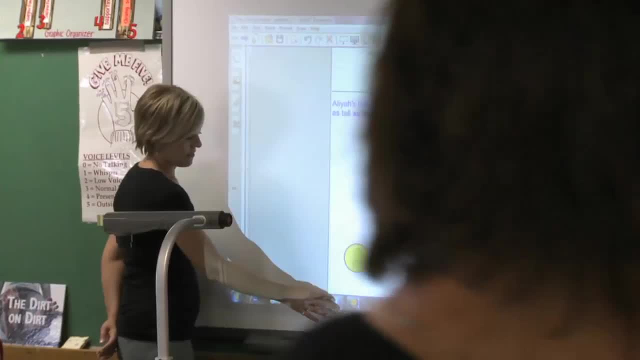 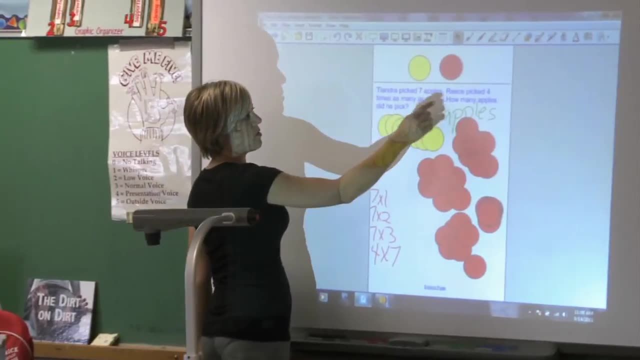 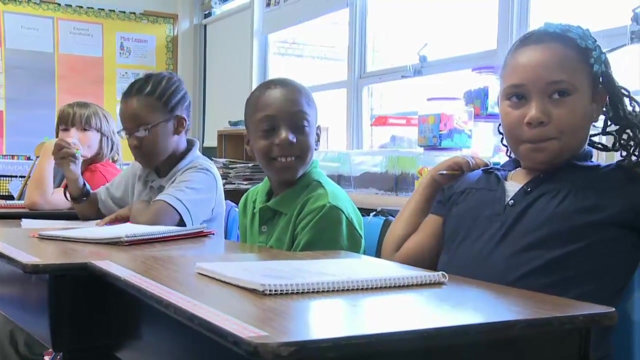 And I want you to focus on the repeated words. I love it, because repeated words is what we were doing in writing. Focus on the repeated words in. Aaliyah's little sister is two feet tall. Her dad is three times as tall as her little sister. 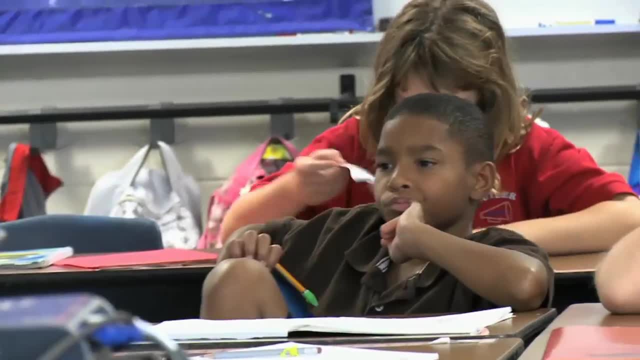 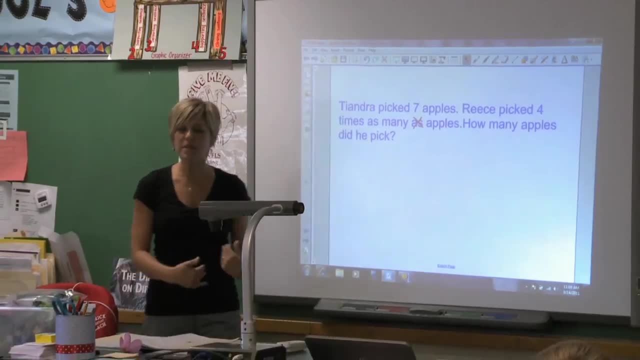 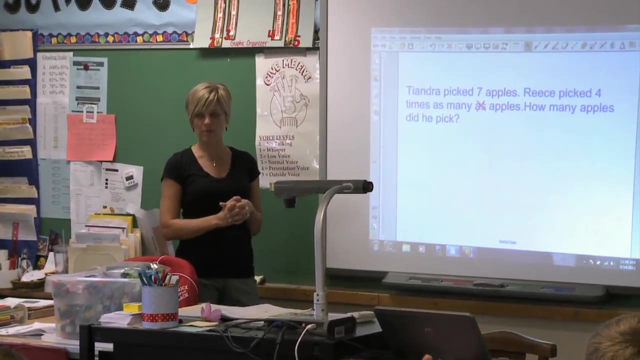 How tall is her dad? DeAndra picked seven apples. Reese picked four times as many apples. How many did he pick? Are there some repeated words in both of those problems? Are there some repeated words in both of those problems? Are there some repeated words? 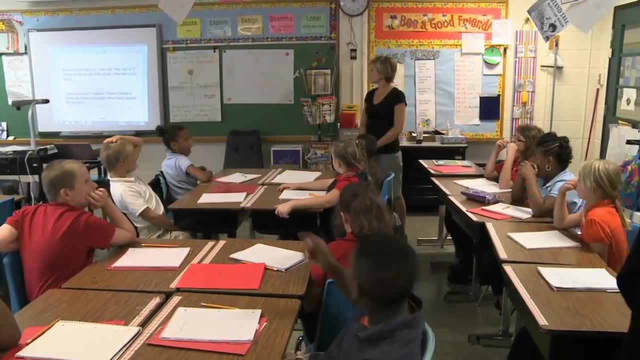 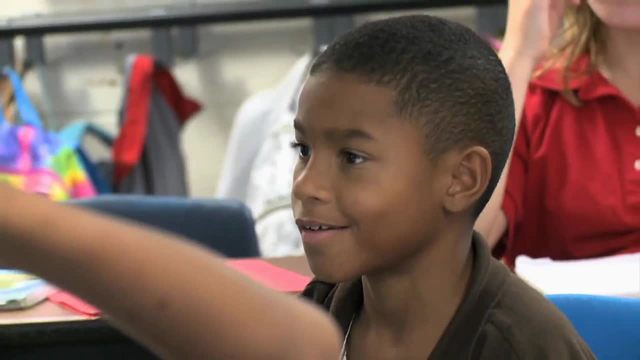 Aaron, are there some repeated words? Yes, what do you see? Picked, Picked. Do you see picked? Oh, okay, I see what you're doing. I want to know. yeah, picked is in your twice, but I want to know if there are some repeated words in both stories. 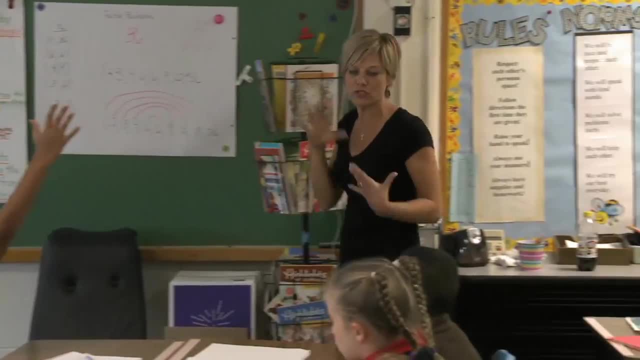 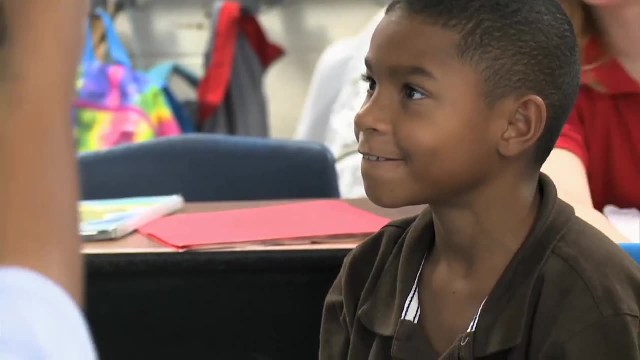 You're absolutely right, So let me rephrase it, Comparing both stories, are there some repeated words? Would you like some help? Are you thinking More time to think or help, Help, Help. Call in somebody. Yeah, they can help. 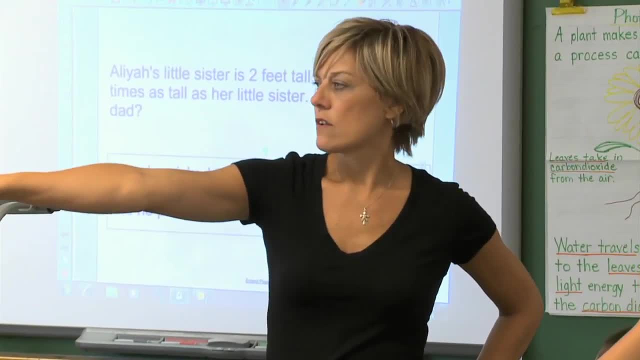 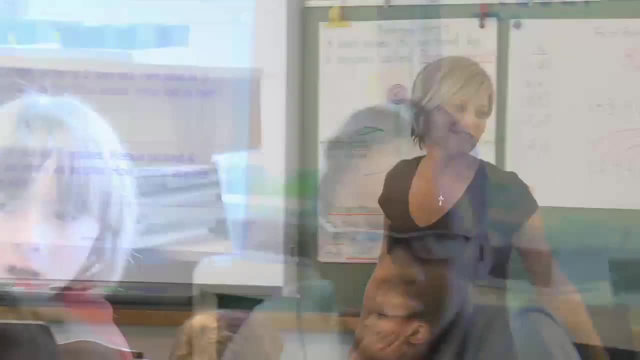 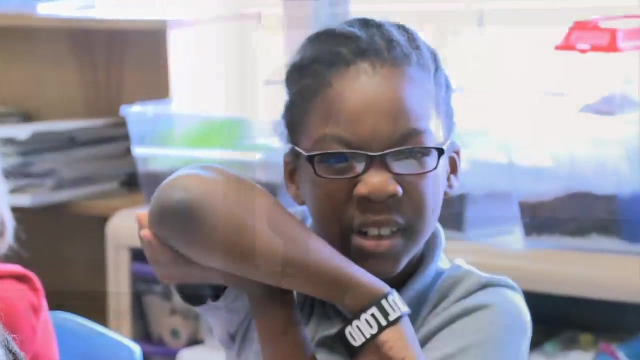 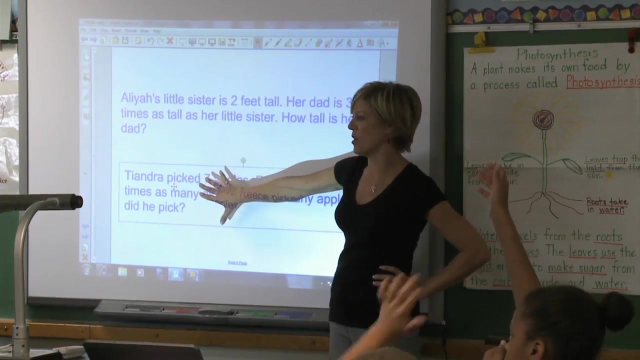 Who DeAndra In the white shirt, Reese The gray shirt? Oh, I don't want it. Yes, What are they? Little sister and apples? Little sister and apples- Are they all the same words? Oh, I want the words in this one to be in this one. 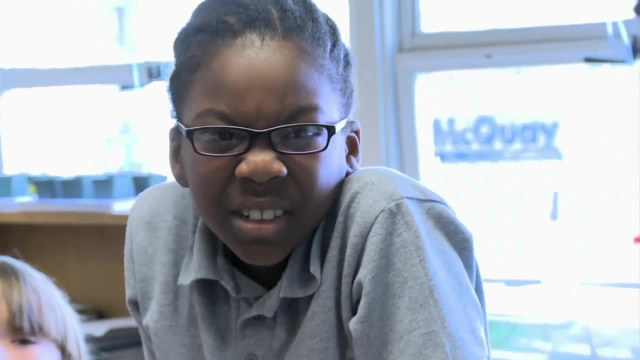 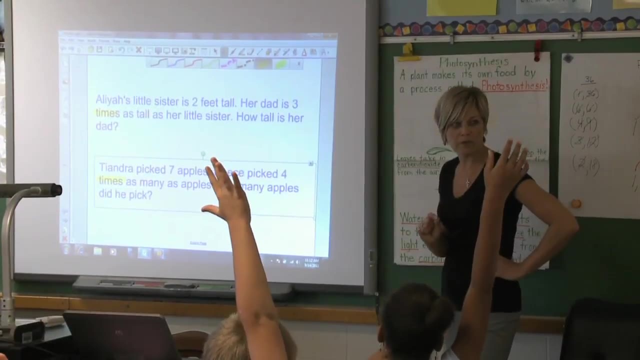 You are picking repeated words. I want the words in one story: Times Times. is that all? And If there's just one little bitty word, then we should probably do it. How Huh, How No, I'm not thinking that one. 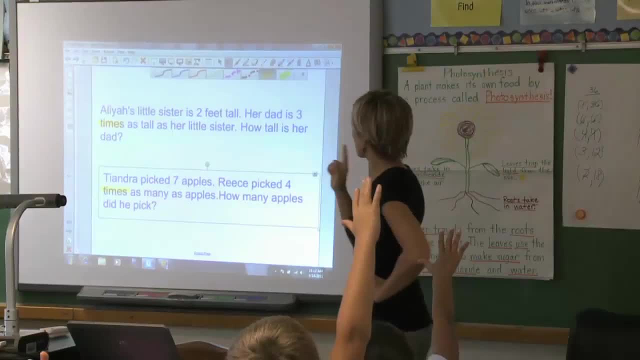 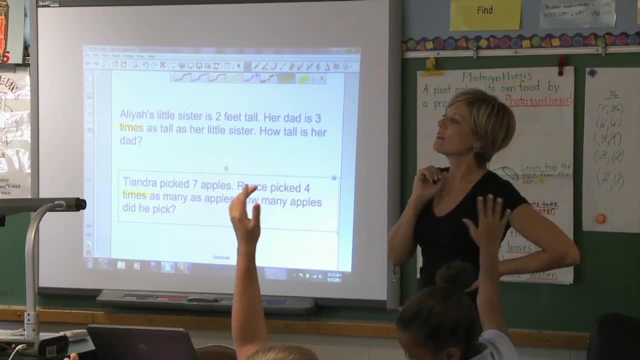 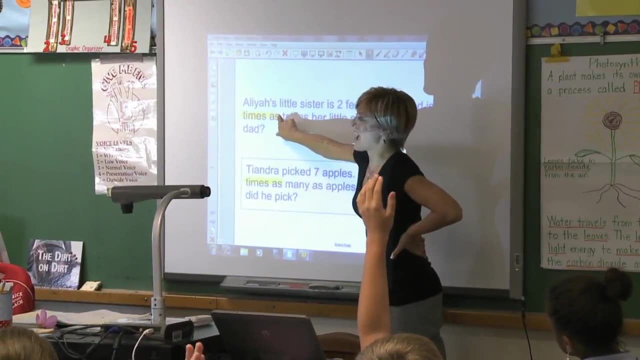 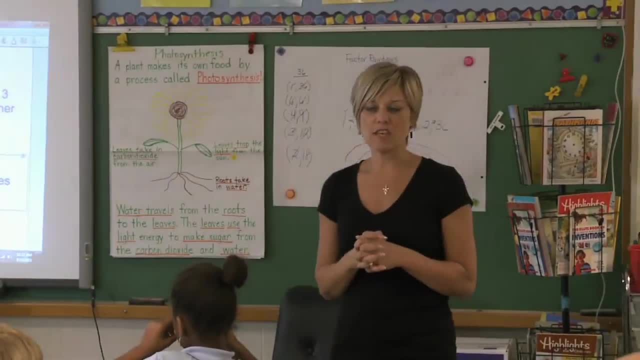 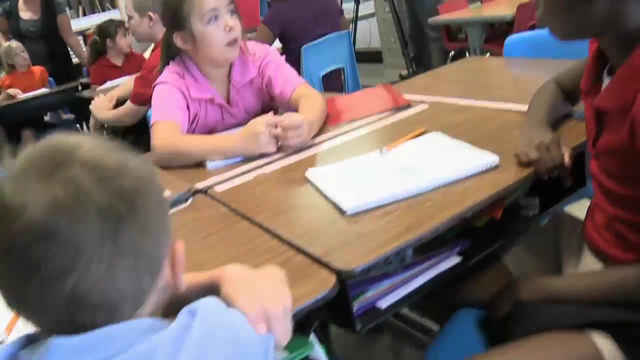 This one's times as many, Okay, So think, Go back to your think. pair and share, Think about multiplicative comparison. Go back, Okay, Okay, A two, three, One, two, three. A two, three. 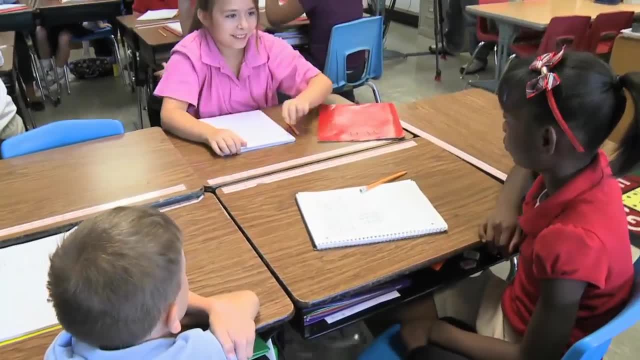 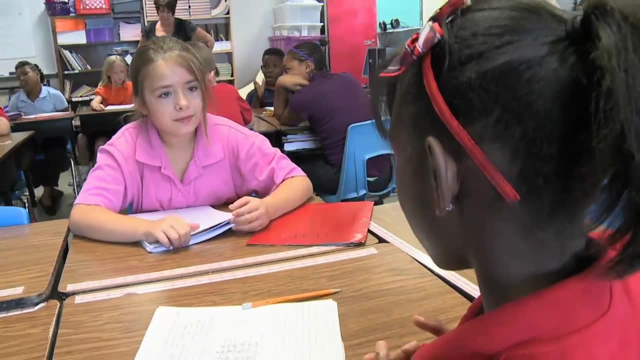 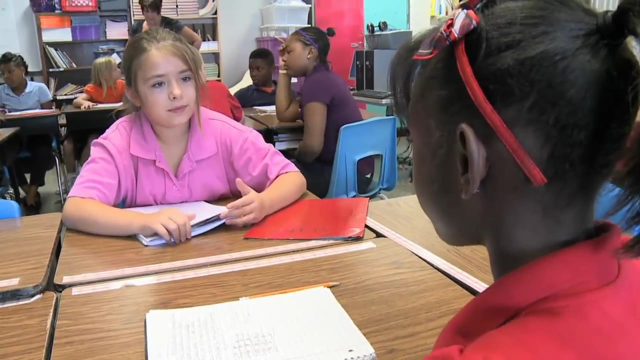 One, two, three, I've been thought- Multiplication comparisons. You go first again. Oh, What does that mean? Uh, Still, I think it's where you can like the community and try to make them like, balance both, and I guess that's all. 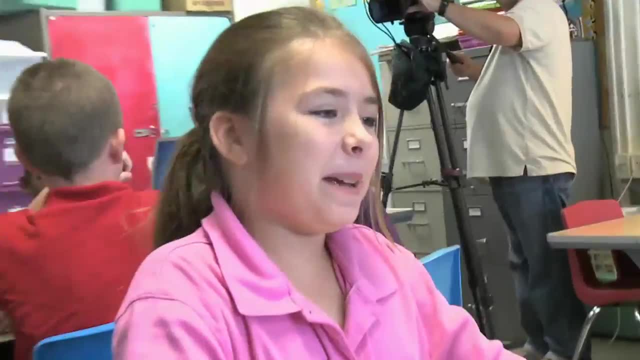 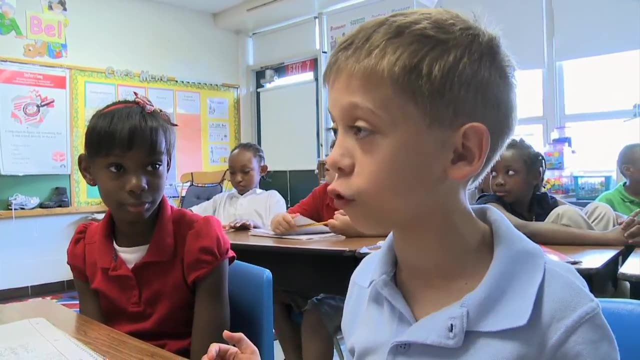 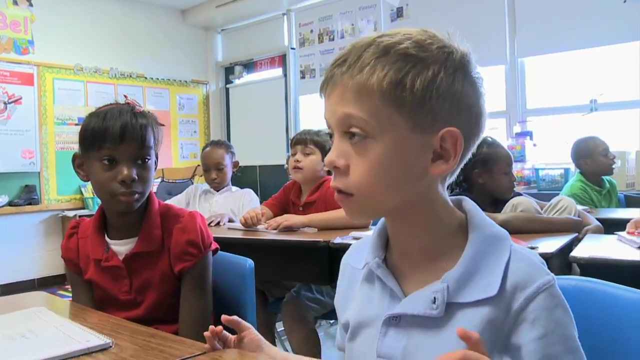 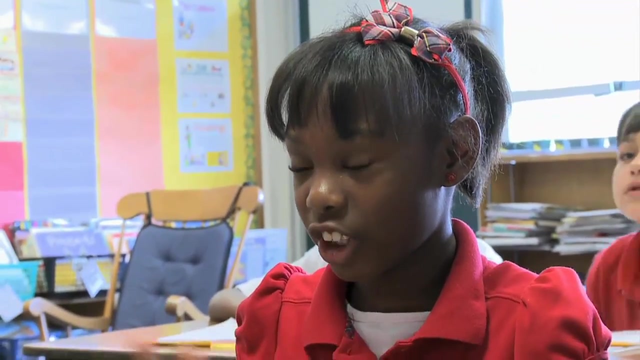 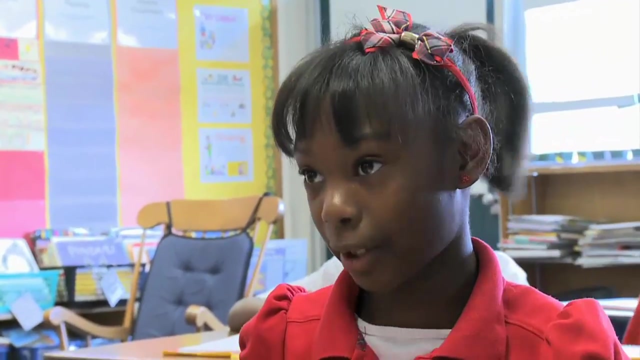 I think it's the same thing where you can keep them balanced. It's like a story problem and it can like help you with story problems like math, about counting and multiplication. I actually think, like I think it's actually like where you can- I'm like trying to chunk it so like it's like in the word- like um, like compare it, like compare it for you know- balance it. 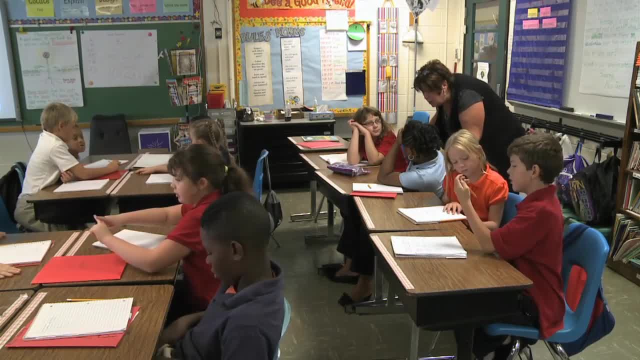 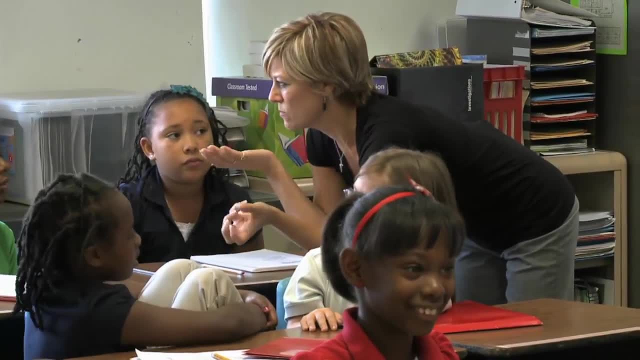 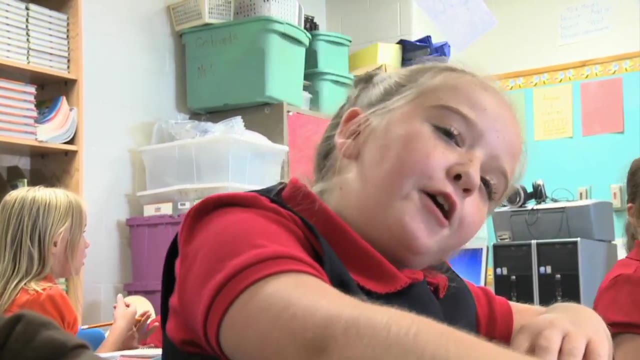 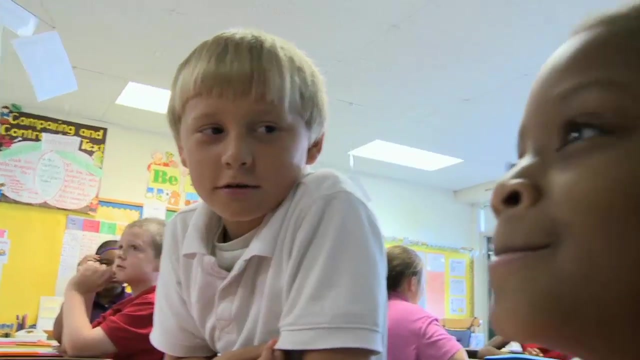 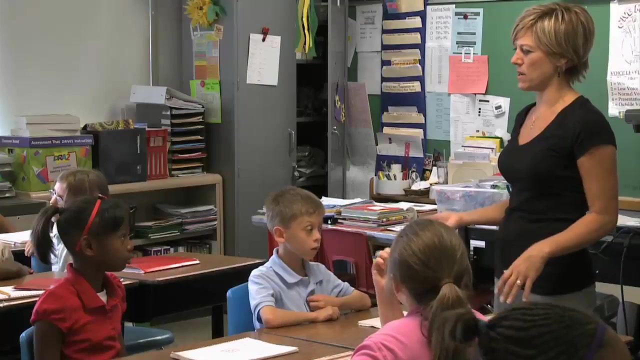 Do you have anything else to say? No, Think about like, choose what you can and think about how they want to balance it. I think we can do pairs. Wait a minute. when I look at the picture, I see two on this side and six on this side when you were talking about your dad. 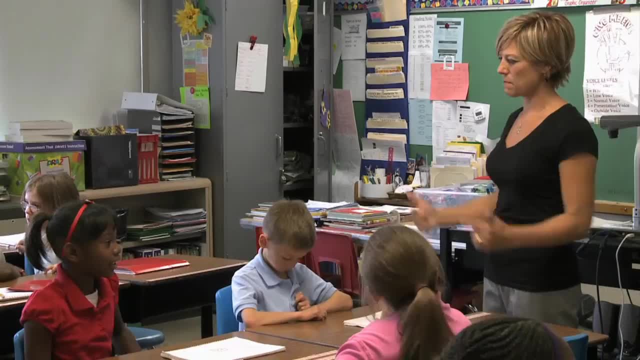 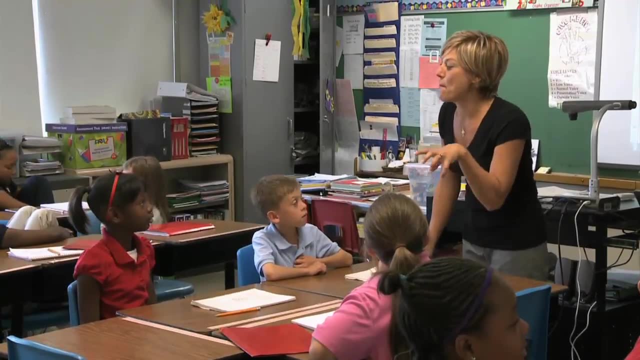 Is that balanced? So what do you mean? You're going to have to explain. You're going to have to explain balance. to me, It's like you can say: you're commutative. Ah, So you're saying balance for another word for commutative. 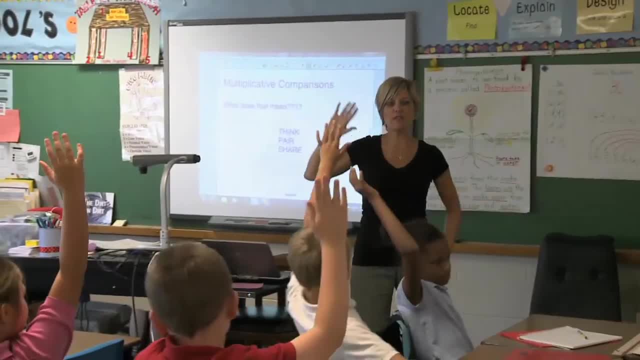 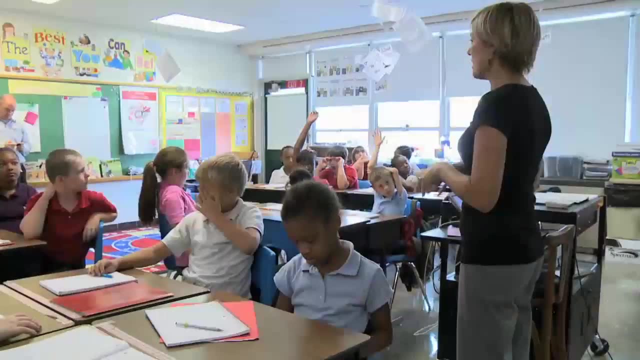 Gotcha. Okay, give me five. Does anybody want to share their thoughts now? Did your thoughts about multiplicative comparisons change? Because I know in the beginning a lot of people say we're going to compare multiplication problems, Multiplication problems. 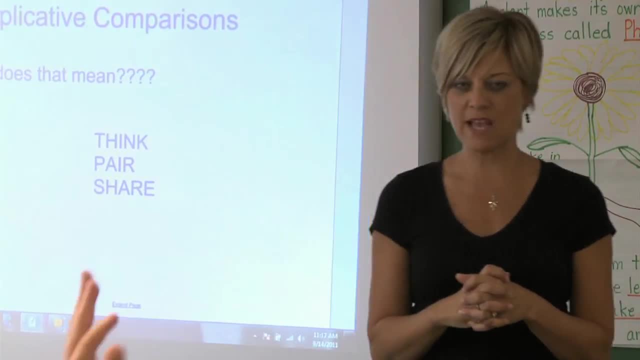 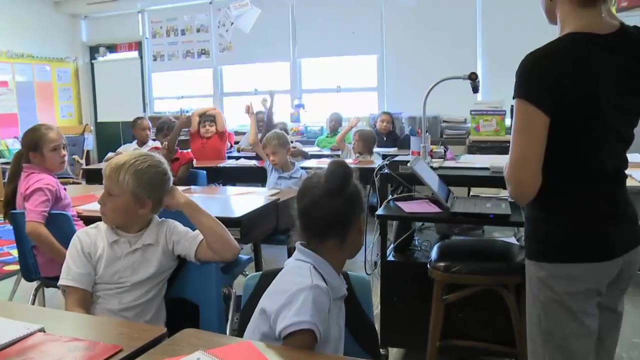 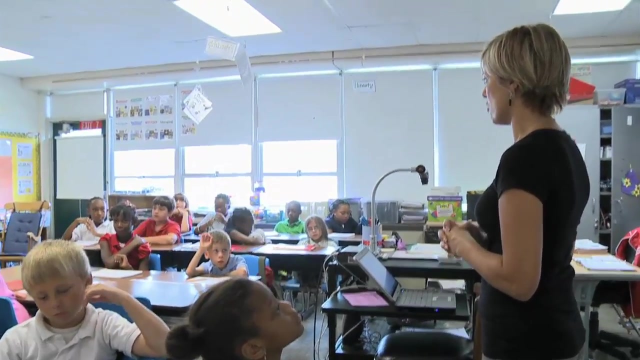 Is that really? That's exactly what we did. Did we compare multiplication problems, Yes or no? Yes, Thumbs up. if you think we did compare multiplication problems, Okay, Explain why we did that, How we did that. If we were comparing multiplication problems, can you explain it? 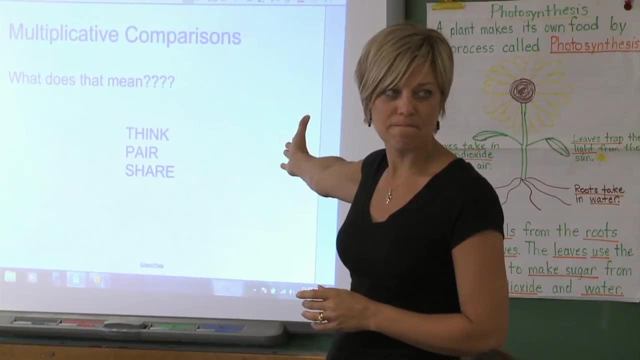 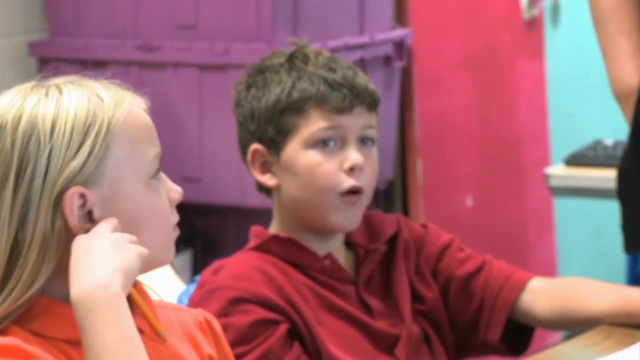 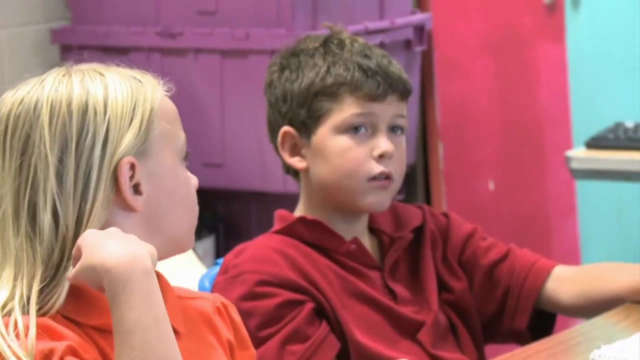 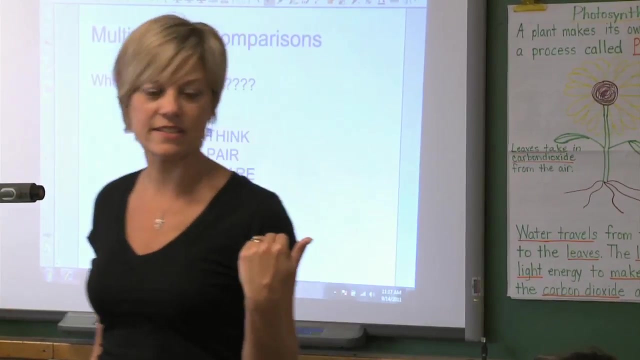 Do you have evidence to explain it? Yes, Matthew, We compared two words that were both in them. You compared two words in them. Did those two words have to do with multiplication? Yes, Okay, Did we compare multiplication problems? Because if you said we did it, you've got to prove it or I'm not going to believe it. 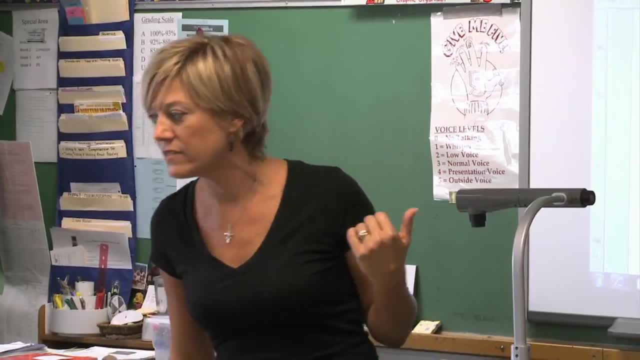 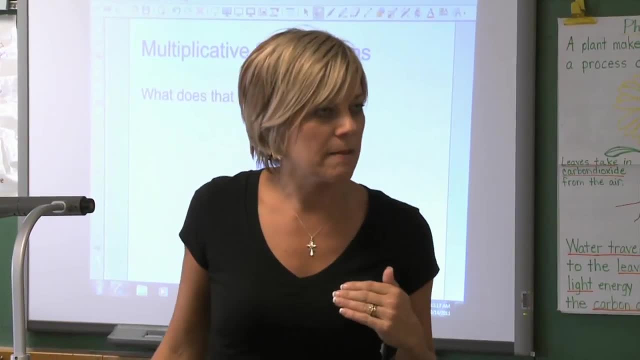 So you people that just raised your hands, you better be thinking about how you're going to prove it, And if you can't prove it, you might say, ooh, now I don't know so much If I really believe that's what we did. 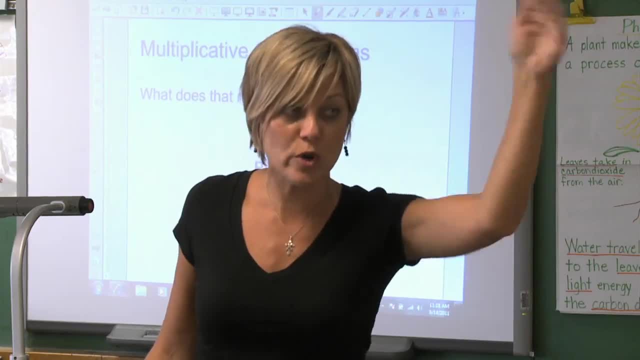 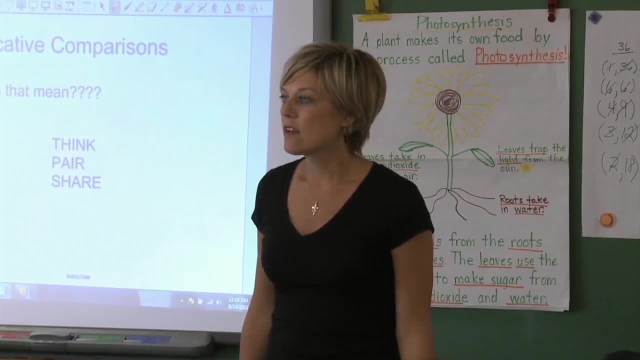 I agree with you. We compared the problems, the word, the story problems And found a repeated word. What do you think we really did? Because what I think- and maybe I'm thinking different than you, but when you all say we compared multiplication problems, 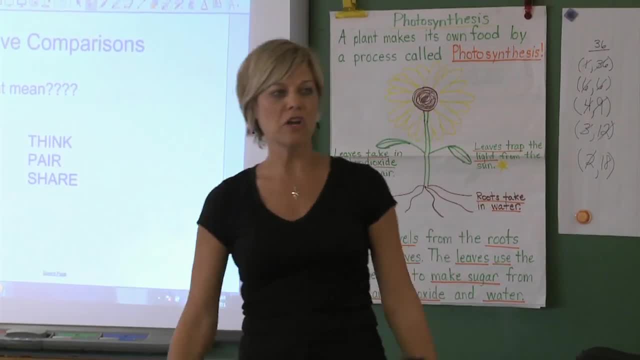 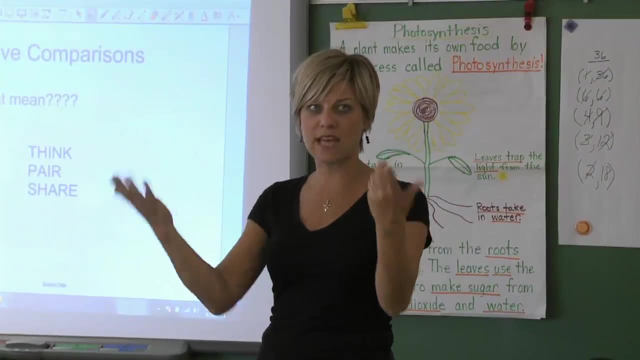 I'm thinking I compared seven times four to two times three. Did I do that? No, No, Well, that's what I'm thinking, because that's what that means to me. So who can tell me what they think multiplicative comparison means? 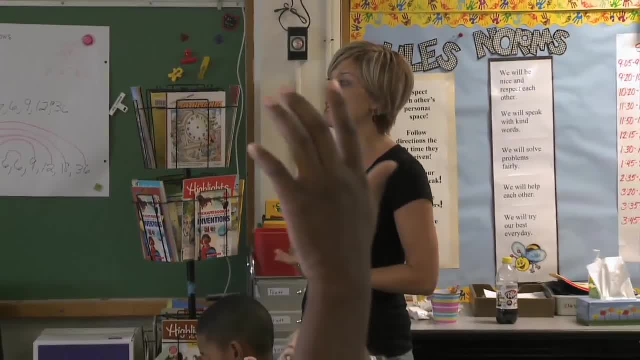 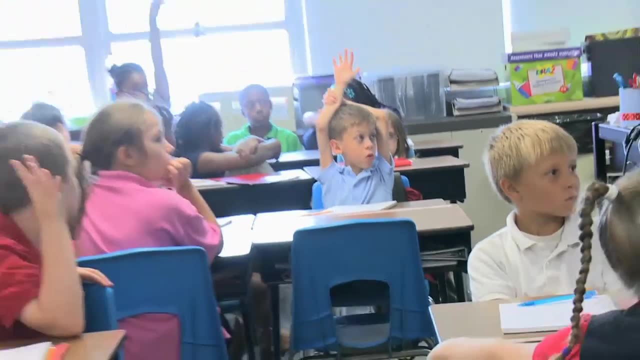 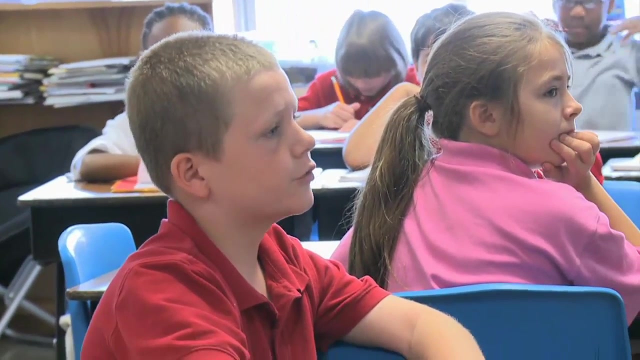 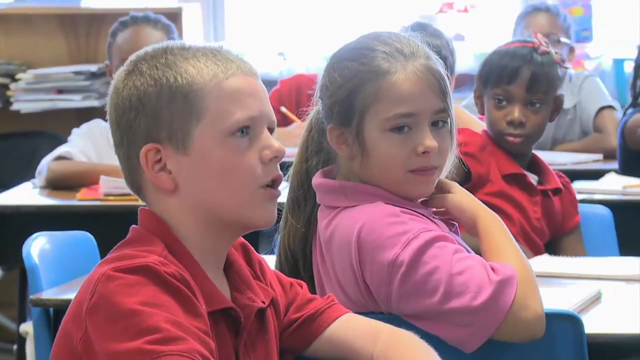 And prove it with evidence. Just like when we infer in reading, we must prove it with evidence. Ethan, nice and loud, I believe that multiple multiplicative comparisons means when you compare the two factors in a multiplication equation. Ooh, say that again. 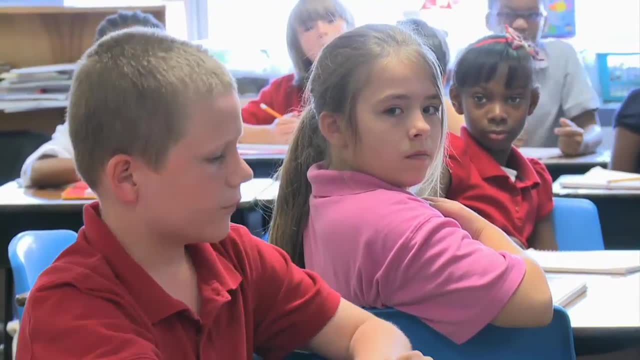 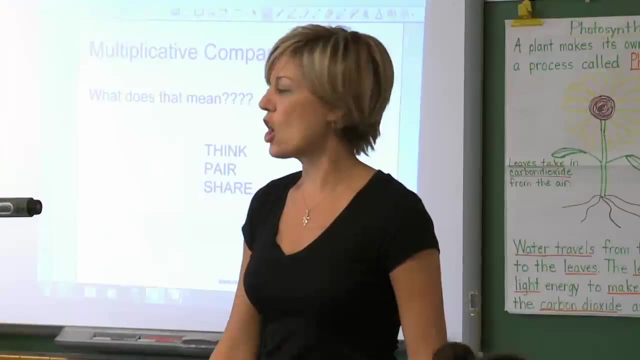 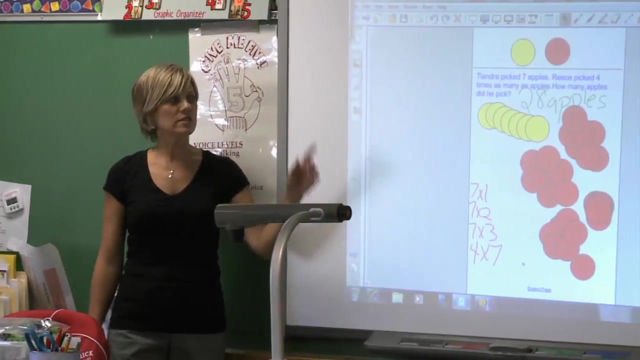 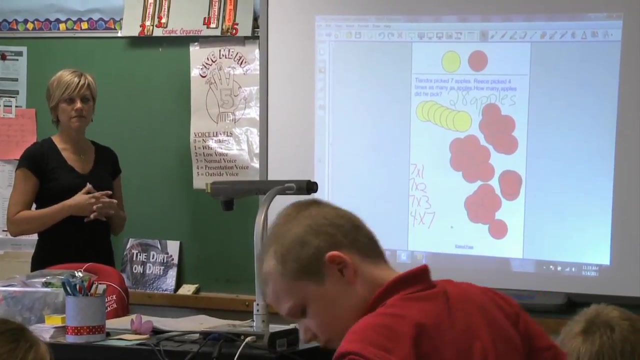 Nice and loud I think it is when you compare two factors of a multiplication equation. So I'm going to bring up this one And you talk to us about what you just said, Like what would be the factor? Come on up. 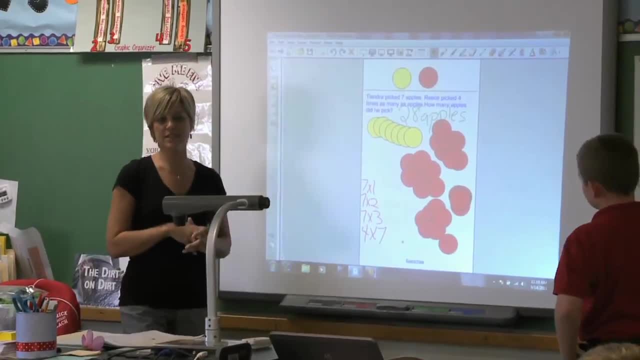 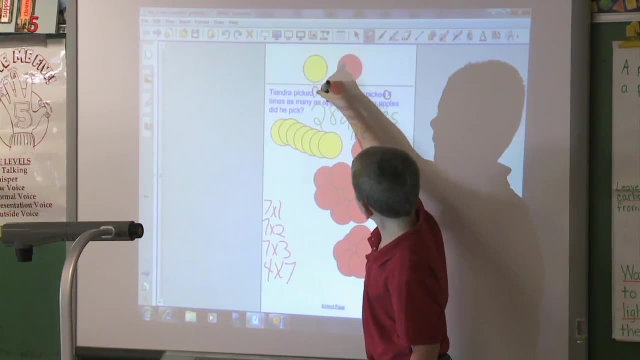 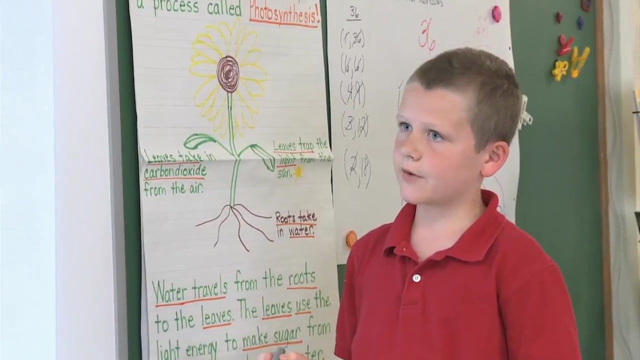 All rise. Miss Pratt's the student, Ethan's the teacher. Um, the factors would be four and seven. How do you know that? Um, I know that because um seven times four would equal twenty-eight. and Did our pictures show that? 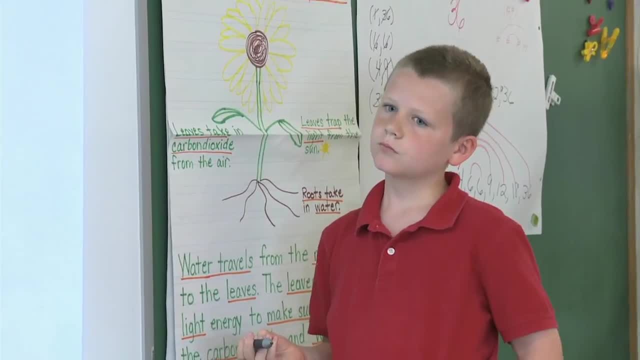 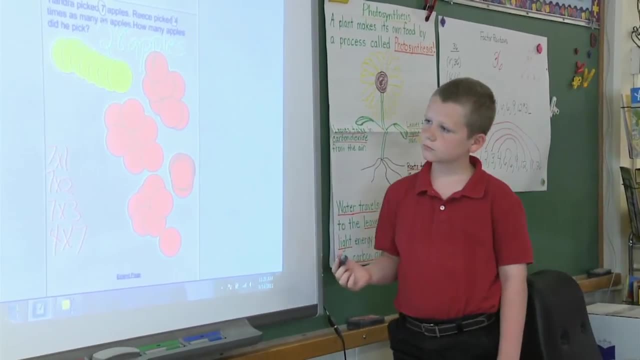 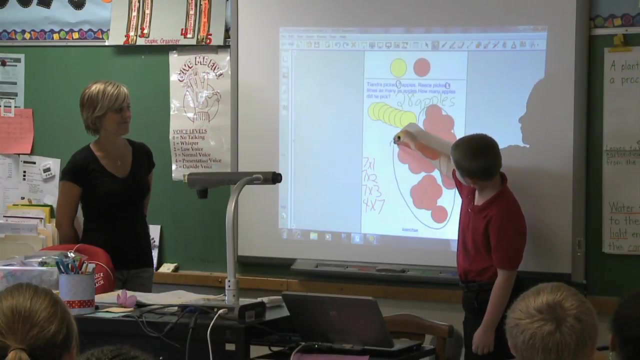 Um, Did our pictures show seven times four or the commutative four times seven? Did it? Yeah, Can you circle that so people can see where it says Four groups of seven or seven groups of four, however you want to look at it. 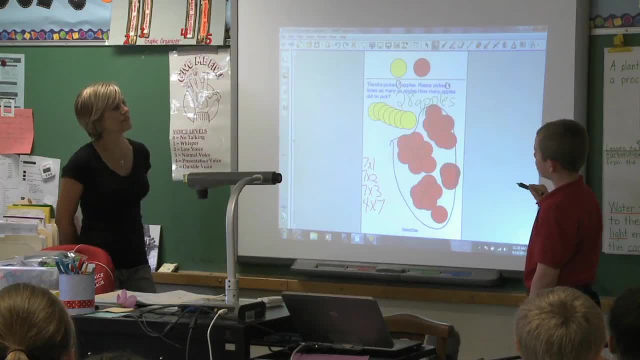 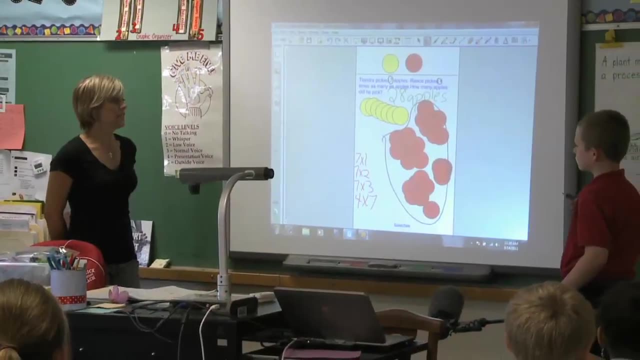 Good, Why don't you circle that one? Because that um is um, the is the number we multiply. Yeah, it is. And who's that about? Tiandra, Tiandra? And what is the rest of the story about? 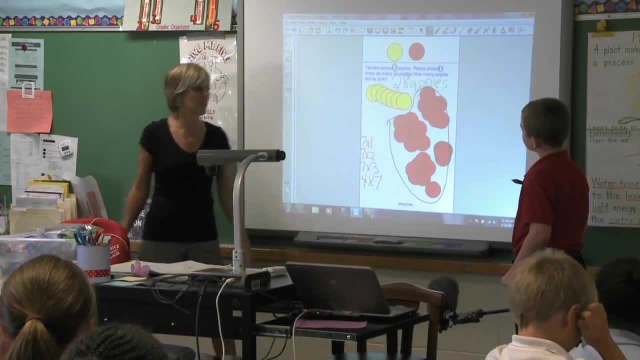 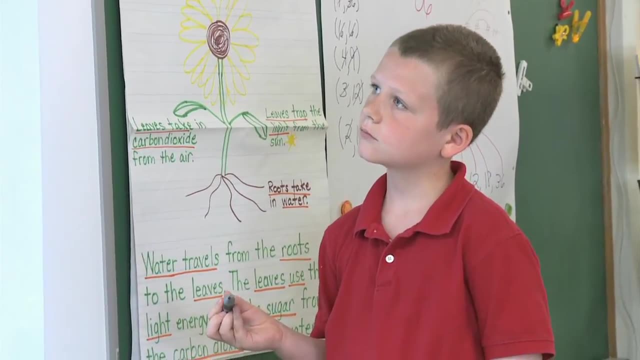 We've got to use this information. But what is the question? But what is the question focusing on? Um? it's focusing on how many apples Reese picked And which one. which one of these colors shows Reese? Um, wedding, Yeah. 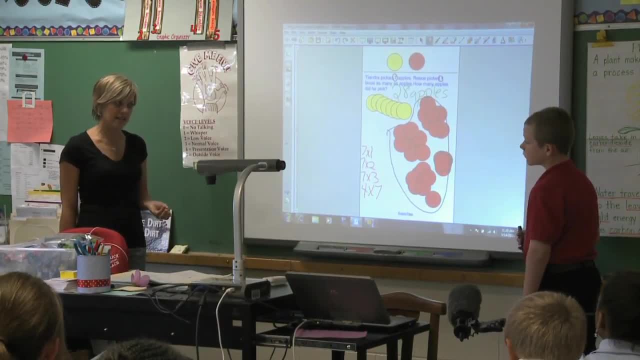 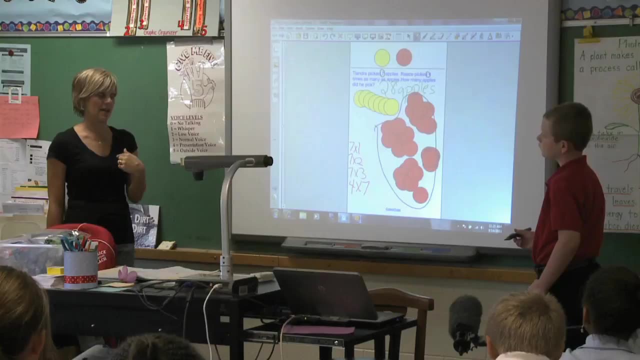 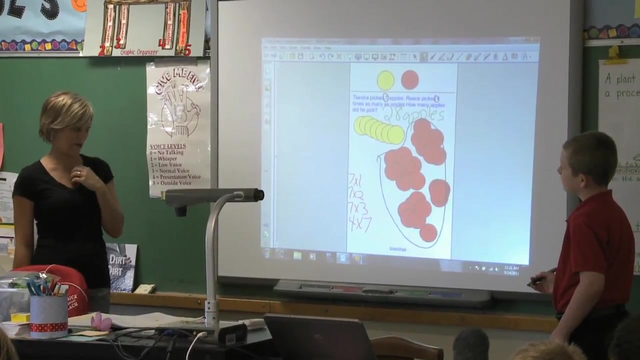 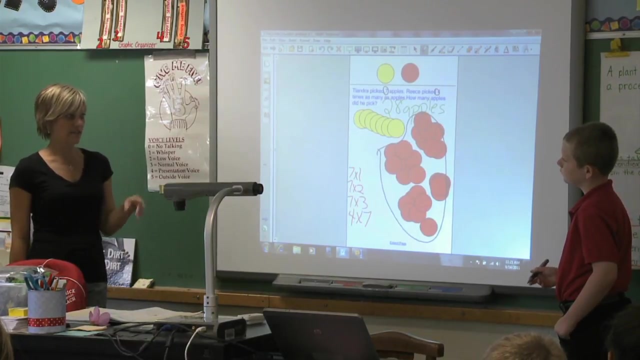 So he said, and let me restate it, and if I'm not saying it right, you help me, Because sometimes kids understand your language better than they understand my language, because they're used to hearing their peers speak. So you're. you're saying that multiplicative, multiplicative comparisons are when you're really comparing the two factors in a story to get a product. 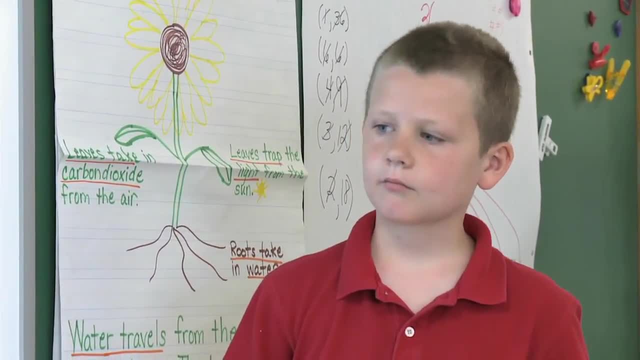 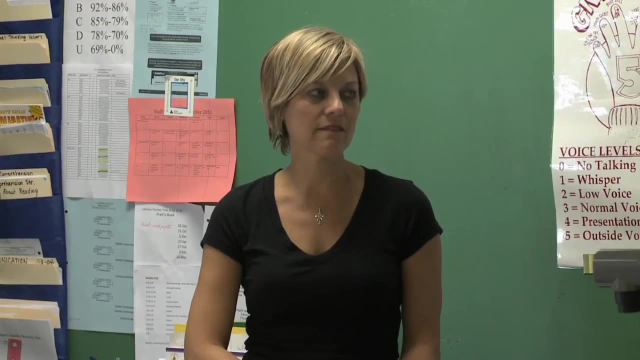 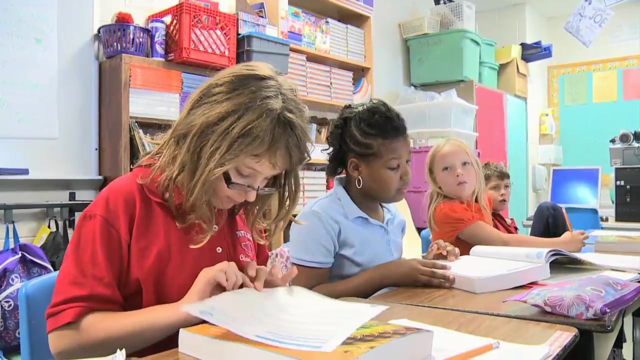 Yes, Go back to your seat, Good job. To sum it up, I want to look at the different ways we can say: four times 70 equals 28.. Yes, And we know the commutative property: Seven times four is 28.. 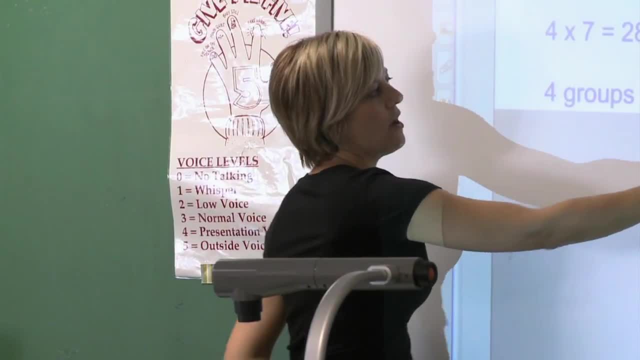 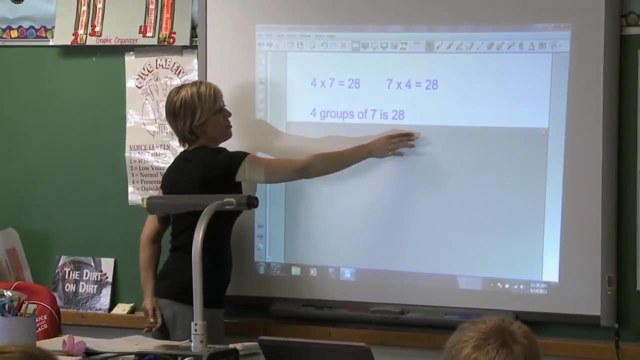 Let's look at the next one. I wonder if we can come up with it. We can say it this way: Let's say it: Four groups of seven is 28.. We could say it this way: Seven groups of four is 28.. 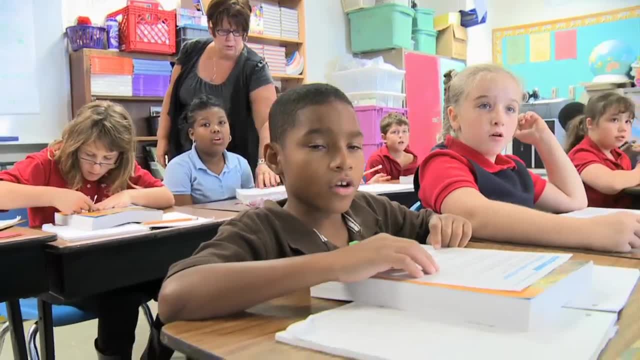 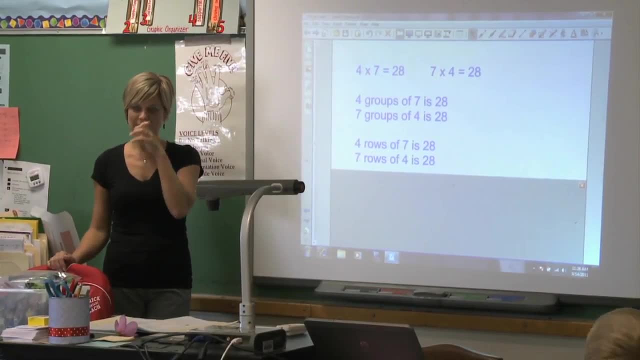 We could say it this way: Four groups of seven is 28.. We could say it this way: Seven groups of four is 28.. I'm going to show you this and I want you to read it carefully. There's another one after it. 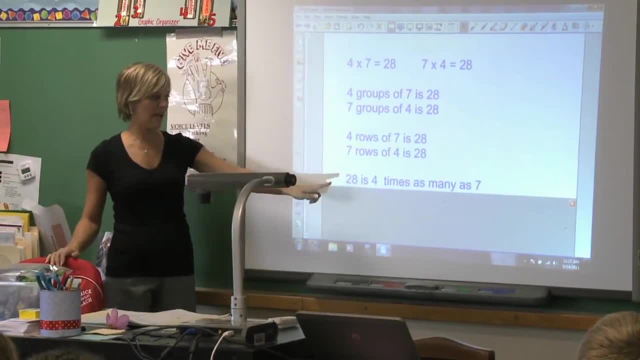 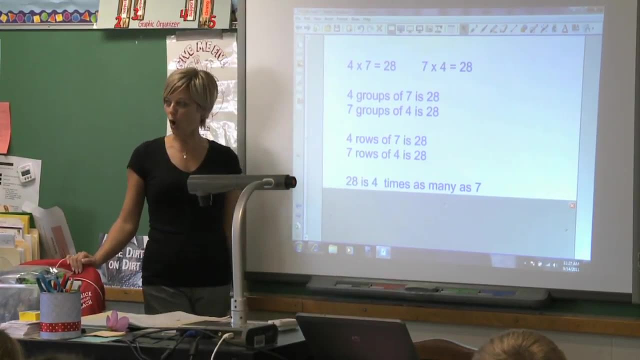 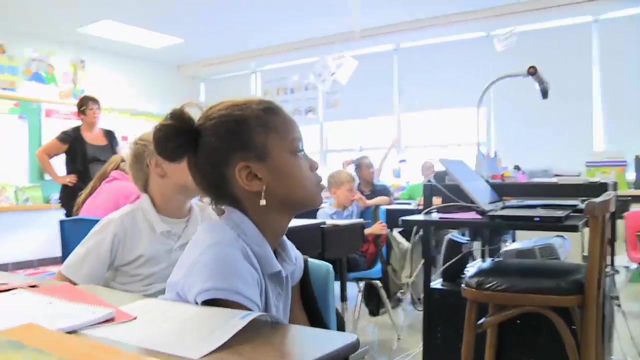 I'm going to show it. I'm going to see if you can guess what it is. We could say 28 is four times as many as seven Or 27.. Think it, think it. What could the other way be? 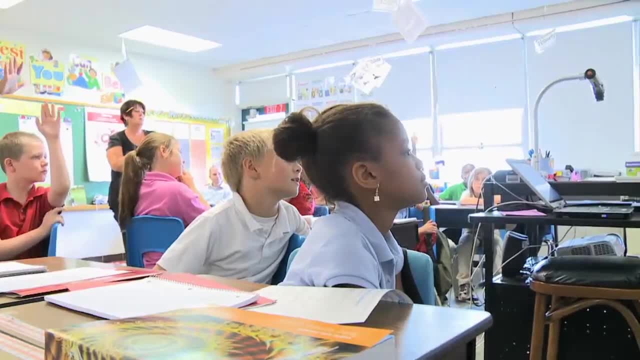 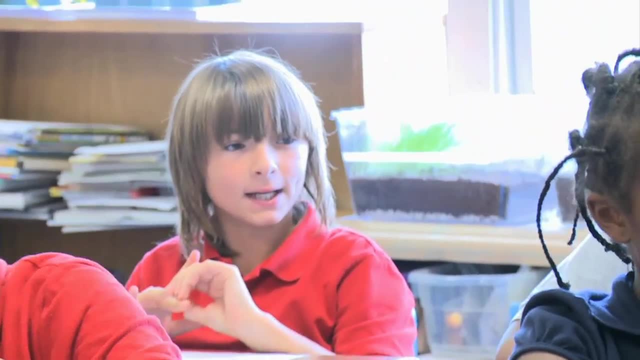 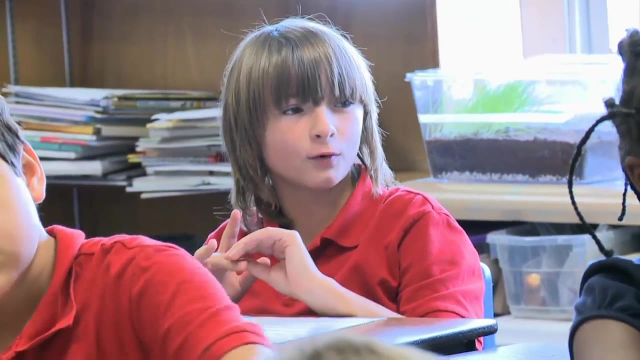 Seven, No, shouting out Trent. what are you thinking Loud? Seven, seven times as many. Seven is 28 times as many as four. Does that make sense? No, Is seven 28 times as big as four? No, 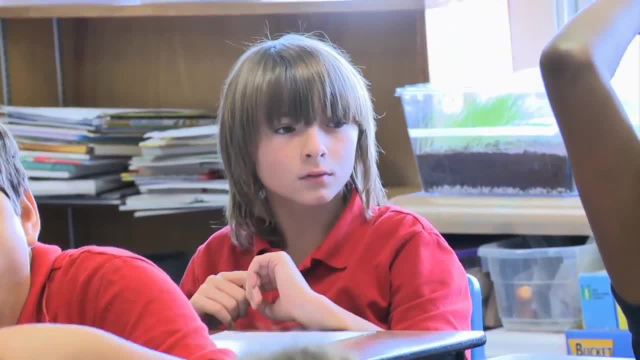 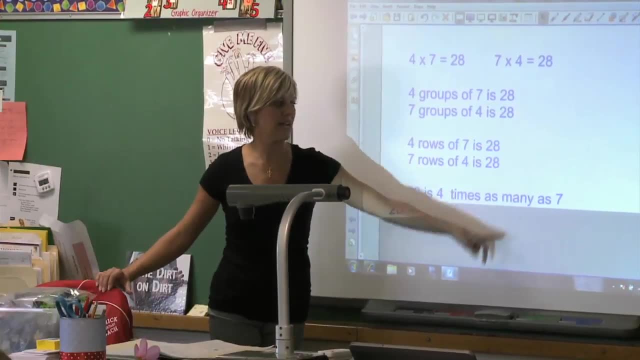 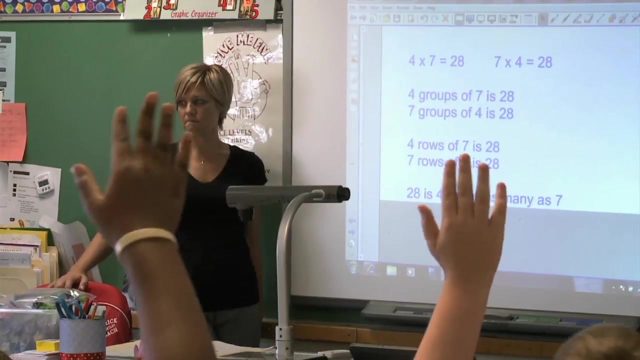 If you think about the pictures, that means we have 28 fours. Is 28 fours going to give us seven? No, Look at how it's written. 28 is four times as many as seven. There's a bunch of factors there. 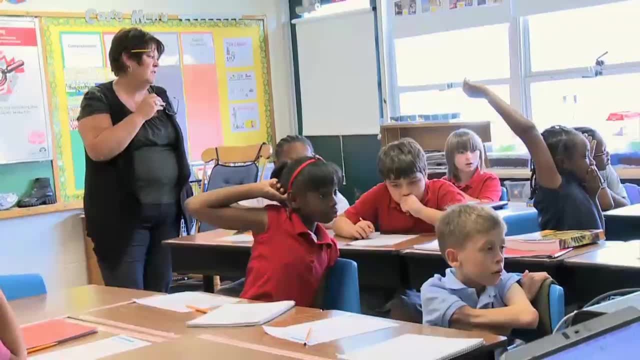 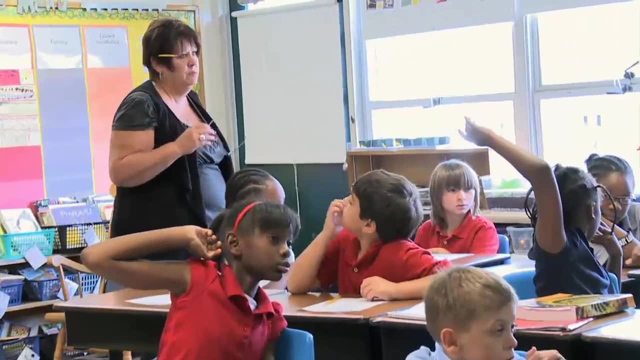 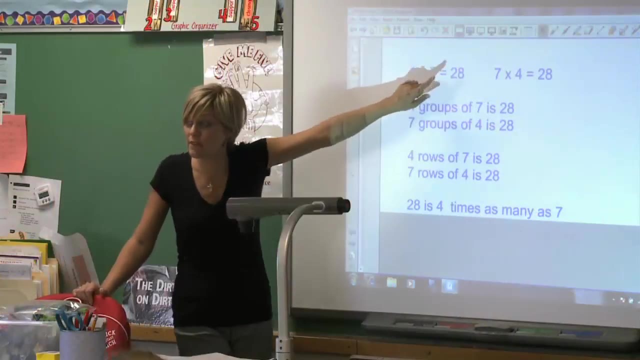 We switched out factors, so what are we going to switch out here? Seven and 28.. No, Is 28 a factor? Got to think of factors. Seven And Four? Yeah, Because four times seven is 28.. Four times seven is 28.. 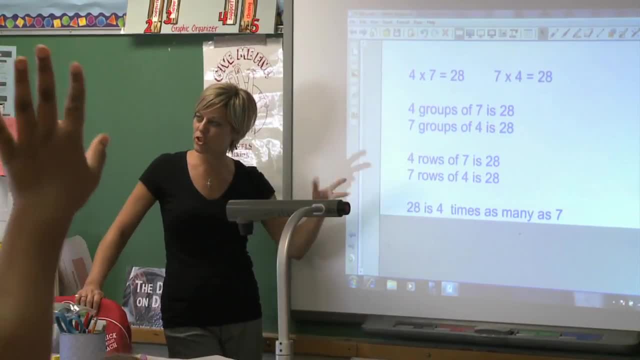 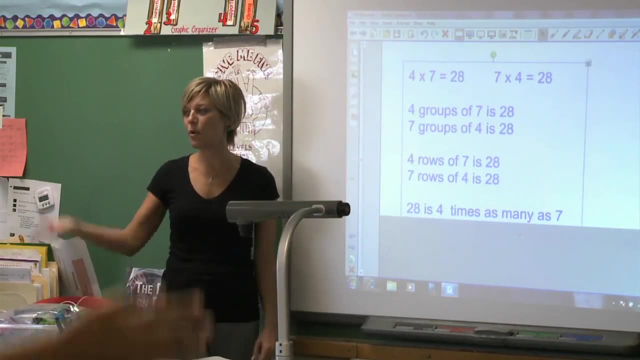 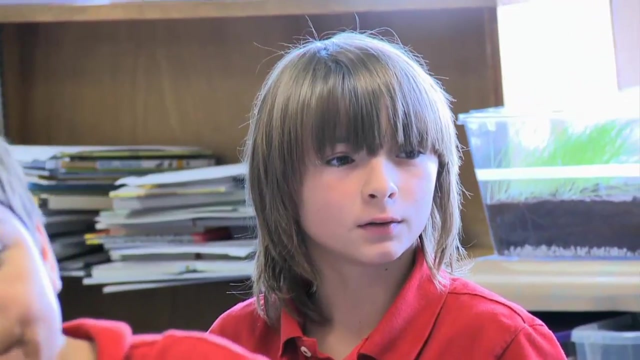 So we switched them out. We got to switch them out. here We're doing. the commutative We can say Is That's what that said. Change it. Change your factors Is seven times as many as four As many.